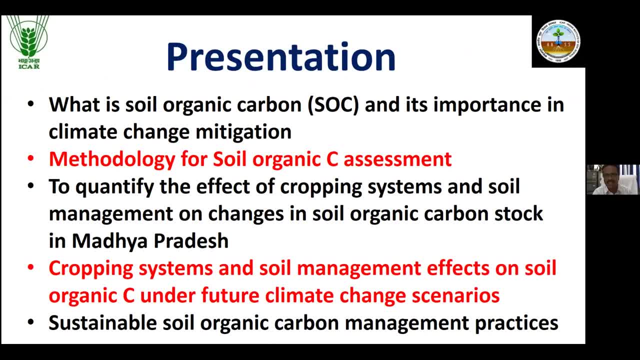 will be in this format. you will have a basic concept: what is soil organic carbon and what's importance in climate change mitigation, how it helps. then, what are those methodologies of soil carbon assessment, what methods you follow and what methods I have followed to give you this presentation or from output of the research, what we have been conducting or we are doing, and to quantify the effect. 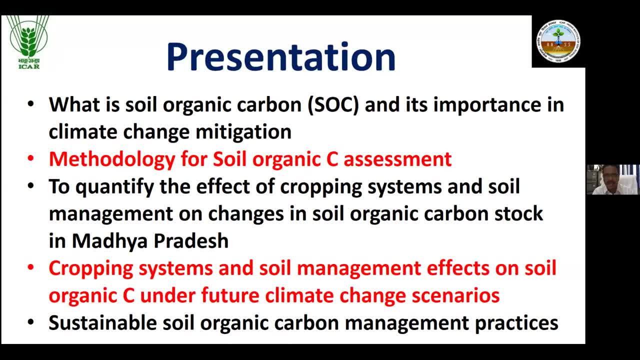 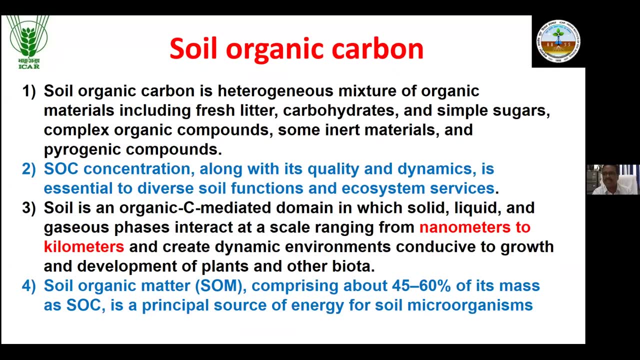 of cropping systems. that's what actually you will see and soil management practices on soil organic carbon and under future climate scenarios also, and what are those sustainable management practices that will improve soil organic carbon. So before you start, so it's a basic concept. actually, what is soil organic carbon is a soil. in organic carbon means carbon in organic form in soil. so what is? 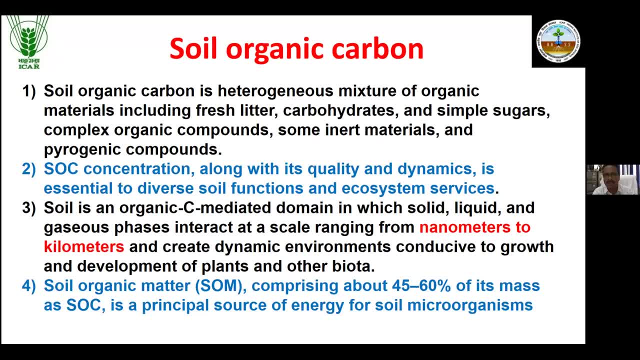 that actually it is the heterogeneous mixture of anything you add into the. you'll have a graphic. so it's for capturing the soil: organic carbon formed according to the soil conditions, then the component that is wound, the soil provided as the product, The process in which that is. 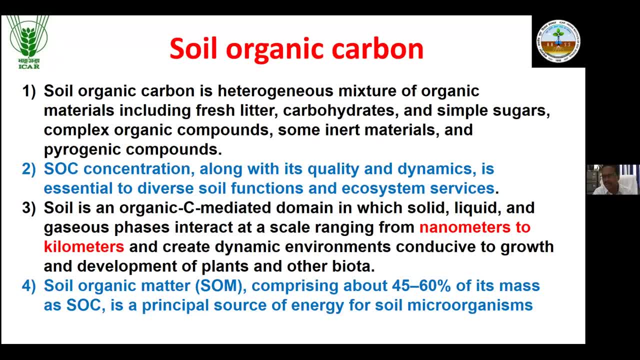 going to happen叫 roa. So we first a chili. like Jabahari isğimiz, this foundry for soil, organic carbon. it is all looking about the initial basis and the whole process of the many factors that we have in place over the years. It also the pivot moment which has been, we have been given. 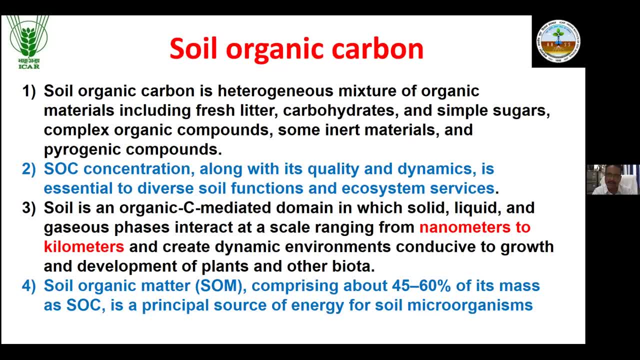 you might be knowing a little bit of knowledge or understanding about soil fertility. if your soil is fertile, if it is a good crop field and if the soil is healthy, then it gives many ecosystem services and even your drinking water will be that you know pure 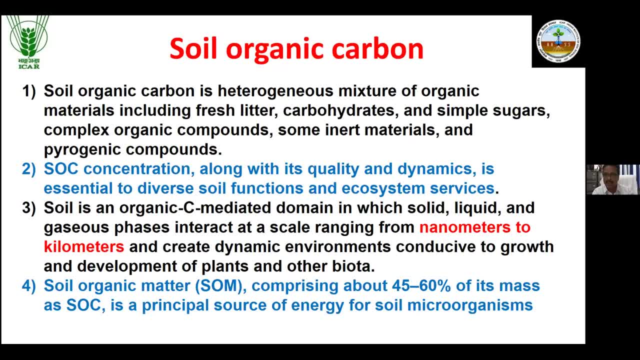 So diverse functions in the soil. you know carbon is a source of energy for the microbes and without microbes you cannot think of anything in this world. So they are everything you know. because of microbes we are here. Otherwise, you know, all those processes that's happening inside the soil is governed by the microbes. 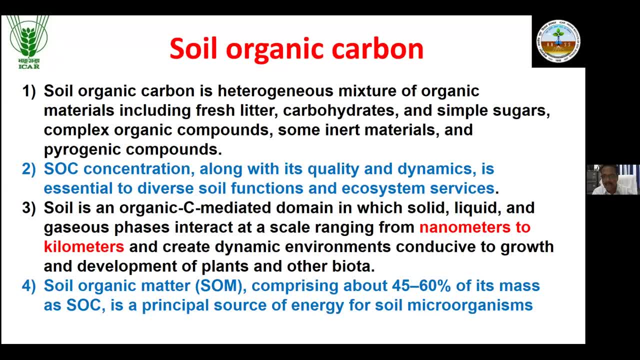 So because of presence of soil, organic matter or organic carbon, because of source of energy for them, they do. you know different nutrient cyclings. you know For plants we need nitro, all essential elements like nitrogen, phosphorus, sulfur, calcium, magnesium. 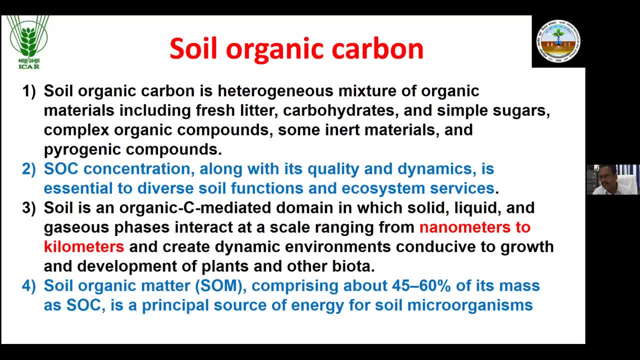 These are all essential micronutrients, like copper, iron, manganese, zinc. You know these are all essential nutrients for plant growth and, because of presence of carbon, because of microbes, We have many essential nutrient cyclings that is happening inside soil. 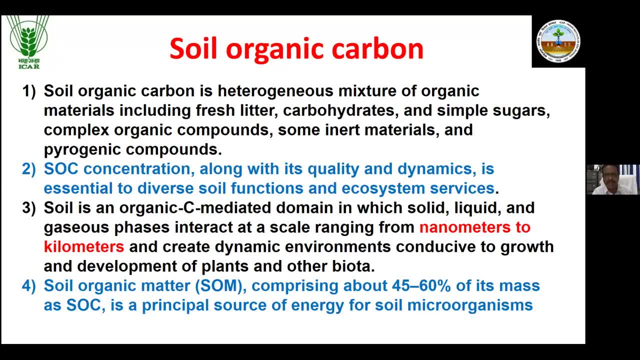 And it's interesting to know that soil is an organic carbon mediated domain in which solid, liquid and gaseous phase interact in a scale ranging from nanometers to kilometers and create dynamic environment conducive to growth and development. that I little bit I mentioned, and other biota. 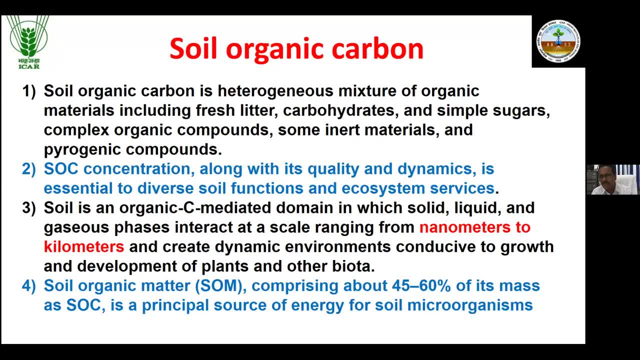 So all biological activity that is happening inside the soil, the presence of carbon, And that's why we call soil is a liquid, We call soil is a living matter or living entity. It's not dead, It's not dirt Soil is. you know, one spoon of soil have millions of microbes present in it. 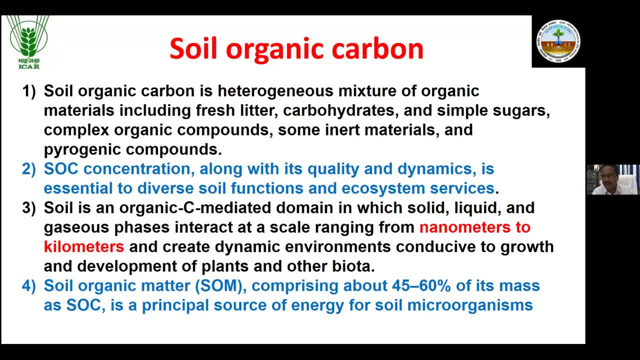 And soil organic matter, which is comprising, you know, about 50 to 45 to 60 percent mass of soil. organic carbon is the principal source of energy for soil microbes that I only mentioned. So this is the basic concept about soil organic carbon. 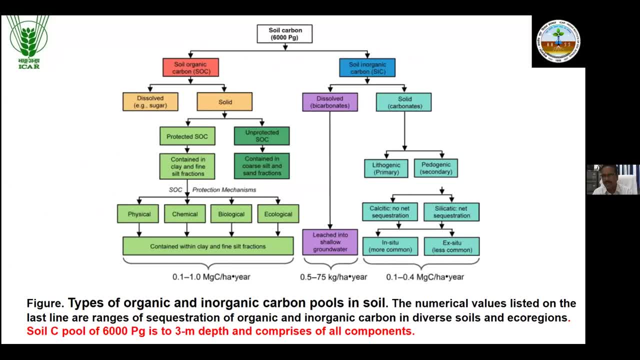 And if I give you this chart and I'll tell you that, what is soil organic carbon? I'm talking about soil organic carbon, Soil carbon. it can be two parts. You can see I was talking about this part, soil organic carbon. given, an important part is all soil organic carbon. 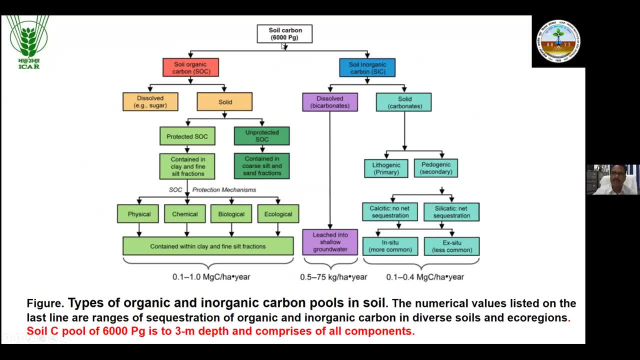 So total is soil carbon And soil carbon. if you see only three meters soil depth, you'll have 6,000 petagram of carbon in this world. So if I break into two parts, one is soil organic carbon, which is very much important for agriculture. 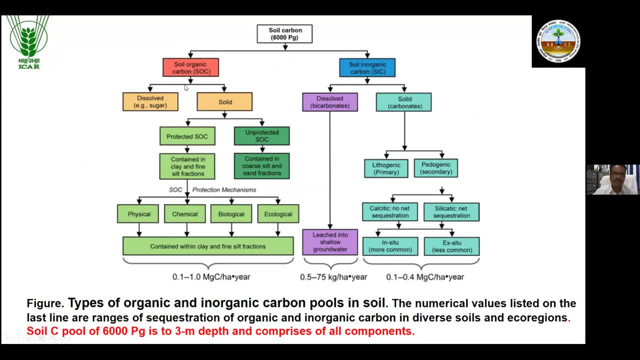 And we are more concerned about this than that. So when it is soil organic carbon, there are two types, As I mentioned earlier. one is soil organic carbon or soluble sugar or soluble carbohydrates that's in soil solution, And one is in solid phase. 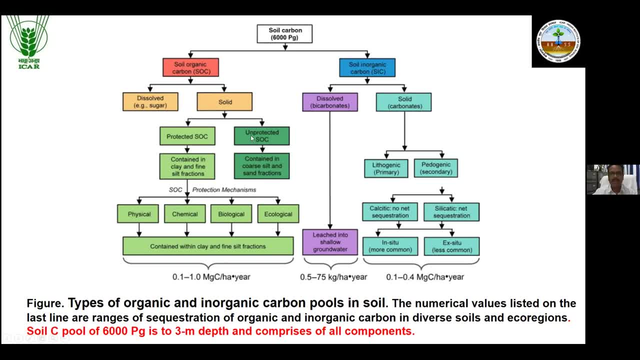 In solid phase this carbon can be protected unprotected. So you must be knowing that soil is part of, you know, sand, silt and clay fraction, So protection is given by this clay and fine silt fractions. And unprotected parts means that is subjected to decomposition by microbes very easily. 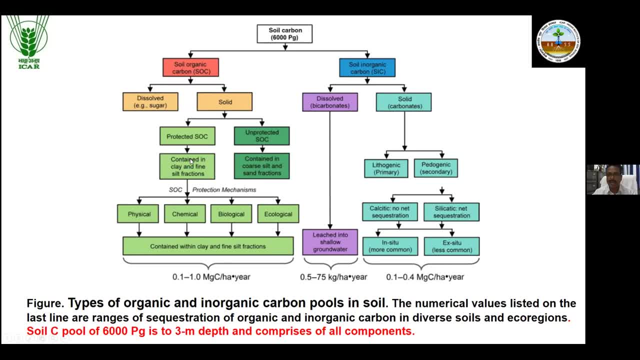 Protected means microbial becomes active And the activity of microbes on this part, because you know that it's source of energy, they will act on it. So we want to give protect to the soil. organic carbon- That means your soil is clay and fine texture. soil or silt content is high. 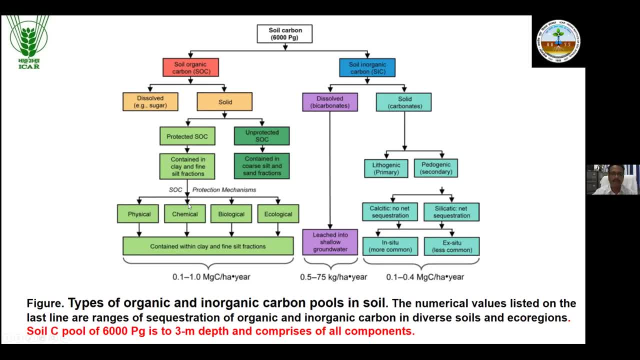 There's every chance that you can protect your soil, organic carbon by these means- physical, chemical, biological, ecological means- And that means the clay and fraction will help you protecting the organic carbon. If it's unprotected, it means it contains the core, silt and silt. 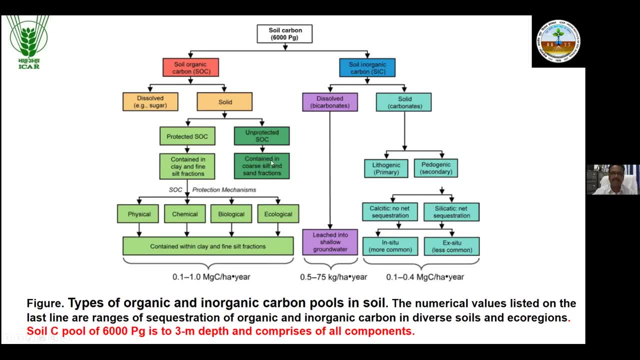 And if it's unprotected, it means it contains the organic carbon. So this is very much subjected to decomposition. But when you talk about the inorganic part, there can be two parts. One is dissolved bicarbonates, Another is solid carbonates. 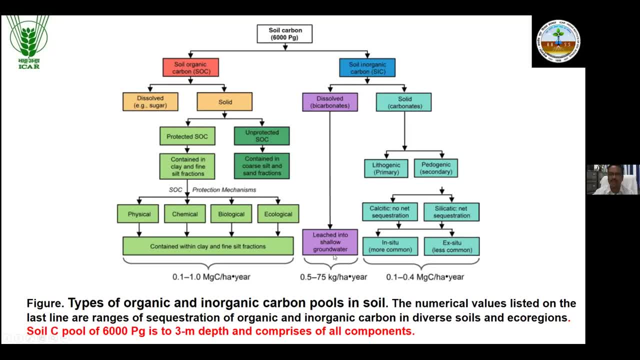 Dissolved carbonates that will be in the soil solution leads to the groundwater with rain But or maybe irrigation water. But if there is light texture soil, Then if it is a solid carbonate then it may be lithogenic or petrogenic, primary or secondary. 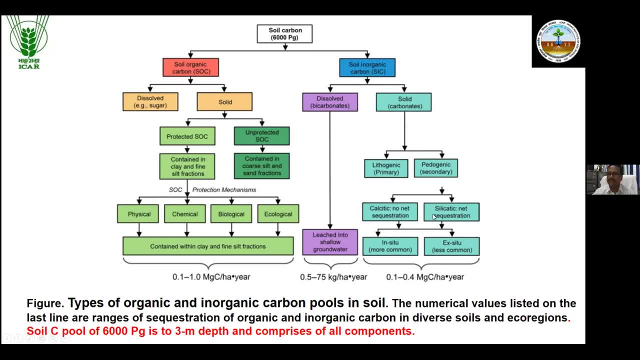 But secondary is important for us. It will give all those calcium, Calcium carbonate, bicarbonate, sodium, magnesium. So these are all present in the soil. They're a part of the inorganic soil carbonate, So my topic will be on this part. 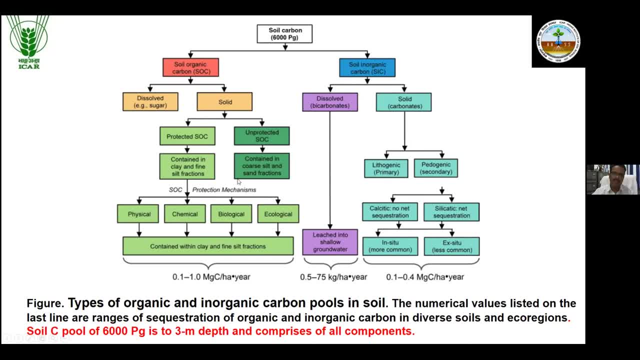 Where we'll be talking about how soil carbon is helpful to us And how we can improve through different management practices And what are the techniques I have used to map the whole soil of Madhya Pradesh, Having different- you know- nutrient management practices. 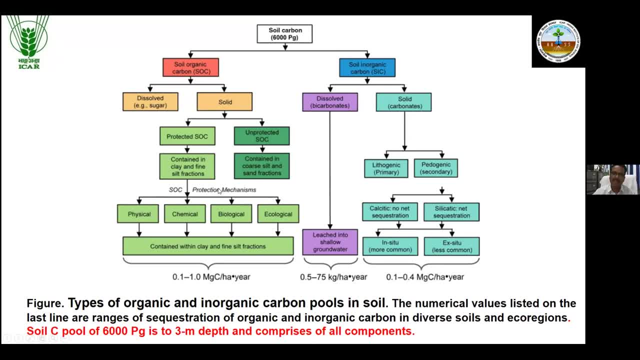 Because, exactly because you all are engineers, But definitely, when you sow a crop, you give different types of management practices: Nutrients, We feed the plants so that we get a good crop yield. So that's what actually I'll be talking about. 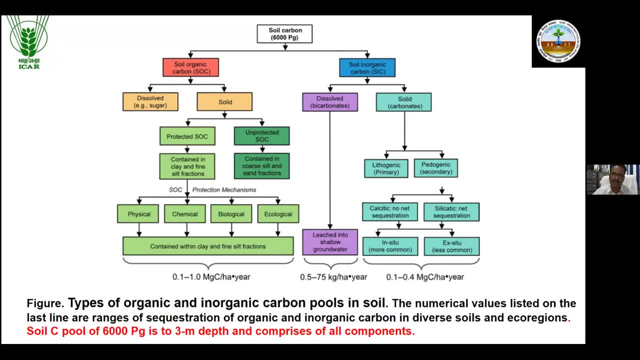 You know the many crops in and around Gopal also Soya bean, wheat, maize, chickpea- So we are talking about- I'll be talking about this- How this cropping system will also affect soil carbon in the system. So, moving to the next slide, 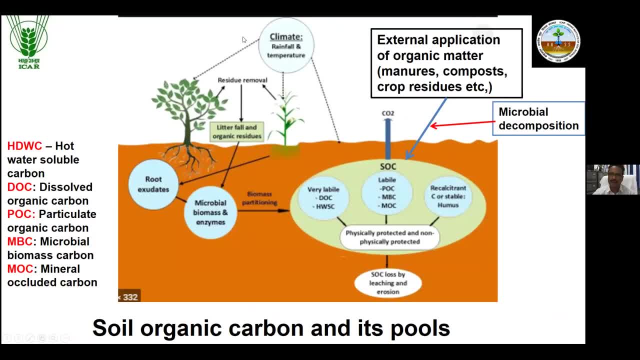 That's what actually. I'm going to give you the picture of The graphical representation of soil organization. So soil organic carbon. You can see where you get the soil organic carbon. So first have a look at this through the climate. But the rainfall, temperature and carbon dioxide concentration in the atmosphere. 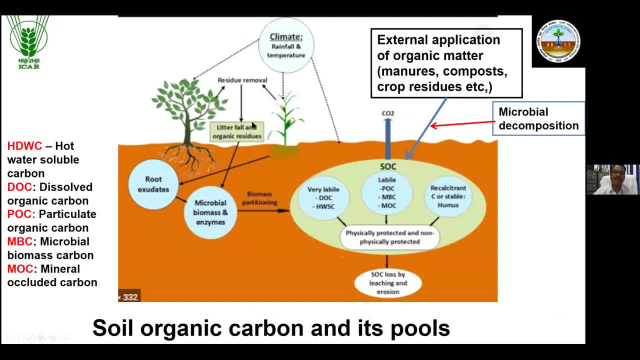 You'll find that plant grows And through the little fall and organic residues Or maybe root exudates coming out of the plants, That will subject it to microbial decompositions And a geometry activity And that gives you the soil organic carbon. 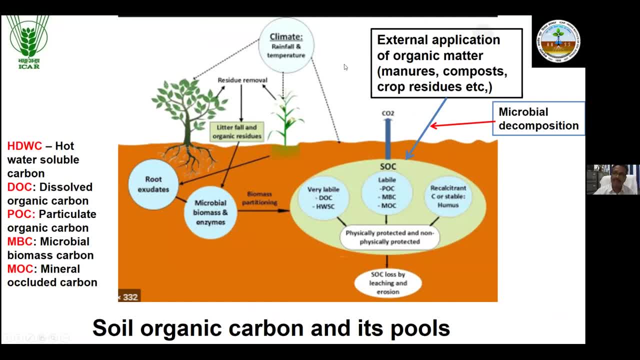 And even from the external sources of application of manures And compost or crop residues, Whatever you want- Through microbial decompositions. So it is part of the soil organic carbon And what you get Actually in soil organic carbon. We bring it to three different pools. 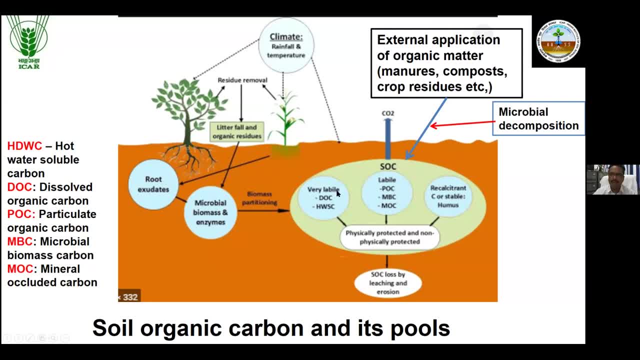 One is very labile, Which is easily available to the microbes. That means this is dissolved organic carbon. That's what I have mentioned here. Then one is SWSC- Hot water soluble. This is the method of extraction. That's why it is known as hot water soluble carbon. 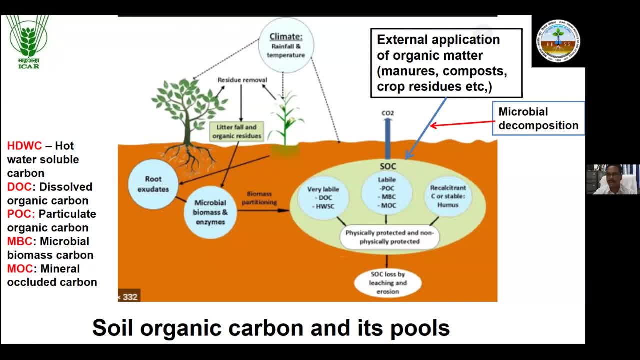 When you add soil to the hot water, Then you get water soluble carbon And you estimate what are the soluble components of carbon coming out of that And you estimate that That becomes the hot water soluble carbon. That's very labile, Easily available to the microbes. 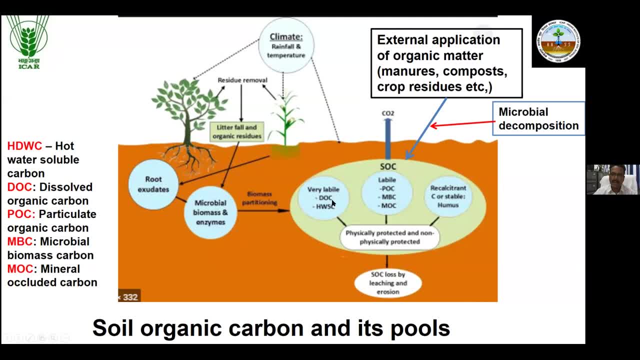 And it will decompose. You know, the simple Next is labile. It is particulate organic carbon, Microbial biomass, carbon Means, microbes, All those living organisms, Microbes just like bacteria, Fungi, Actinomyces, All those. 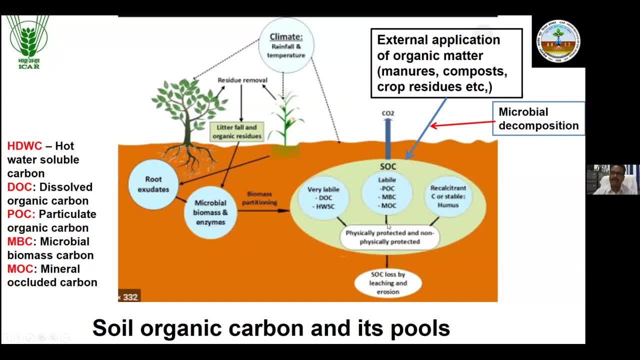 And mineral occluded carbon. These are also part of labile carbon And there are recalcitrant- Or maybe it's called humus, Which is the most important part of the soil, organic carbon. That means they are resistant to decomposition. 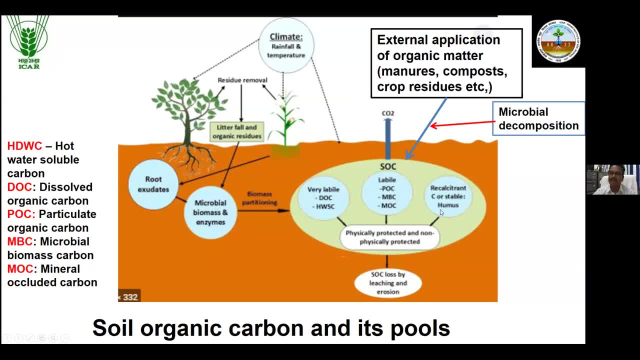 More this humus is there in your soil, Your carbon content. You know you are sequestering more carbon to the soil. So we always target those management practices Which can improve these two practices, Because their residence time And their stay in the soil. 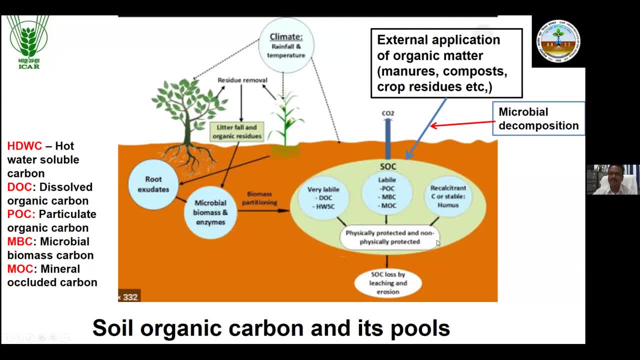 It's much more years. I'll come to that in the next slide. You'll find that. So these three practices, They are physically protected And non-physical protected. also That I have already mentioned in the previous slide How they are physically protected. 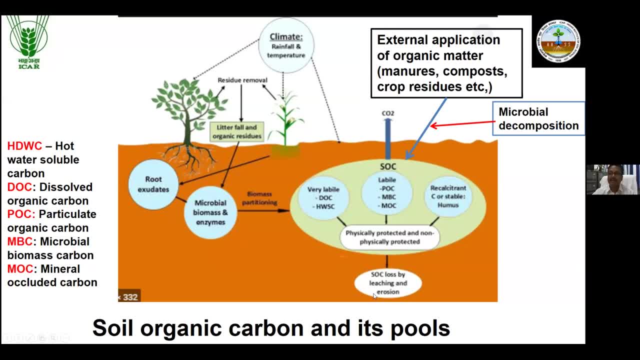 And they are also subjected to leaching loss, Or by erosion Through surface runoff, Or maybe leaching loss When they are soluble in water There are. The soil is light textured, Having more sand content That every chance that it will leach down to the profile. 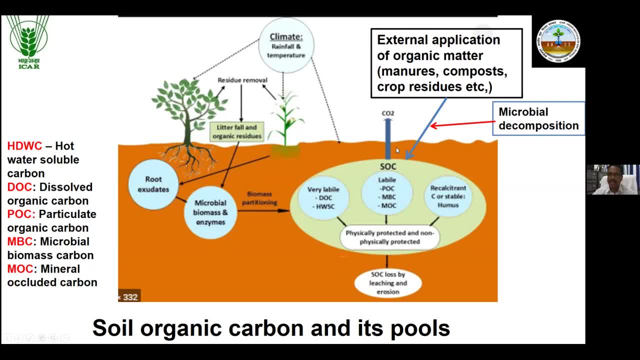 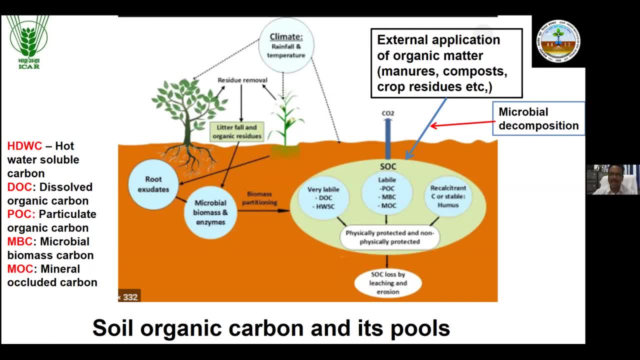 Is very, very soft And very, very soft. So There is one, A basic. I think You've got A good idea How, What is solar carbon And how They are present in the soil And what are those components in solar carbon. 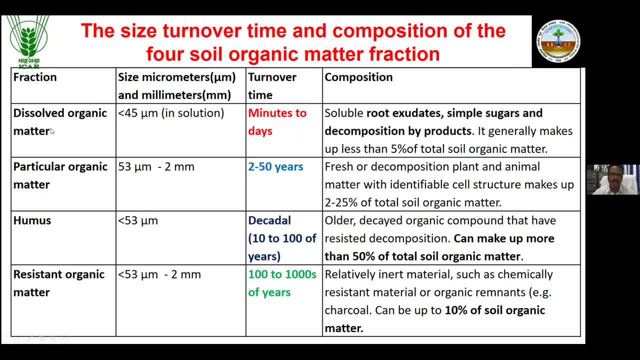 And which component We are targeting When you go for Our managing practices. So that's what actually? All those Components I mentioned In previous slides- You will see That that fraction Is digital organic matter Or digital carbon. 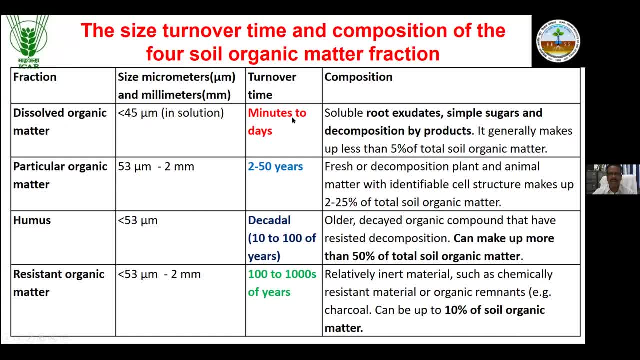 Then particulate organic matter, Then humus Diesel. organic carbon is very easily digestible and decomposed by. these are simple sugars decommissioned by products. So minutes to a few days they're in the soil, So they're very labile. 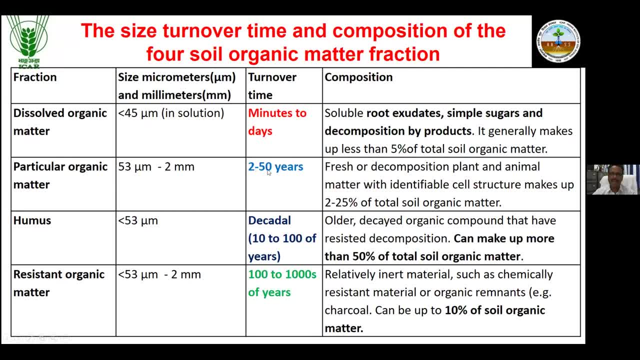 And next is the particular organic matter. Its time is two to 50 years depending upon the types of materials and quality of the material structure present in the material. And next is humus. where you target that tends to 100 years. So formation of humus takes that much time. 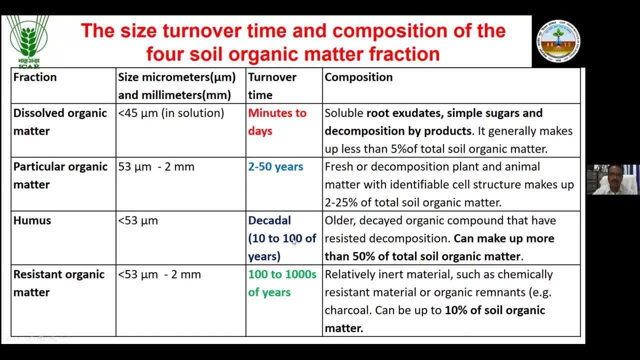 So the turnover time. that's also helpful for us to improve the soil organic carbon pools. This is one pool of the soil organic carbon. Then resistance: it is 100 years to 1,000 years- And their resistance with their inert material. 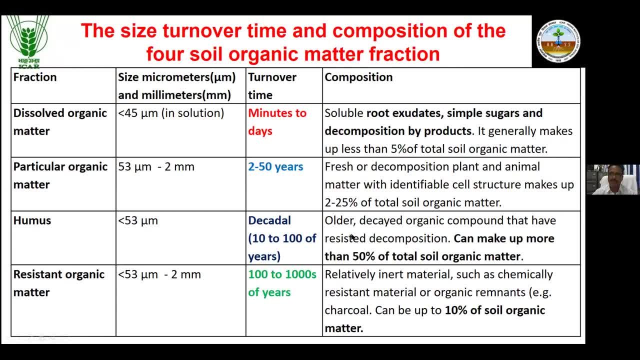 and microbes don't act on it. So by the time, so you are talking biochar, so you get many inert material because microbes don't act on those type of materials. So that's why adding biochar sometimes lead to improve your soil: organic carbon sequestration. 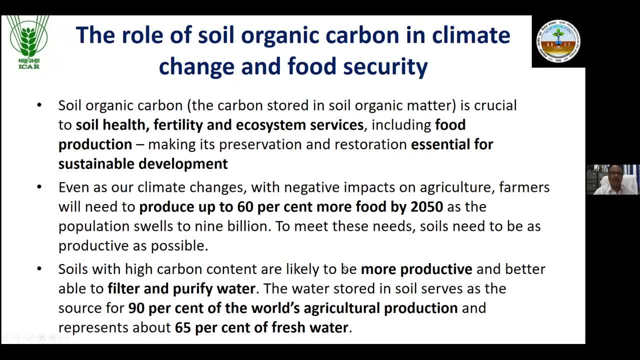 in the soil. Next is the role of soil organic carbon in climate change and food security. So when you talk about soil organic carbon, definitely you are talking about soil health and fertility and ecosystem services that I mentioned earlier and food production, So making it a preservation and restoration. 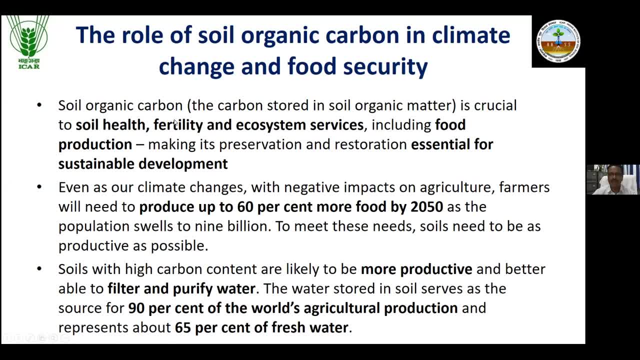 essential for suitable development, Because without soil carbon we cannot think of soil health and fertility. When you can't think of soil health and fertility, don't think of soil productivity. So we don't get good yield, unless otherwise your soil is good in carbon. 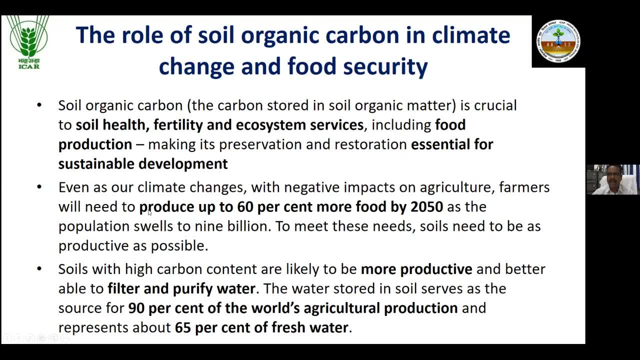 Even in climate change scenarios with negative impacts on agriculture, farmers need to produce. look at the 60% more food by 2050 because the population will swell to 9 billion. So we have to improve food production by 60%. That means to meet these needs. 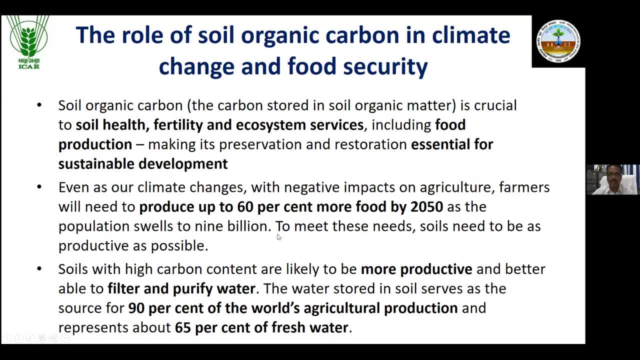 soil need to be as productive as possible. That's what actually most important thing is that: to make the soil more productive. we think about carbon, And carbon means that we need to make the soil more productive. Carbon means it's not inorganic. 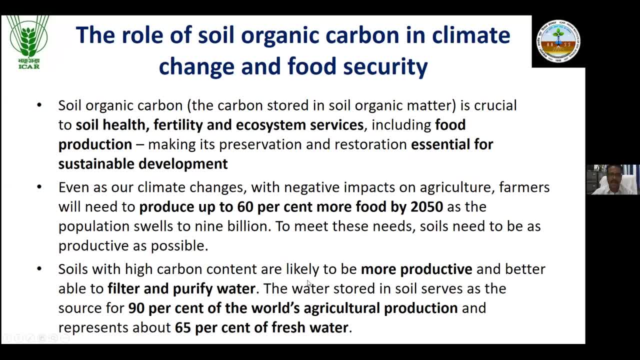 it's the organic carbon I'm talking about. So soils with high carbon content like to be more productive- that I mentioned- and better able to filter and purify water, And water stored in the soil serves as source of 90% of the world's agriculture production. 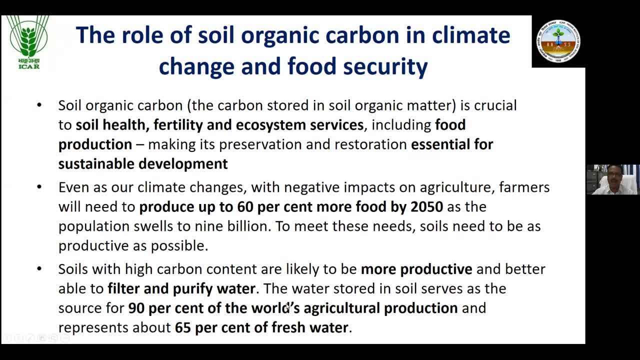 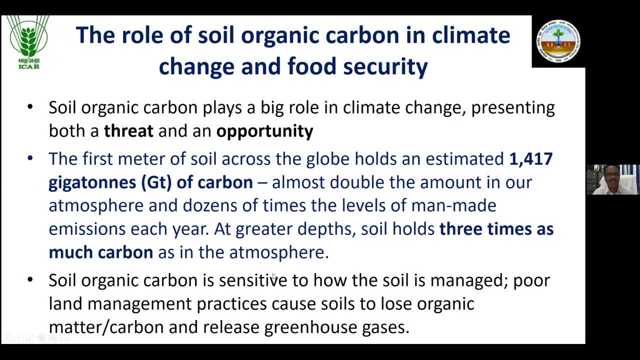 and refrigerant: 65% of wastewater. So how important carbon for security and climate change you can imagine in that way. And next is carbon plays bigger role in climate change. It plays a big, both threat and opportunity. because why did I say threat? 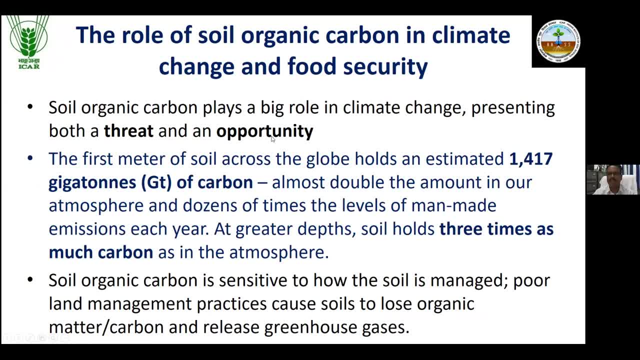 Because you know methane production and methane carbon is a source of methane production. When your soil is rich in carbon and there is stagnation of water on anaerobic condition fuels, that time there is formation of methane And that's why it is a threat. 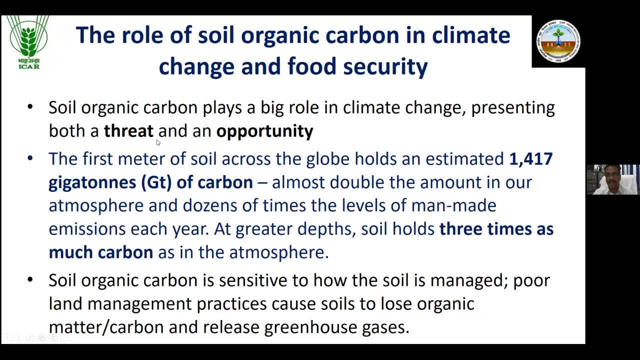 But we can reduce that threat to opportunity by suitable management practices, Because we know that rice soils, because you need some margins for those soils, and that's threat to you know, methane, that's a threat for us, But with suitable management practices. 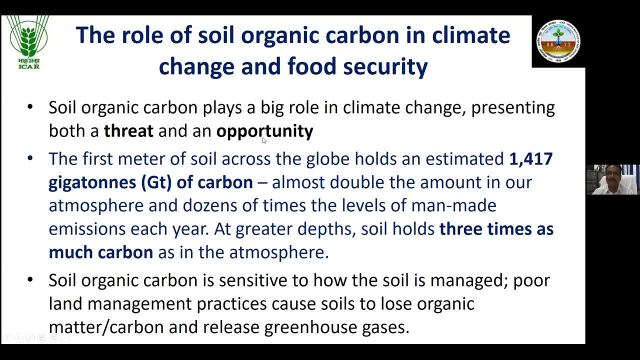 we can reduce the methane level. I'll give you example what type of management practices we can follow. If you are stagnating, then you are creating an environment that is anaerobic condition suitable for, you know, methane production. But what management practices? 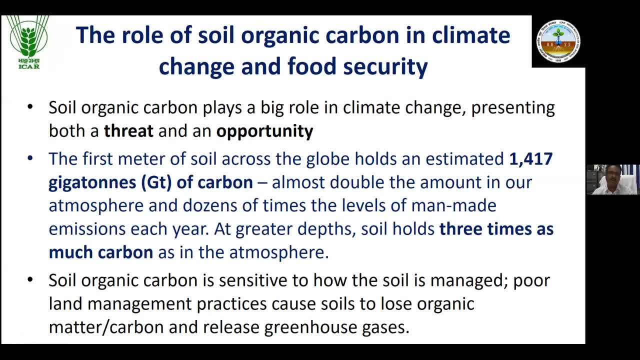 you go for aerobic rice cultivation or maybe direct seeded rice. You don't go for puddling, So in that case you are not creating that environment like stagnation of water And alternative wetting and drying condition also makes you know methane production less. 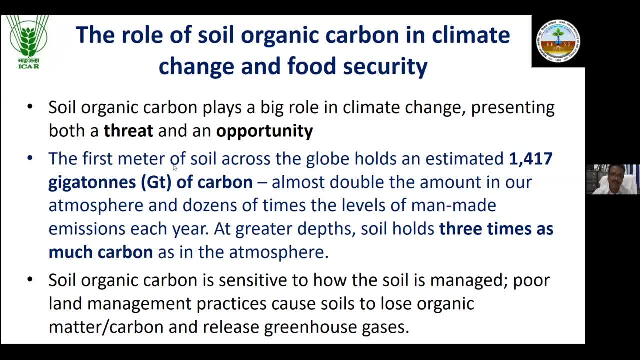 you know, it's lower than methane production. So the management practices, so that means the carbon trade- we can make this opportunity that we are utilizing carbon, And carbon is always beneficial, as I mentioned. So it's a threat as well as opportunity. 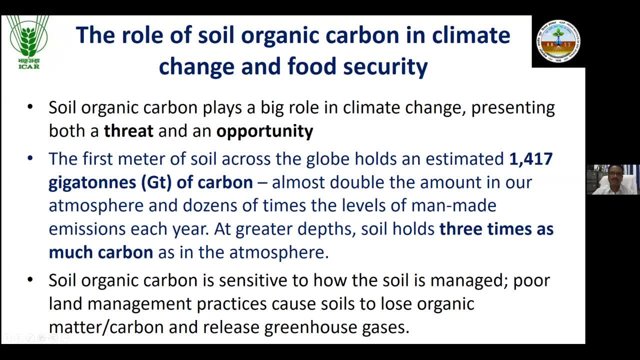 but we have to convert the threat to opportunity. So you know the first method of soil. I talked about six meters having 6,000 petagram of carbon, total carbon I was talking about. but you can see that you know. 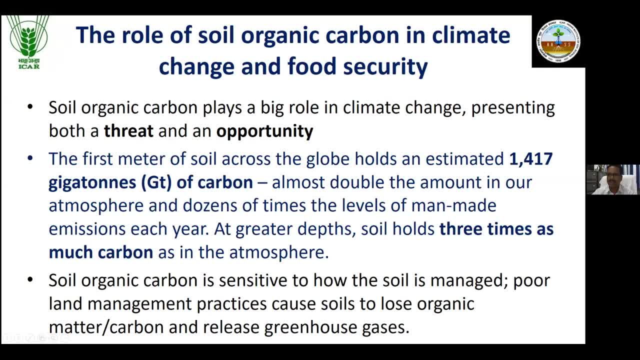 you can see that. you know. you can see that one meter bed also having 1,417 megatons of carbon, almost double the amount in your atmosphere, and that's times the level of man-made emissions each year. So how much important once you store the carbon in soils. 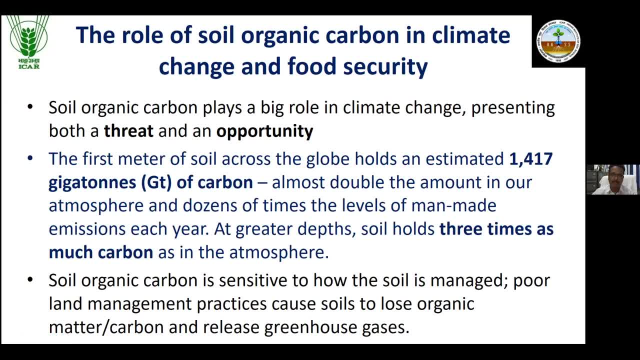 that means you are mitigating the impact of carbon climate change. So at greater depth, soil holds three times as much carbon as the atmosphere. So how much soil is important so far as sink for carbon? So soil carbon is sensitive. How soil is managed. 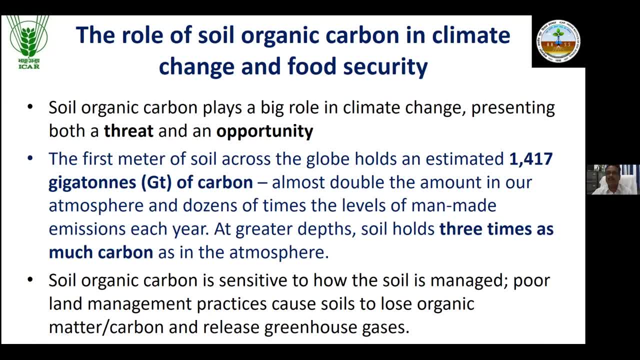 That's what actually your managing practices decides: whether you can hold more carbon in soil or not. So poor management practices just cause soil to lose organic matter and release greenhouse gases. So your managing practice is important and it will tell you whether your system is carbon sink. 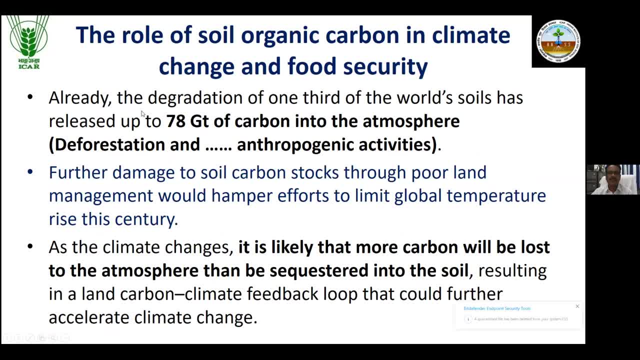 or carbon source. Similarly, if you degrade- you know already degraded lands, one third of soil is already degraded and released up to 70 gigatons of carbon. So that's important. So many things will happen to the atmosphere, So to the, you know. 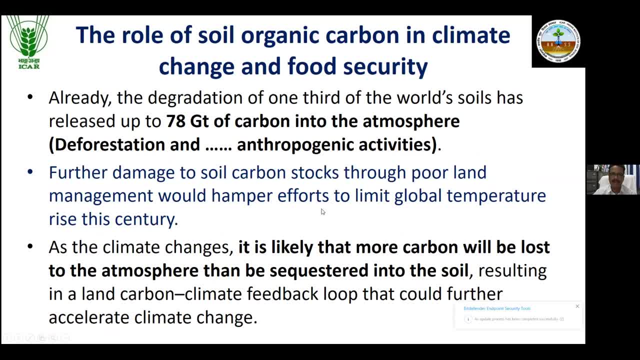 through the process of deforestation and anthropogenic activities and further damage to the soil carbon stock through poor landman practices would hamper the efforts of global temperature rise in this century. So it is likely that more carbon will be lost to the atmosphere than the sequester. 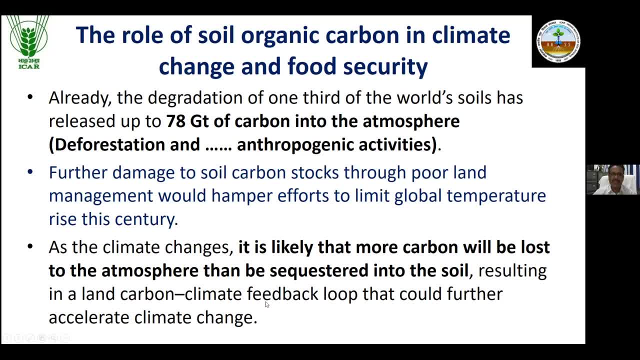 in process of climate change, resulting in land carbon, climate feedback loop that could further accelerate climate change. So soil, again carbon carbon or a total carbon, you can say. soil carbon is very much important and soil plays important control in storing the carbon, so it has a tremendous application in the soil organ carbon. 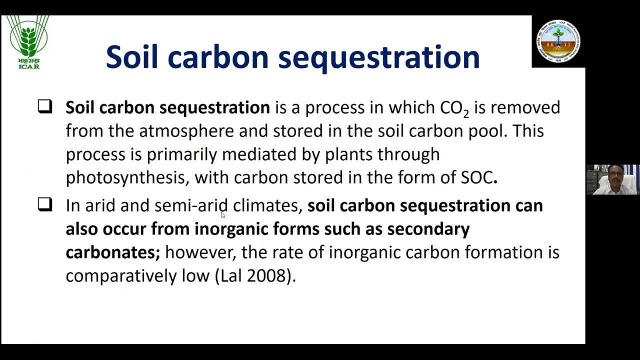 mitigating the climate change effect. so, uh, when we talk about soil and carbon tonight, we talk about soil carbon sequestrations. so what is sequestration? is what? what is this process? it is the process in which soil car, in which carbon dioxide is removed from the atmosphere. 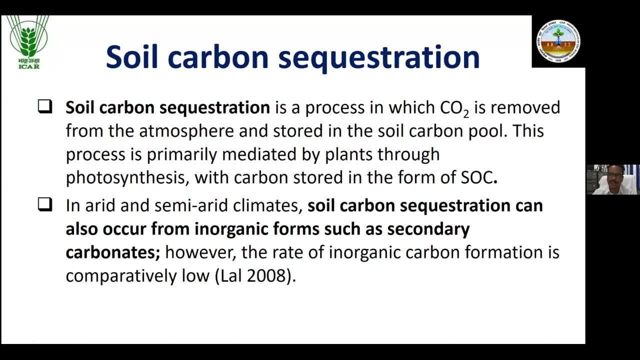 and stored in the soil, carbon pools, that pools- i was talking about that- at three different pools. so we want to bring those carbon dioxide through the process of- maybe you can say by growing plants photos to trap those carbons- and through that plants if you go to the soil and and this process. 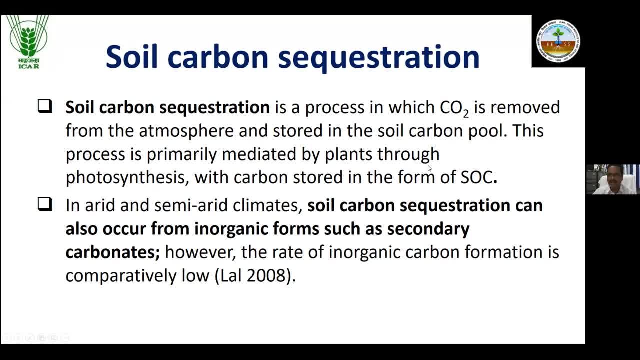 is primarily mediated by plants. definitely, plant is the biggest source of gas carbon capture and through photosynthesis, with carbon stored in the soil, carbon capture and through photosynthesis, the form of soil organic carbon. in editing and reducing soil carbon situation can be occurred to inorganic forms, as i mentioned in that flow diagram as secondary carbohydrates. however, the rate of 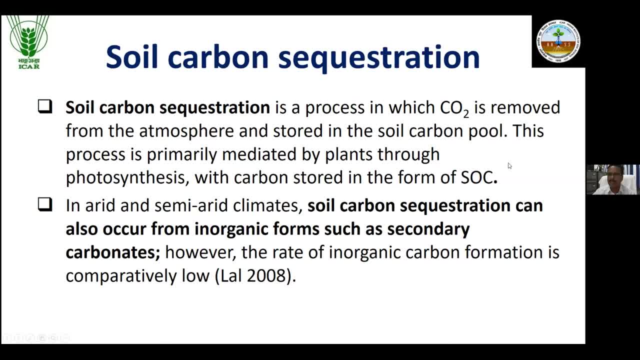 inorganic carbon formation is compared to low as compared to solid carbon. so the the process is that we have to improve the pools of carbon. that means less low mobile, mobile or labile, and more resistant fraction, which will be increased so that we can store more carbon in the soil. 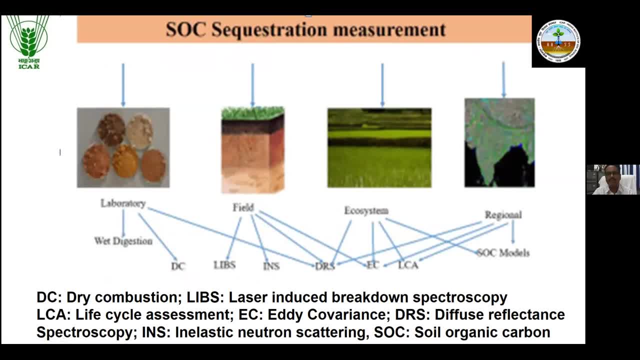 so if i'm talking about carbon situation, what are those measurements processes we follow, definitely when i talk about the soil in the laboratory conditions. so my presentation will be based on this also, some of the techniques i have followed in the laboratory. we have weight digestion technique. we call it potassium permanganate acid digestion. so with that, 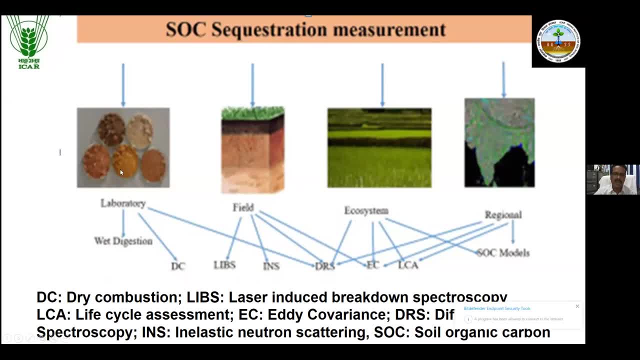 actually we try to find out what is organic carbon content of the soil and we can go for also dry combustion techniques. you can take the soil- analyzers are available like chn analyzer, or maybe just burning the soil. dry combustion, simple: burn the soil and see how much carbon loss there and through mass balance you can see how much carbon. 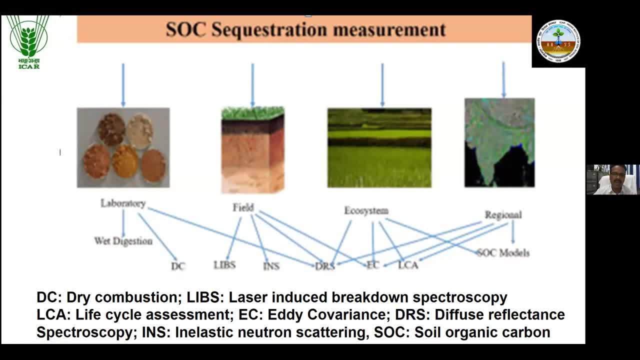 that is called dry combustion and there are different instruments like your total organic carbon or total carbon analyzer. you have chn analyzers, carbon hydrogen nitrogen, this- you know these instruments directly can. you can get the carbon content of the soil or you can go for drs. 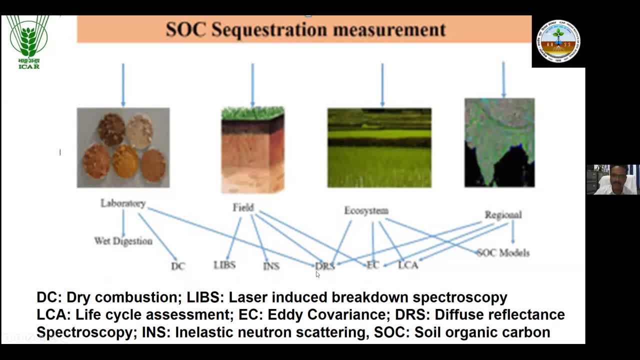 that is, diffuse reflectance spectroscopy. you are also working on this to estimate soil organic carbon in soils. that means near infrared and mid-infrared spectroscopy we can use and find out what is the carbon content in the soil. then there are others like leaves, laser induced breakdown. 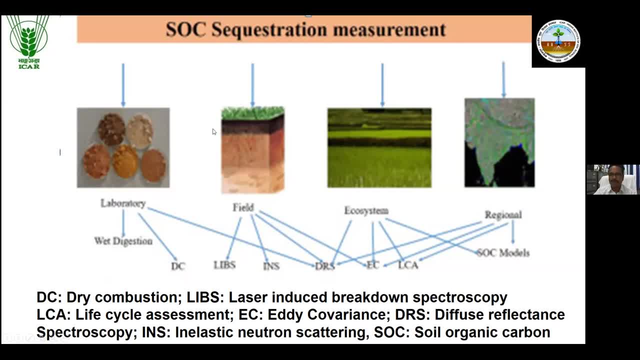 spectroscopy, and also when we cover talk about the field condition, we follow. these principles are these methods. but when you talk about ecosystem services, we go for two approaches. one is another, which life cycle assessment in agriculture, and when you go for regional scale measurement, that time we need modeling and soil organic carbon models or ecosystem models based on these. 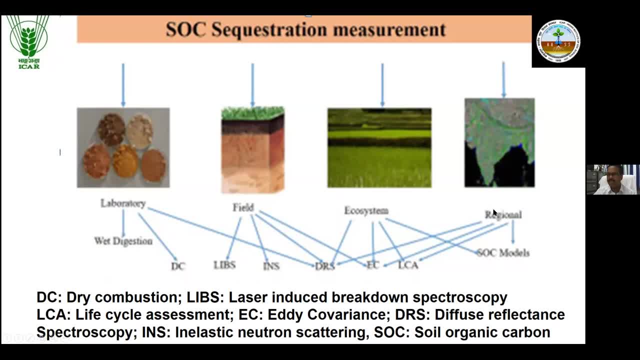 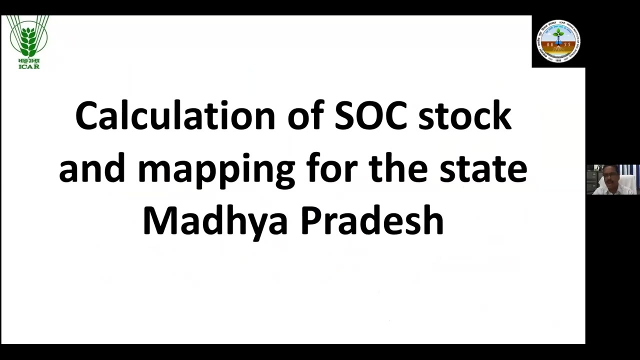 measurements and techniques. we- uh, we go for a special distribution of soil organic carbon through suitable techniques and in this case, modeling will help us on estimating the carbon balance, or carbon stock or carbon change on a large scale or regional scale or a country scale. so, based on this, i i want to show you how we have done for. 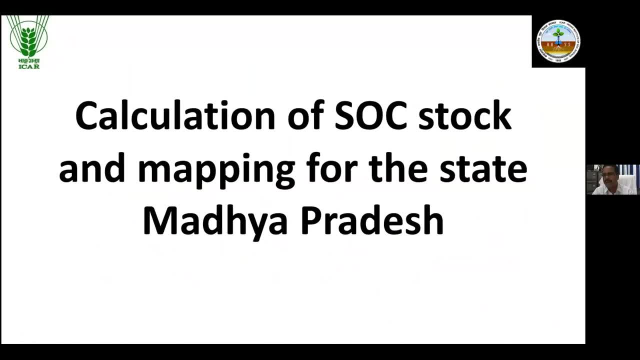 the state mother for this and what are those methods we have followed and what are those uh management practices, uh that leads to increase uh in soil organic carbon stock, and what is the stock of solid and carbon in the whole state? so in this case, you can see that this is soil map. 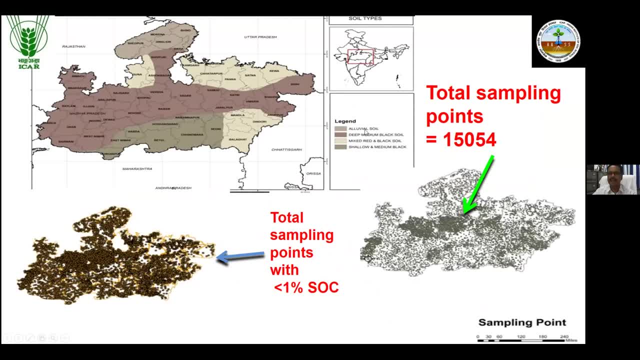 for the mother, but this will mostly find in different types of soils and alluvial soils: deep medium black cells, mixed red and black cells, shallow and medium black cells. you can see this is from mpcst map we have taken and based on that this is the sampling points. you can say we have collected 15 054 samples from the state and 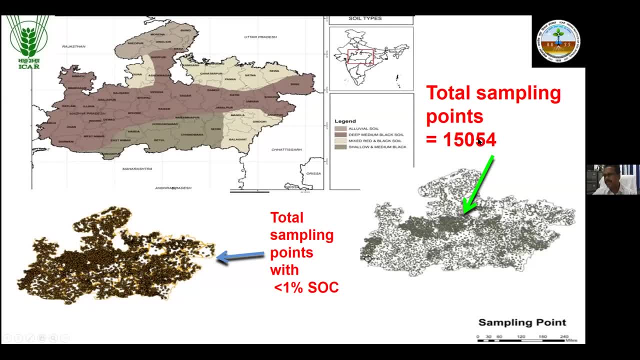 this sample collection was to our all-india coordinated research project on micronutrient, secondary nutrients and heavy metals, and from them we got those points. and since agricultural soils- because it covers almost all types of soils, starting from forest soils or all over- we come down to less than one percent carbon, because most of the soils are less than one. but 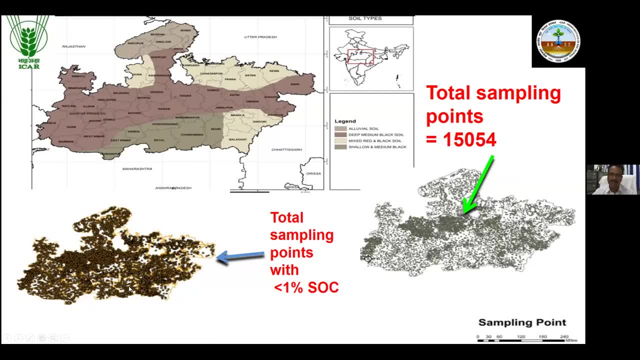 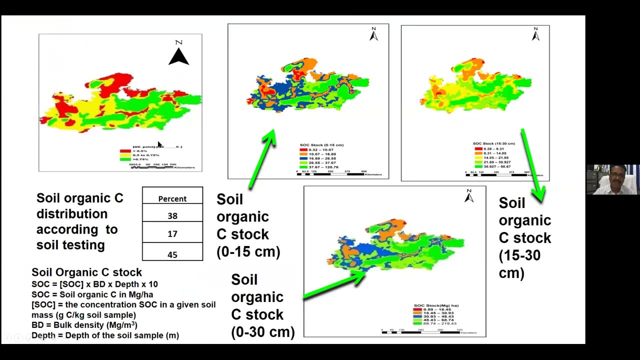 even i'll talk to you about that- how much carbon there in the month for this. but uh, you can see those sampling points from 15 000 to come down around 10 to 11 000 samples here and from those samples we analyzed to find out what is the carbon map for the spread based on the weight digestion. 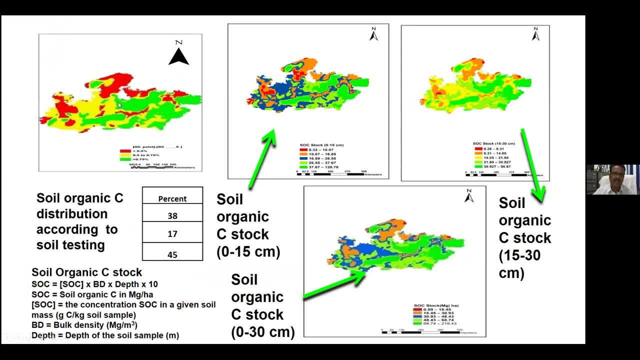 technique i was talking about. so from there you can find that the around 50 soils are coming to be low in soil organic carbon and medium around 70 percent high. high means because this category is 0.5 to 0.75 percent organic carbon. below 0.5 percent it is low, and 0.5 to 0.75 percent if the 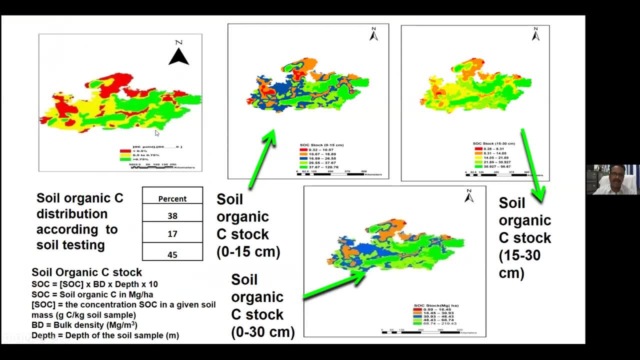 organic carbon content is there in the soil. it is medium and greater than 0.75 percent. it is high. so based on that, this is the map we have developed. then we developed. this is the surface. concentration means concentration of soil organic carbon in the top soil. 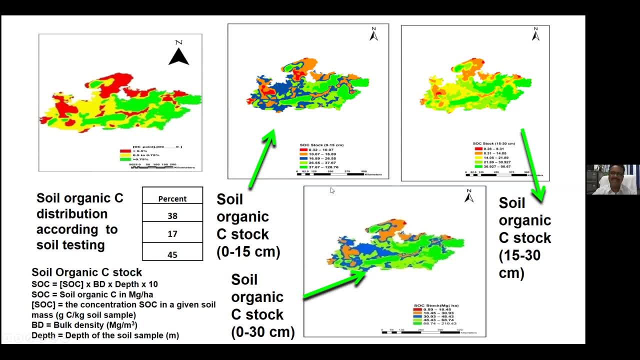 but when you talk about the soil, usually we think of 30 stops, 30 centimeters, because top 30 centimeters starts to be productive, because 75 percent of root growth they are in the top 70 percent of the soil, um surface soil. so that's why we went for again stock stock measurement. we 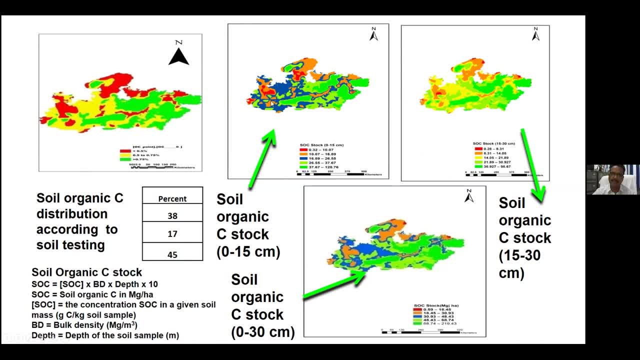 did it through this concentration multiplied by ball density of soil. politics it is: we follow a certain procedure to find out what is the ball density of soil, then depth, and we find out what is the stock. that stock in terms of tons for hectare, how much carbon there in the 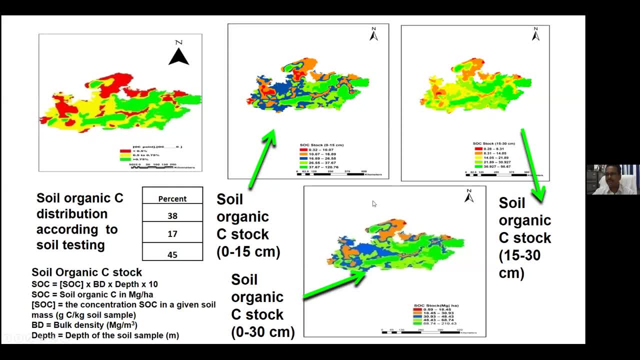 top 15 centimeter, then around the next layer 15 to 30. so and total stock about 0 to 30 top 30 centimeters. so we'd like that we mapped for the whole state of madhya pradesh and find out which area of the state having more carbon, which area having less carbon and if we find that receiving 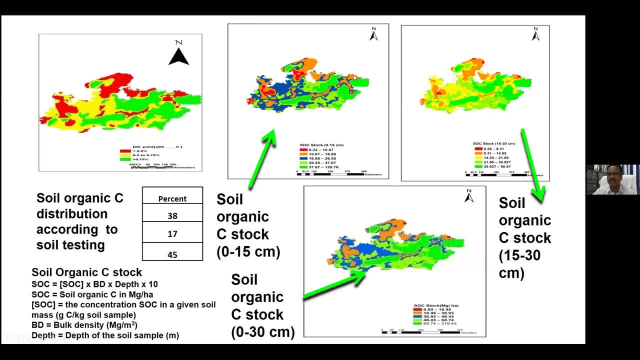 the areas are receiving more rainfall- the eastern part of madhya pradesh and to the central part, despite they are having higher organic carbon content than western part and the northern part of madhya pradesh. so, uh, this is um the one way we did it, and through. 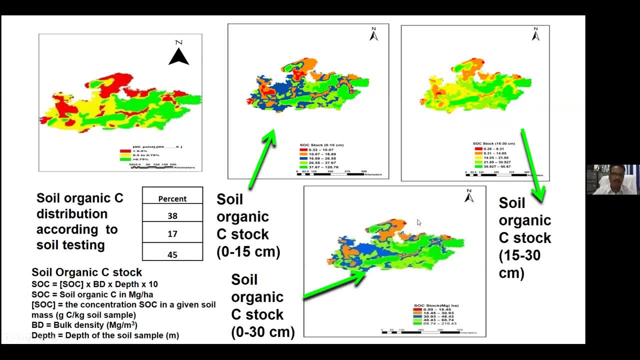 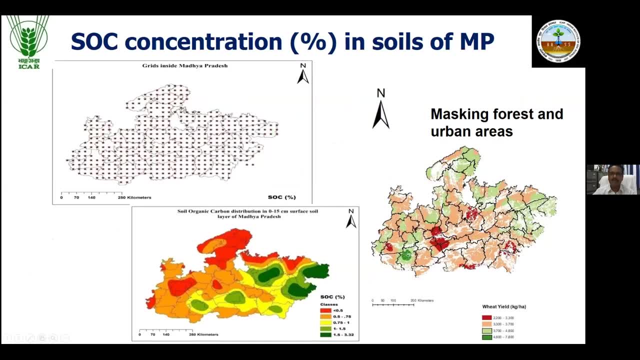 education, um creating techniques. we map those um areas for the whole state of madhya pradesh. then, uh, from this then we try to find out, uh, what are those? we impose the different kinds of management practices. uh, just like what type of crop we grow for this type of? uh, some soils- just like in current season means rainy season- we grow. 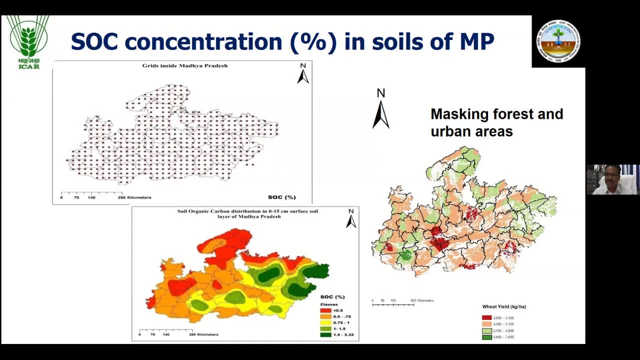 soybean, the mage, then in rubbish season it's winter. you can see that recently which was harvested wheat and chickpea, then other types of pulses also. but my my presence will confine to mage wheat, chickpea and this and soybean also. so these are most dominant crops for the state. 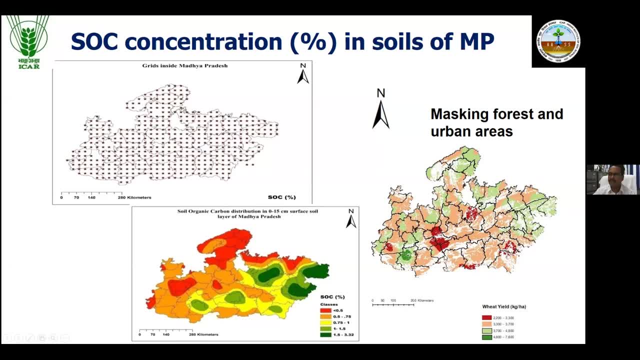 madhya pradesh. you can see those uh. we only targeted those areas having uh acres of practices, so we excluded uh those forest areas as well as those urban areas for our calculations and estimation of organic carbon. and you can see when i talk about any management practices and we see that if you follow certain management. 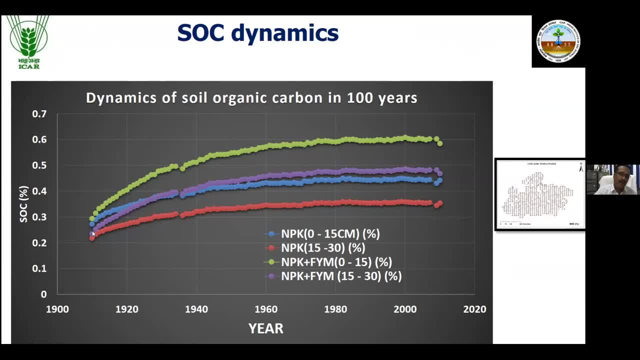 practices for years after years, there is every chance that the soil organic carbon may increase, but after certain years it may come to the plateau. when it comes to the plateau under any management practices, but it takes certain year and that plateau we call it equilibrium, calcium, uh carbon concentrate. that means that further following those management practices we won't get. 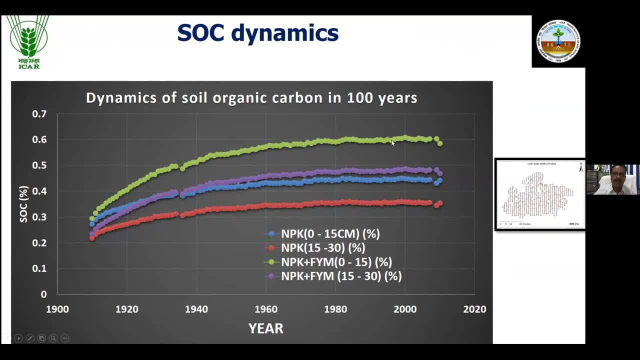 you know, for increasing soil, organic carbon. so here in swineweed cropping system we have followed: nbk means nitrogen, phosphorus and potassium. that means these major nutrients, these essential nutrients will apply ample quantity. that means a balanced fertilization. apart from that, that also, we have added extra of five, uh, five tons of farm and manuals for regular. so this so that when you 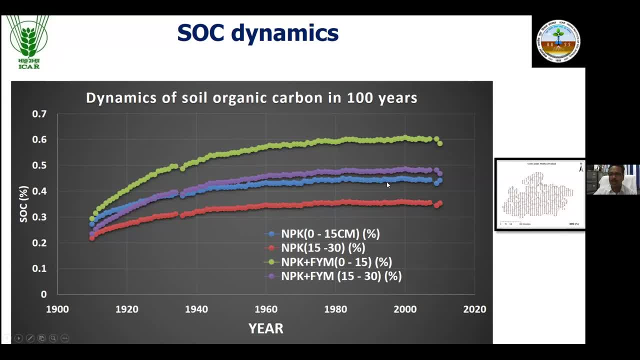 are. look at this top centimeter. when you uh a balanced fertilizer, definitely after certain years it comes to plateau. but when you are farming at manuals means format manuals. it contains more carbon. that means you are adding extra carbon from external sources to the soil, so that is jump in. 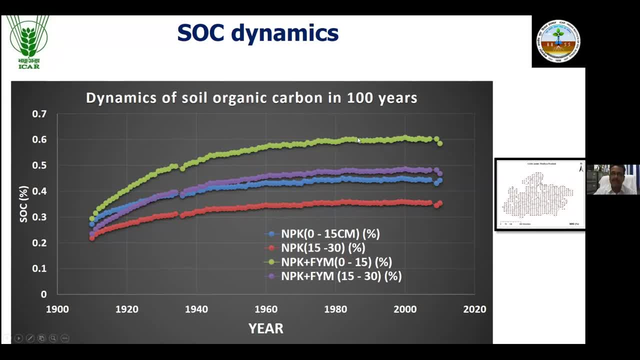 carbon content and you will see that not only the carbon concentration increases, but the time to reach plateau also, that year that also increases. so, um, similarly that is shifting spectra. sorry, shift in the line also in case of uh 15 to 30 centimeters. so this shows that when you follow, 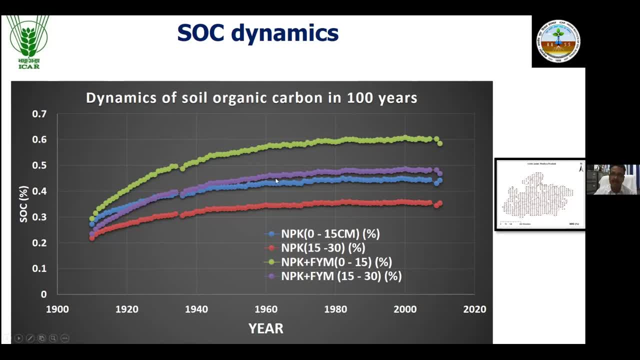 certain management practices, having balanced fertilization, because you cannot feed the crop with suboptimal doses of any type of nutrients. balance means you are giving it ample quantity, according to need and according to the productivity. so in that case, so um that that rich plateau may be maybe 50, 60, 40 depends upon the types of soil, types of crops you are following. once you reach 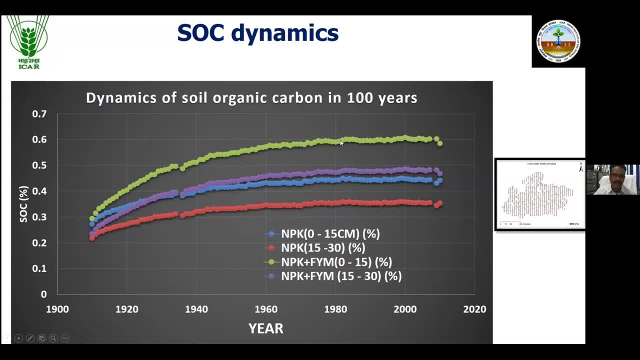 that plateau. if you withdraw this management practice, definitely again this value will come down. so once you follow this by the practice, that means you will find that this soil is having this capacity to reach this equilibrium of this much carbon concentration of this many years, so further increase is not possible. so, based on this concept and principle, so we have analyzed, uh, the carbon. 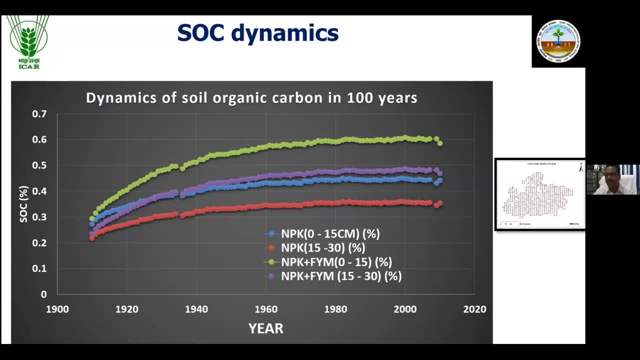 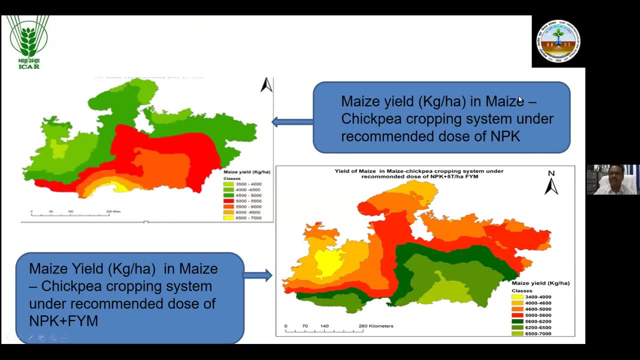 how much maximum carbon we can store on a particular cropping system and nutrient management practices for the state mother for this. so you'll find that we have followed uh for mage in magic system. so you can see the magic. we map the whole state of different range of yields based on our 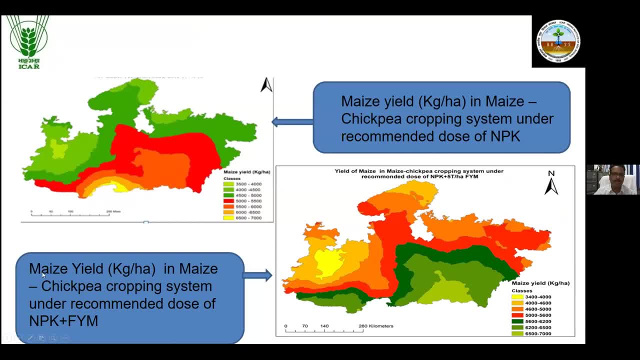 balanced recommended dose of nitrogen, phosphorus and potassium mesil. then in presence of in absence of fom, farm and manuals, as well as in presence of farm and manuals, and you'll see that when you add more carbon to the system- and not only it adds nutrient, bottles carbon and that is increasing. 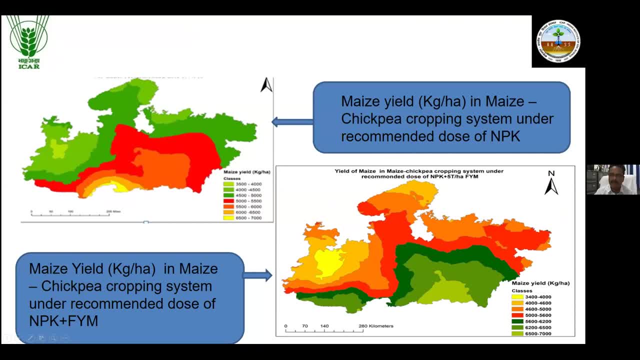 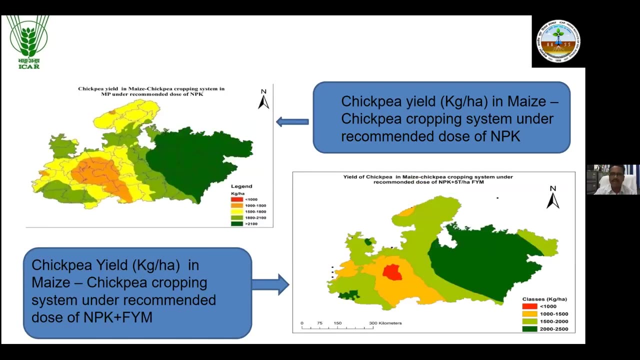 profile. i'll present in different way later on why application of farm and manuals increases a crop field. because it increases carbon as well, as he adds carbon to the soil as well as nutrients to the soil also. next is similarly for chickpea also. you can see that the chickpea under balanced. Betty to工 lang describes the. 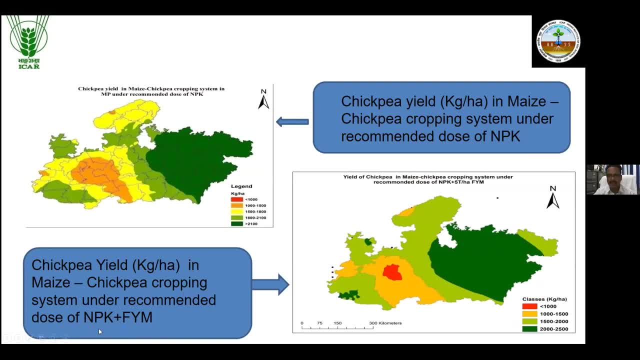 concept specialists last year, fertilization and in balanced fertilizer from our members are we call it integrative nutrient management. integrated nutrient management means in addition to inorganic fertilizer we are adding Organic lighthouse also. so integrated nutrient management is very much important as well, as we are encouraging farmers also to go for integrating moutain management, because we have seen 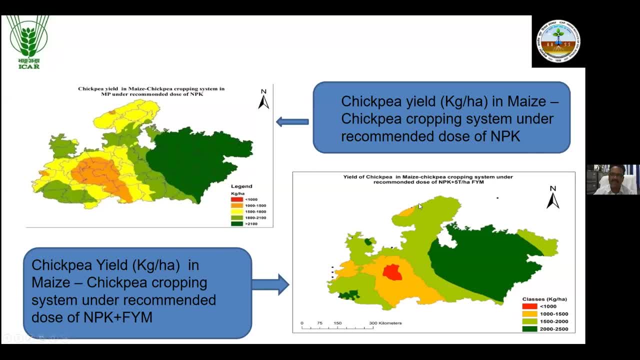 cataloging formal long term experiment integer of 45-year data from our試 결ión long term experiments of 45 years in different parts of india that when you you go for integrating uh integrated nutrient management, not only you are improving the soil health profile but also the carbon content. so integrated nutrient management is very much. 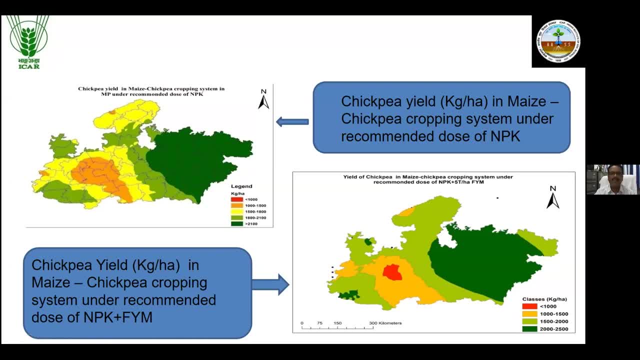 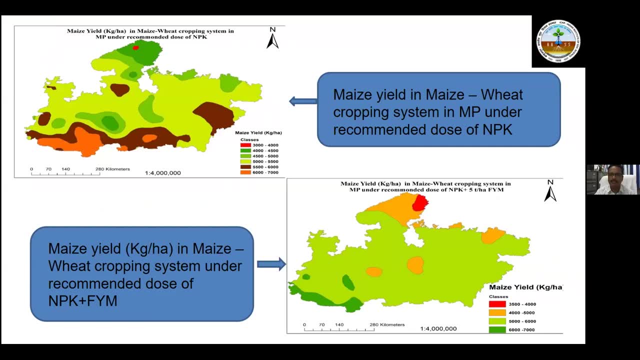 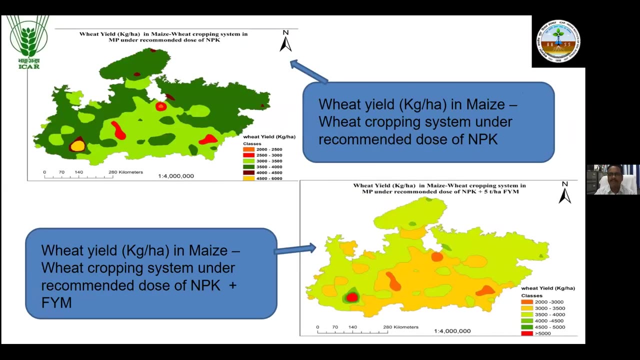 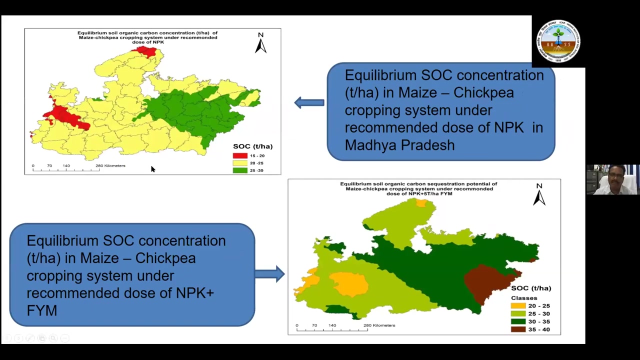 important in this aspect. similarly, you'll see also maize, really measured, proper system in the presence of fom farm and manuals, as well as balance population. similarly you'll see the retail also. so we have mapped for the whole state for different cropping system and nutrient management practices based on those cropping system and nutrient management practices that. 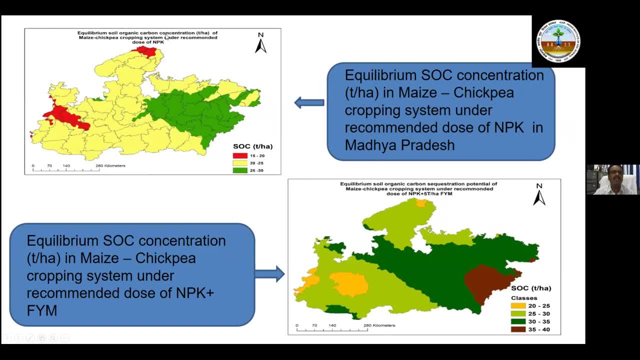 equilibrium carbon concentration. then we map. you can see the equilibrium soil organic carbon concentration in balance, as well as the presence of farm and manuals. so you'll see that when there is presence of farm and manuals you see this range it has. that means it has gone up soil carbon stock. 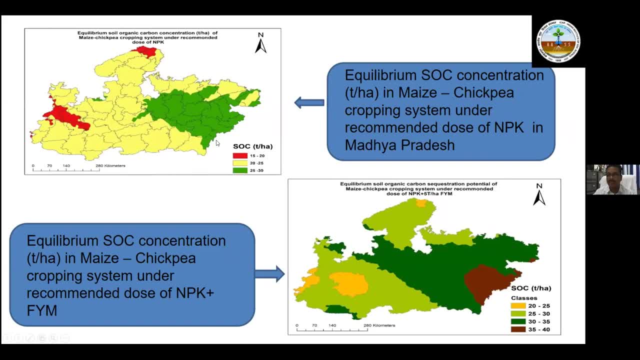 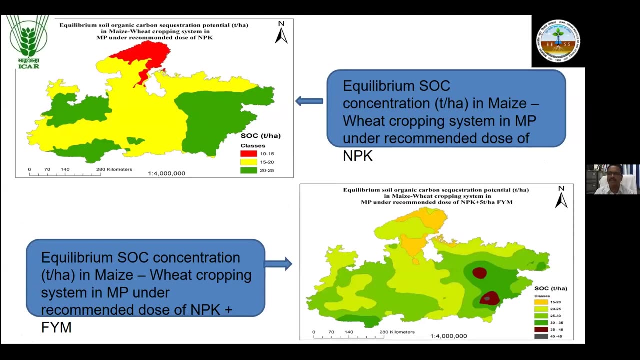 in the soil has gone up and and you can see those increase in the eastern part of much for this, where it is the more rainfall, so that is carbon conservation is beneficial in this region. next is uh, similarly, uh, we also go uh, two cropping systems. so that was. 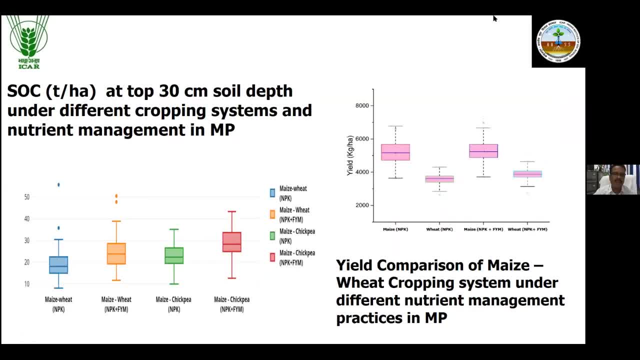 made chickpea and this is measured system and now you can see the stock means carbon soil organ, carbon stock in top 30 centimeter of soil. you can see where you have at a major system in and in presence of army and manuals, that means when we are. 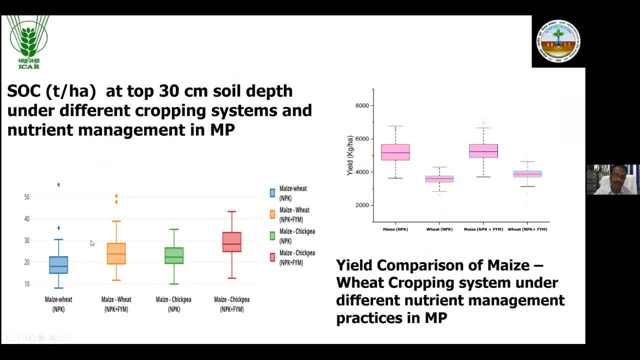 going for only in organic application. but when you are organic, to that that means integrated, that's farm and manual- is every channel that soil organic stock is increasing and similarly in another cropping system also, when you go for farm and manuals. but you can go for also what we compost. 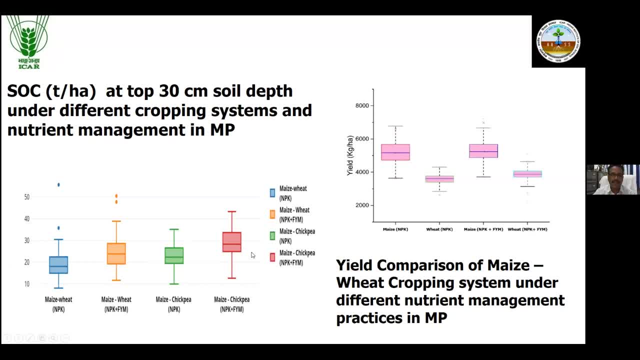 or any type of compost. definitely it is going to increase the carbon content. that means any cropping system, not only the cropping system, uh improves the carbon content. you can see that different two cropping system, this coffee system giving more carbon, but side by side it also presents of harm and also improving the carbon content similarly you. 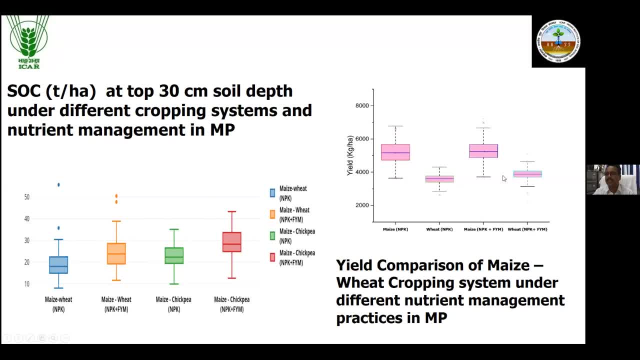 can see the increasing yield. also look at those increasing yield in the presence of farm and manuals. so that means not only it increases carbon, but also it improves uh, probably when you add organic matter or manure compost in addition to your inorganic fertilizers. so based on that, we 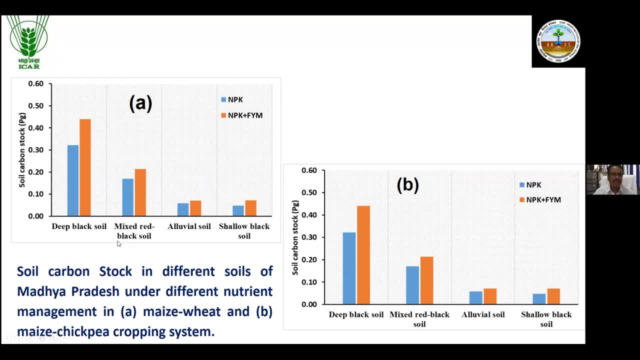 map the whole statement for this and you can see the carbon content of the growing soil with the And you can see. look at this soil-wise again. we differentiated this one soil-wise. at the deep black soils, mixed-rate alluvials and shallow soils, you can see the soil organic stock. 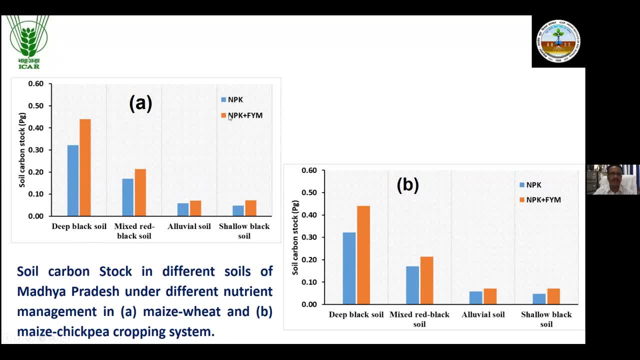 for maize feed cropping system and maize pick-uping system. You can see this NPK means balanced fertilization, when you add farm and manure energy. in addition to that, there is increase in soil organic carbon stock And different soils follow the similar trend. 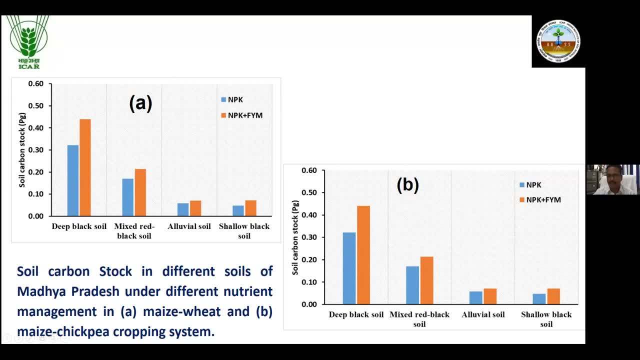 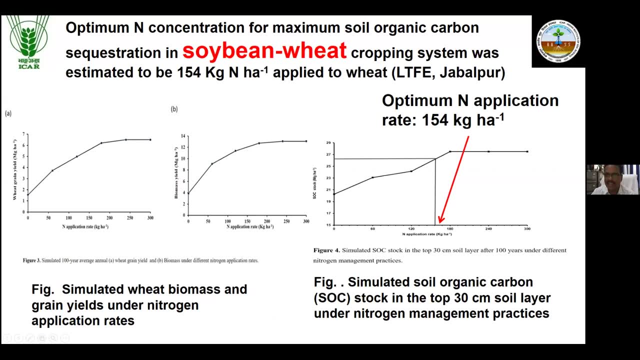 in all types of soils that are in much of this, and it's also in cropping system. Then another important thing we try to find out- this experiment is 45 years old experiment from Jabalpur. We have one experiment, long-term fertility experiment, we call it. 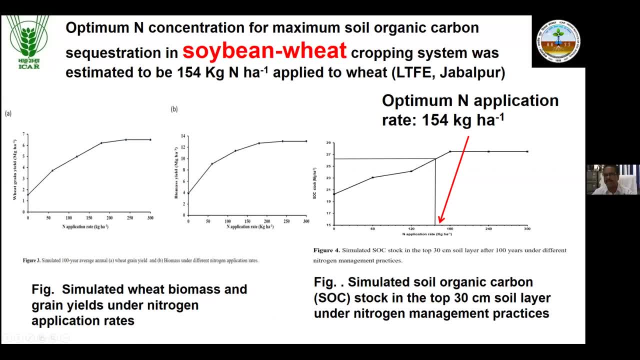 We try to find out what should be the optimum nitrogen application for wheat for maximum carbon sequestration. So look at this, we try to find out. it comes to be 154 kilogram per hectare. So this is one. this is one type of innovation. you can say that. 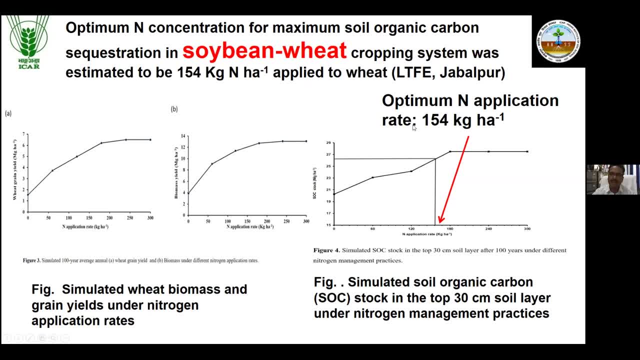 we try to find out what should, But usually we don't apply that much nitrogen to wheat. We go for around 120 kilo nitrogen, Though the crop respond is there to 150, but we don't go because of economics, Because when you increase 120 kilo to 150 kilo, 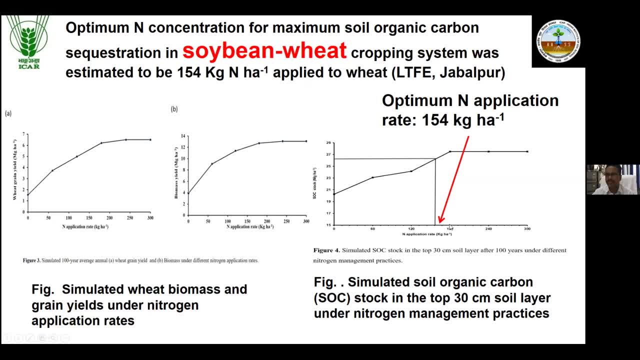 the yield may increase, but it's not economically viable. That's what carbon doesn't see the economics. because it saw that with increasing nitrogen dose your bio-economy will be better. Your biomass production is increasing and crop yield is increasing, though not significant from the 120 kilogram. 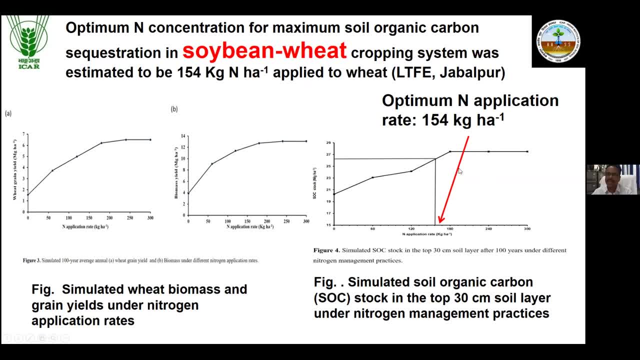 but it adds a lot of- you know, a soil organic carbon to the soil through the roots and roots to exudates. That's why, when you go for finding out the optimum nitrogen concentration for maximum carbon sequestration for wheat, it comes to be 150 kilogram per hectare. 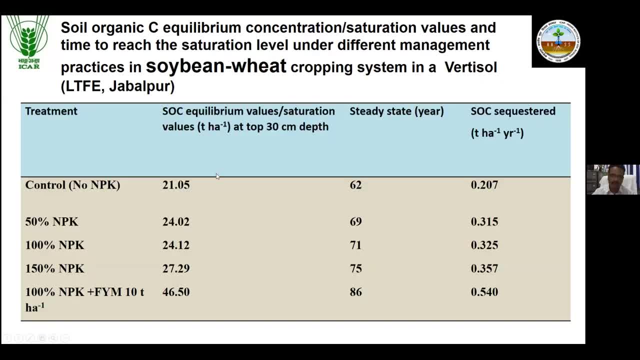 Similarly from that experiment. also, I want to put this one before you just to say that if you apply for balanced fertilization, that means 100% balanced fertilizer and integrated nutrient management, And this is suboptimal means. suppose you are adding 100 kilogram nitrogen. 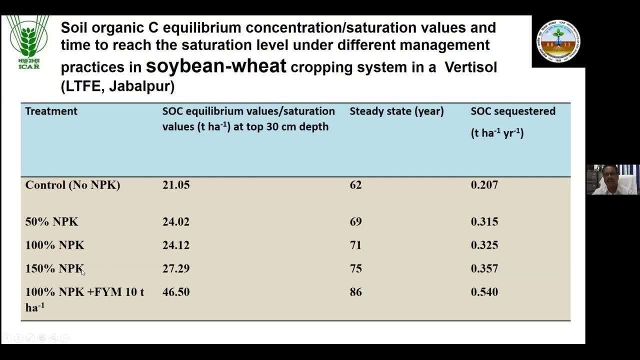 you are adding 50% means 50 kilo nitrogen. You are feeding the crop less. So when you are on 150% means you are feeding the crop more nutrient. but you can see that control means you didn't add anything for 45 years. 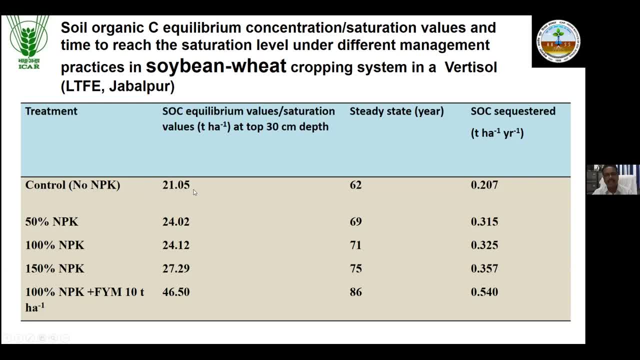 That means that flood didn't receive anything. Only the crop was grown based on the. you know the. you know the available nutrient status from the soil. That means inherent capacity of the soil to produce the crop, That is your soil fertility, that based on that. 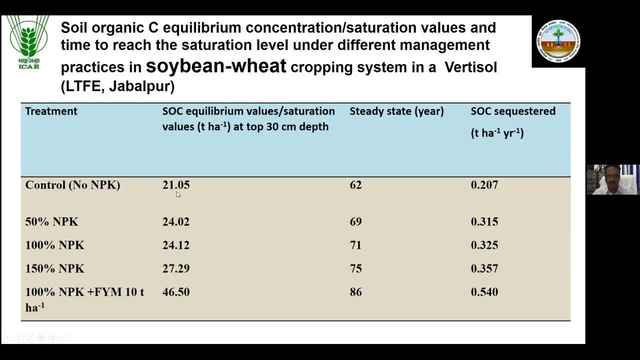 And we'll see that, actually, the crop was growing without crop because, just like your grasses grow, you know everywhere you will find when there is a shower of rain, because the soil having its inherent potential to supply nutrients even if you don't add anything. 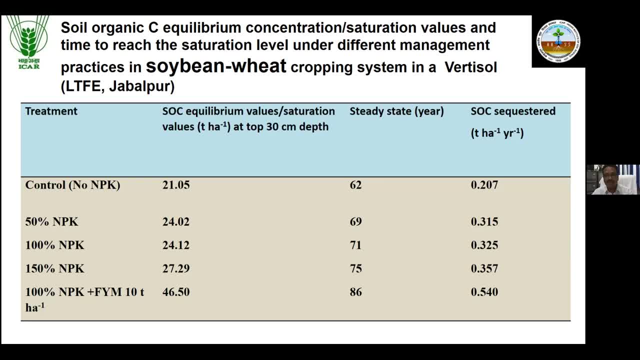 from external sources. Because of our field crops needs more nutrients, because we need it economically, economic produce. That's why you add external sources. Otherwise, if you sow the crop, the plant will grow and it will die also when the time comes. So in that case you can see that how much carbon. 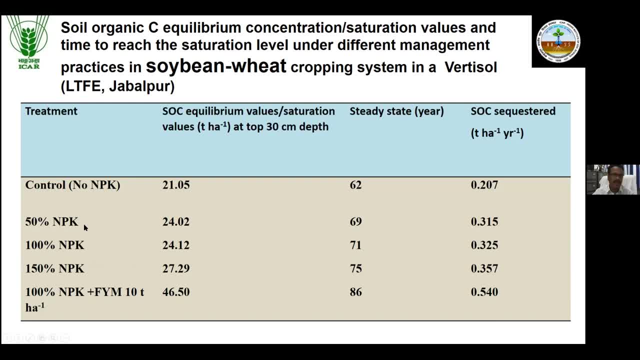 is sequestered per hectare per year, depending upon the type of treatment we are following. for soybean wheat cropping system in Jabalpit, It's 45 years experiment and we find that when you are adding farm and manure, you are adding 540 kilogram of carbon. 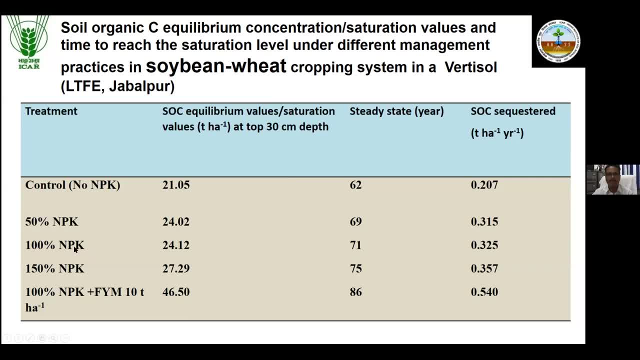 0.5 tons per hectare per year. Similarly, if you are not adding anything still, since the plant is growing so it add little bit of organic matter, it is very less. Even it is less than that it's estimated value. 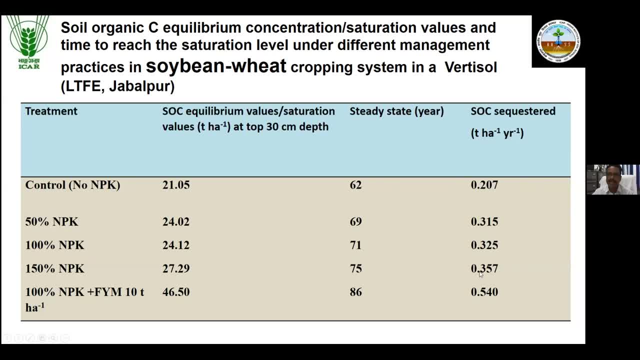 but it may be less than that. But when you are adding nutrient and there's plant growth is there. that is every time that carbon is sequestered in the system And this is the time to reach that equilibrium. Remember in the previous slide. 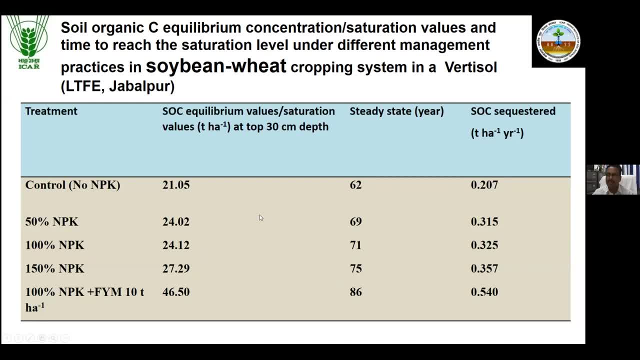 I show you the plateau where actually, when you follow certain management practices, it will go to a plateau position where that further application of a particular nutrient and manager practices will not increase the soil organic carbon. That's what actually the to reach this. 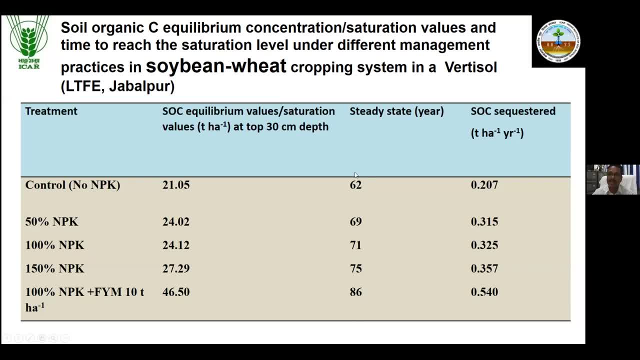 This is for black soils, but if you change the soil types, this value will change under similar management practice. it may not, because the cropping system may change, soil texture may change, soil types may change and this value may be 30,, 40,, 50 years. 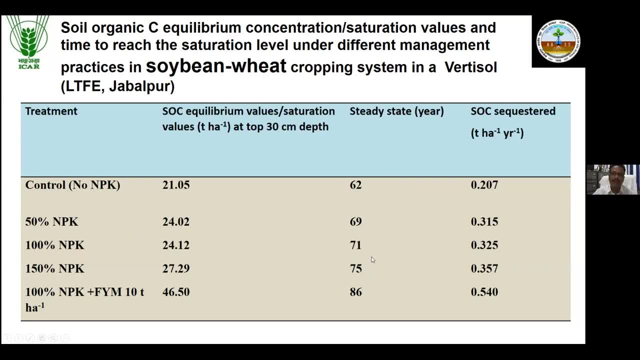 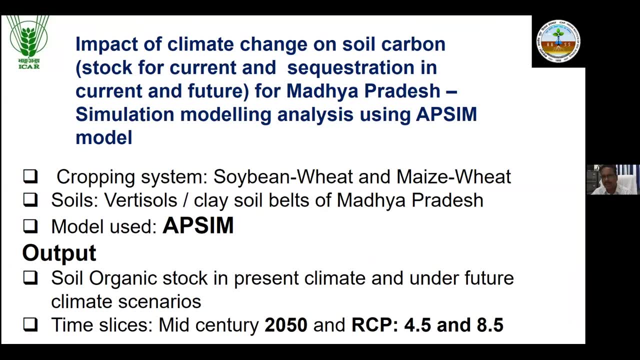 it may be 60 years, depending upon the crop and the soil types. then I want to show you a little bit about climate change impact. we have studied, based on whatever I showed you is the present value, how much we can increase if you follow that. but but in the context of climate change, the 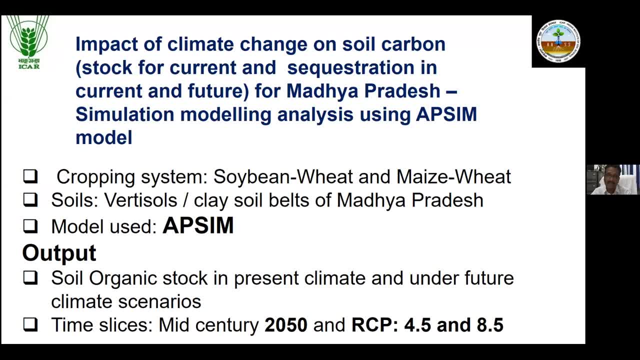 climate change was not considered in type of modeling activities or simulations, but here we are considering only one aspect of climate change, that's mid-century 2050 under RCPs means representative consumption pathways of 4.5- how the carbon will behave or whether there is a return that carbon. 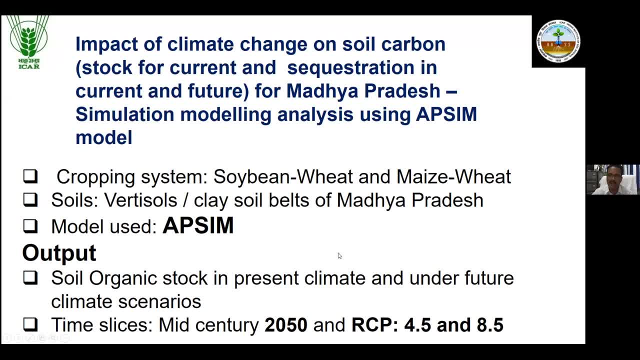 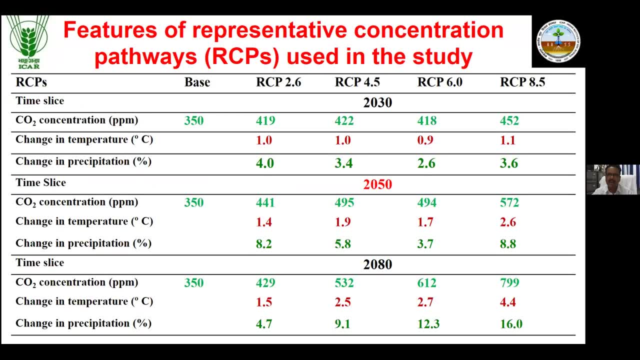 increase or decrease? if it's increase, how much? if it is, how much? so we found that is mixed balance. there are there is increases and decreases, but I'll show you how we work. so these are the for the central India. but you can say that what and I I guess by this time you know what is our. 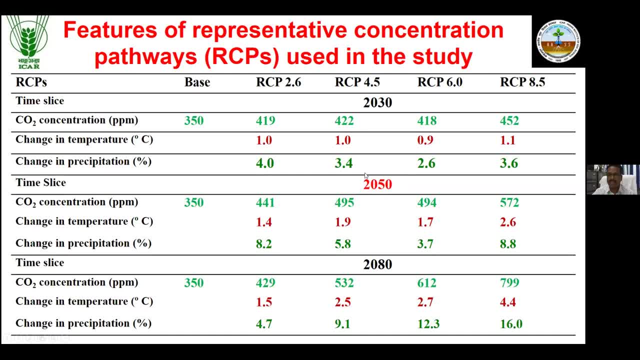 piece and different time slices. it's based on DCM general circulation models of around 15 to 20 models for use for this downstream this data, and we got this data and we expect that in Madhya Pradesh, that is, in future climate, that is increase in rainfall. if you look at the change in precipitation means. 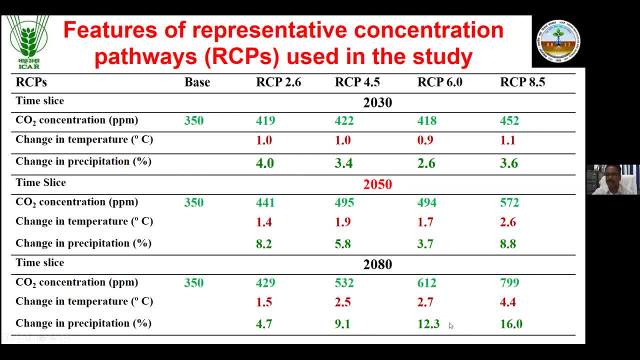 rainfall increases there. so we are expecting more and more rain in our future climate scenarios. and what are the temperature? temperature also going to increase. so we expect that. because we are targeting 2050, we are expecting at around 1.9 degree increase in temperature, having 500 ppm carbon dioxide. 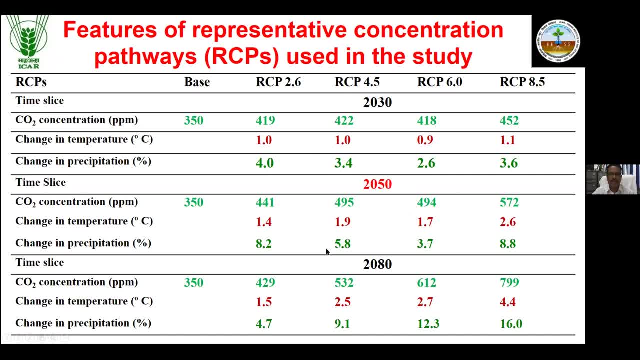 concentration under RCP footprint and your precipitation increase will be around 6%. that 6% average. that can be, you know, much more rain in a short period of time and that will be too difficult for us to handle unless other way you follow certain conservation efforts, practices, conservation, or is a? 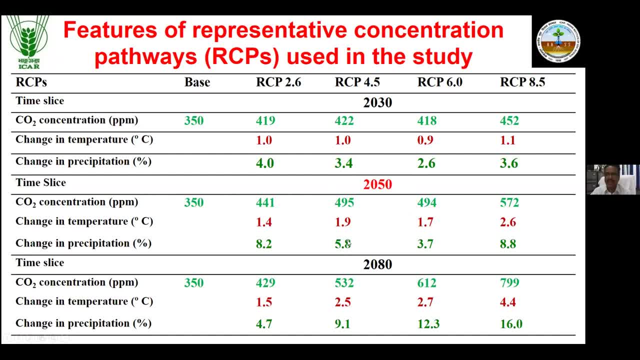 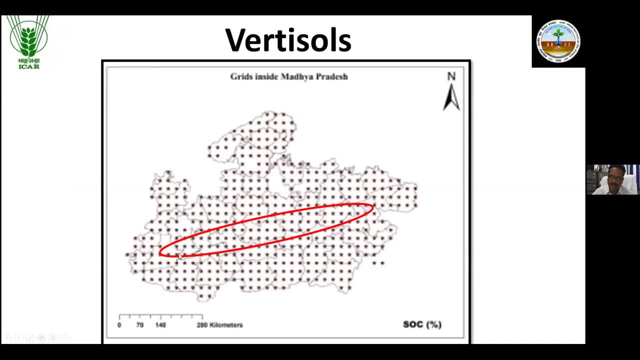 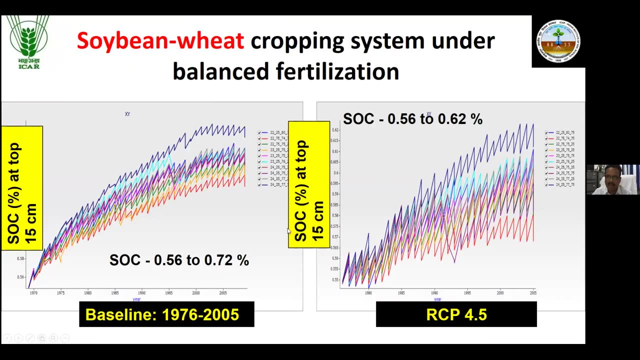 major question any kind of how can we just get a better discussion on this question? I think about the right between the two. what if the soil are baking, or their, your indoor, or your indoor? they can not have a lot of water. well, if they can't have a lot of water, 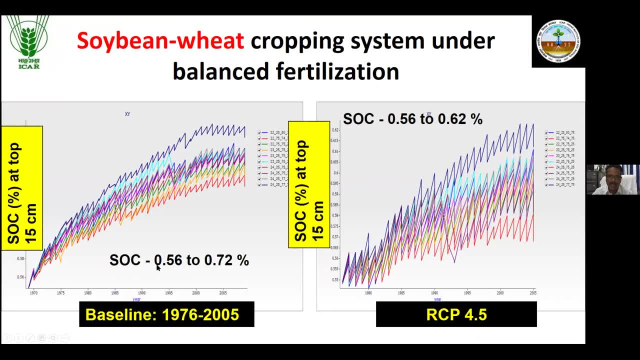 and they're grew very nicely in this region. we have to determine if your soil- and we can see that that increases from 0.5 to 0.6 baseline- means. this is what we are following now. but when you go to RCP 4.5, where we increase the 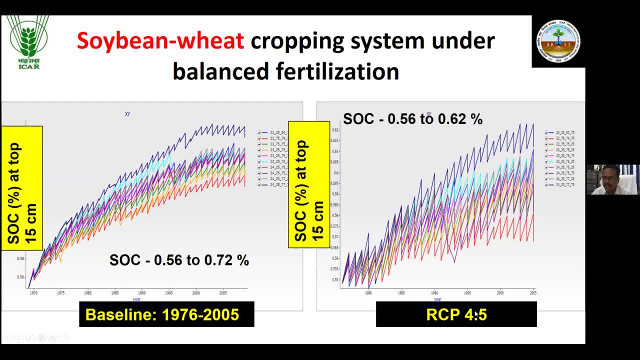 temperature by 1.9 degree and carbon dioxide concentration 500 ppm. for this 5 minute system, you will be surprised to see that there is not much decrease in solar and carbon, because two things comes into play here. one is carbon dioxide, next is temperature, and temperature. you know that it has. 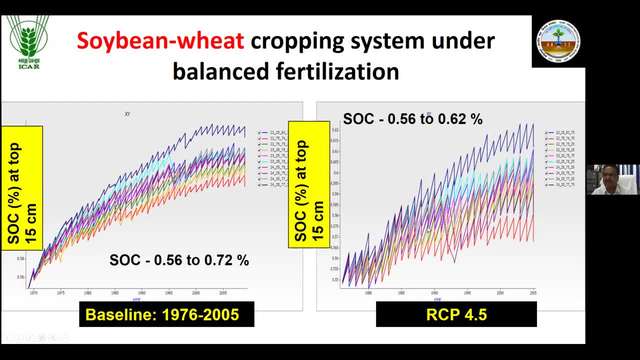 negative impact on crops- anybody, because increase in temperature is not favorable to anyone. similarly, it is not favorable to crops also, but side by side. when it is talking about carbon dioxide. in that case, increasing carbon dioxide concentration, it favors the plant growth. we call it fertilizing effect of carbon dioxide, so C3 or C4. 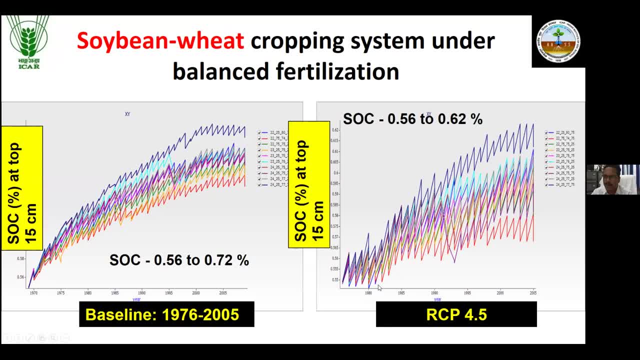 plants depends upon the types of plants. they respond to the increase in carbon dioxide concentration. so C3 plant, they respond around C3 plants they respond around C4 plants and C3 plants they respond around 600 or 700 ppm, but seaport plants they may go as high as 900 or 800, 800, 900 ppm carbon dioxide. 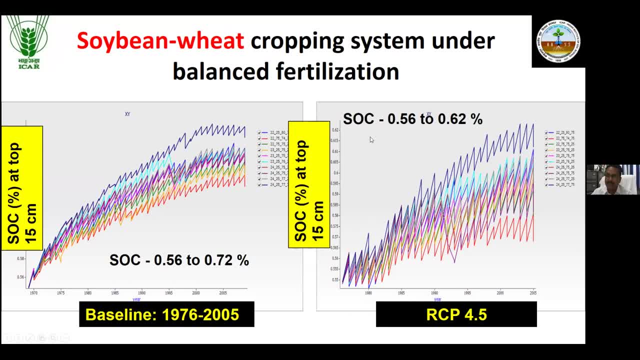 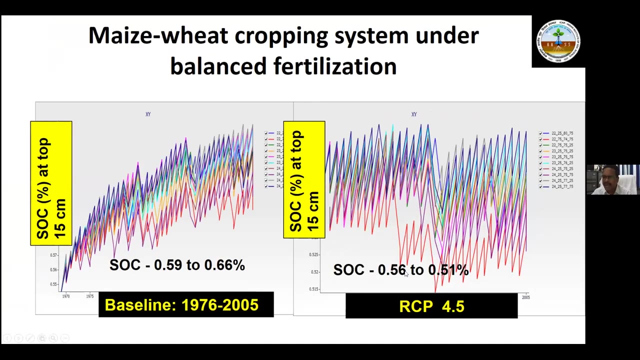 so this carbon dioxide ppm or 500 ppm, that must have favored the swineweed crop. the growth has increased. that's why increasing carbon dioxide is sometimes offset the negative impact of temperature. so in the interaction of carbon temperature that might have affected the crop, but in another also uh, but major system, there was slight decline, though it is not significant. 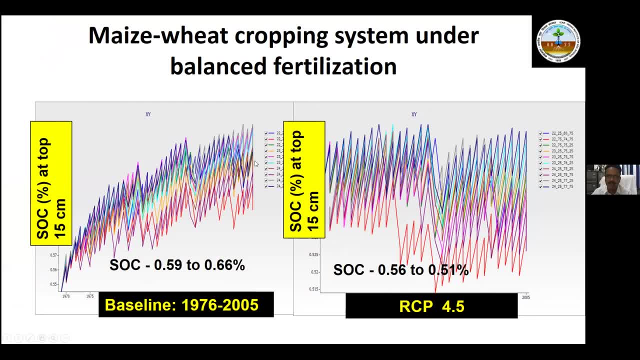 in this case though, normal case because, as you know, you follow certain management practice to increase, but temperature increase with carbon dioxide increase in concentration. still there is decline in major system, but it didn't see it, we didn't see in, so i mean as well as mhp system. 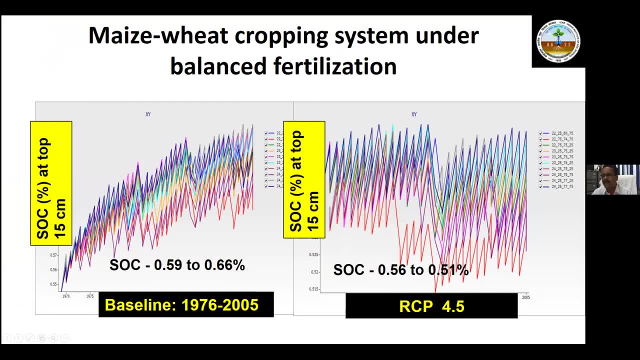 that means it shows that when you add anything legume to the system it becomes more resilient. change major system: both are cereals, but uh made chickpea. chickpea, gram of gram. that actually is a different cropping system. so it shows uh different uh phenomenon and that's what actually: the carbon. 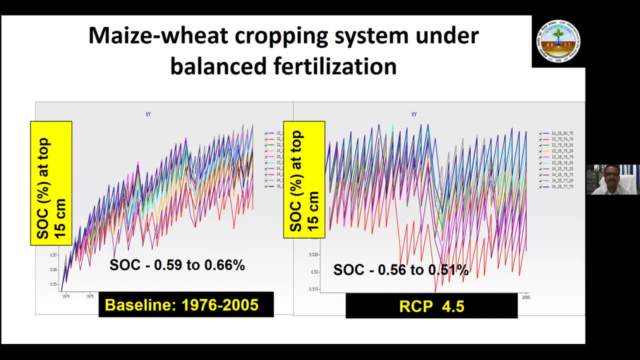 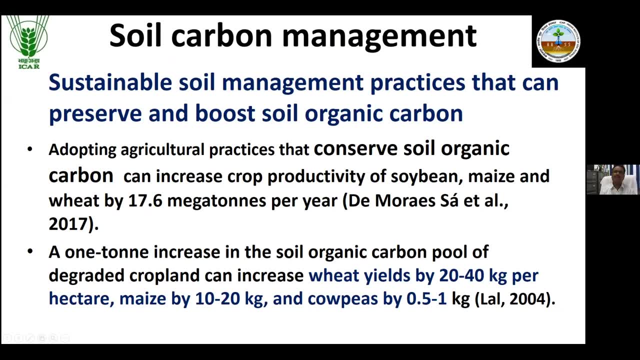 concentration decline is less in that case. so i will again uh come to this um, because i'm coming to the last part of my presentation. what are those soil management practices we should follow, uh to boost soil organic carbon? so i have some certain examples, though in india we have plenty of examples i have also shown you. 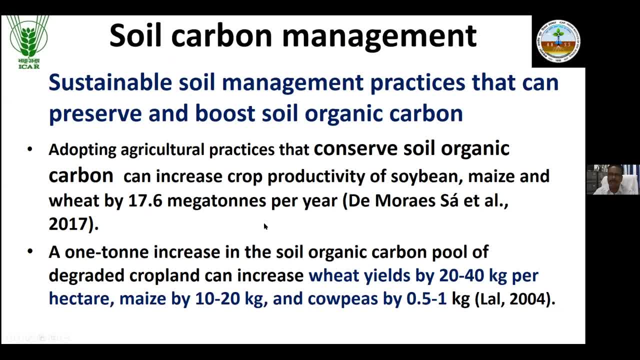 examples: if you follow the um management practices, just like coffee system or nutrients, so definitely you are going to increase the carbon content. that already you. you saw in my previous slides but i am showing you one, some examples adapting the practices to conserve solar carbon carbon. those are the practices which conjure solar organic carbon. that means that organic uh, that. 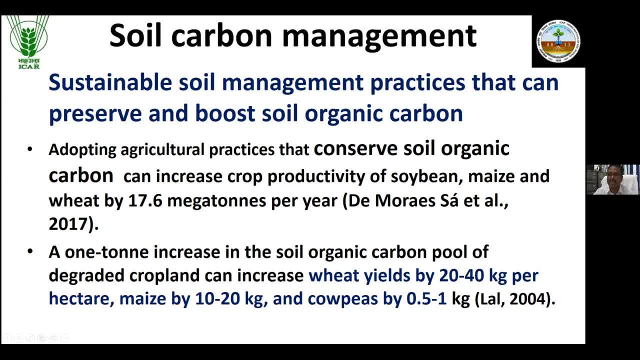 conditions that you have to follow uh conservation protocol. use the best plants- Maineunktl people in india. they conservate organic biota. so this is the term that i willant. we have broken down into many available achoes. i already know um. we have to do a very good research on underground. 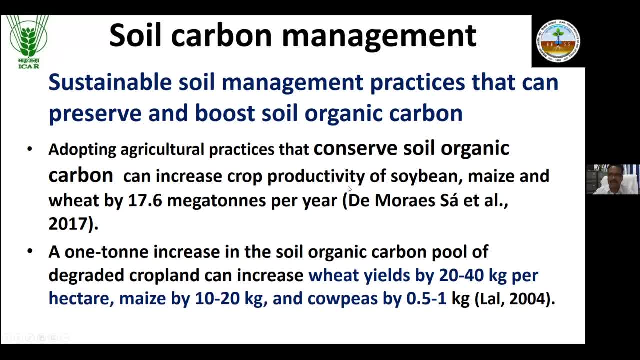 transport here. so it has been estimated that once you conserve the carbon you are increasing the crop similarly. one ton of increasing solar in carbon pool degraded the crop. any degree of crop land can increase weight yield by 20 to 40 kg per hectare, and other crops also. so that means how carbon 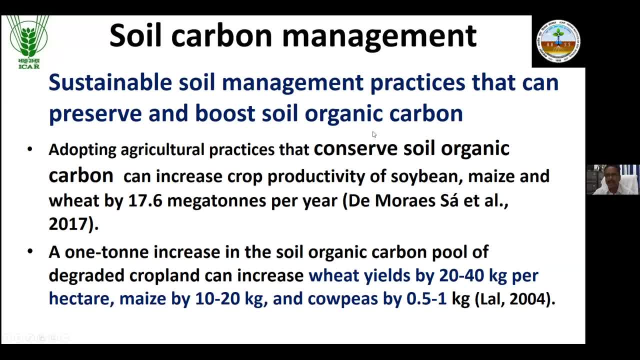 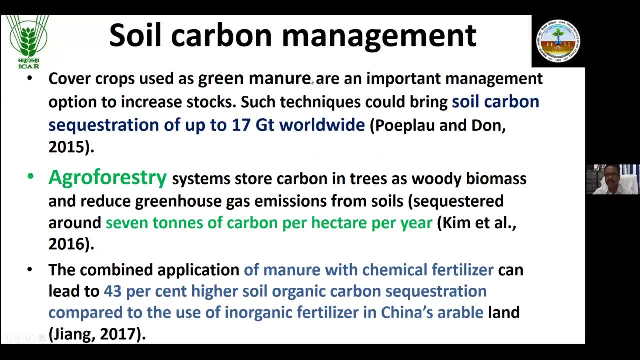 help in building not only building soil fertility but also increasing crop yield similarly. so one concept is green manure. i know you are all engineers, you might be knowing, but green manures means any problem. the leaves and the whole plant is also added to the soil, so they are carbon, and it has been seen that such techniques could. 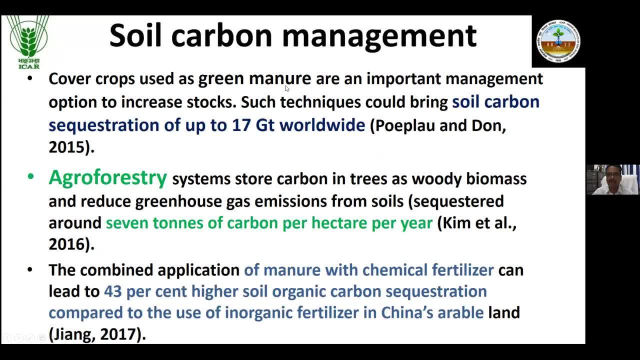 bring soil carbon to 17 gigatons worldwide if you follow- but not many people follow this nowadays, but still it is- it should be followed in the present context of climate change when you see that carbon- improving solar, organic carbon- can mitigate the negative impact of climate change. 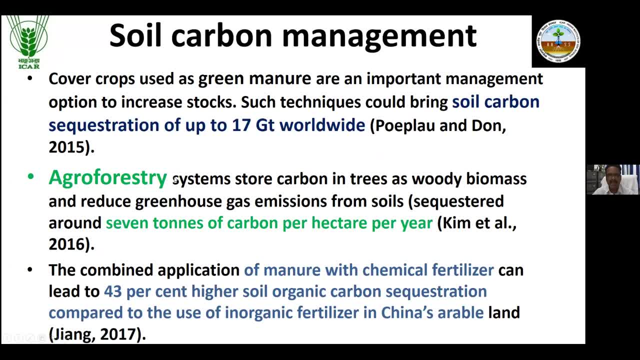 and most important is agroforestry system, where agriculture and forestry goes together. this system is most productive system so far sequestration of carbon is concerned. it's been estimated that seven tons of carbon per hectare per year can be sequestered through this process, and next is combined application of: 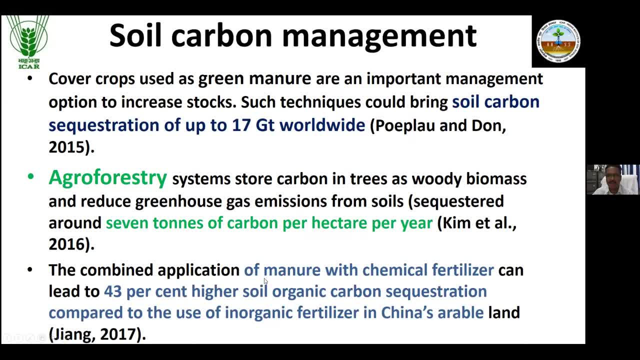 manures with chemical fertilizers. that we call it integrated nutrient management. i presented also some slides from jabalpur so can lead to 43 percent higher organic carbon carbon those they have seen in china and india also. we have seen all our soils from all experiments, all india. 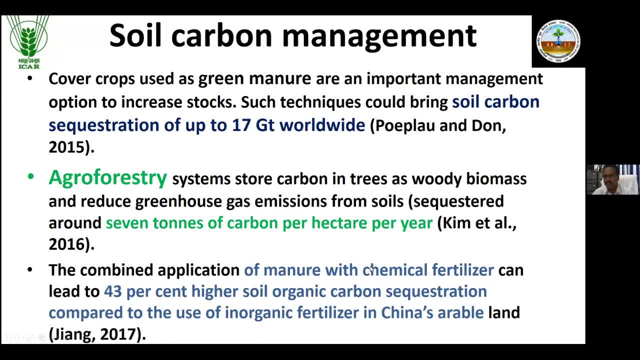 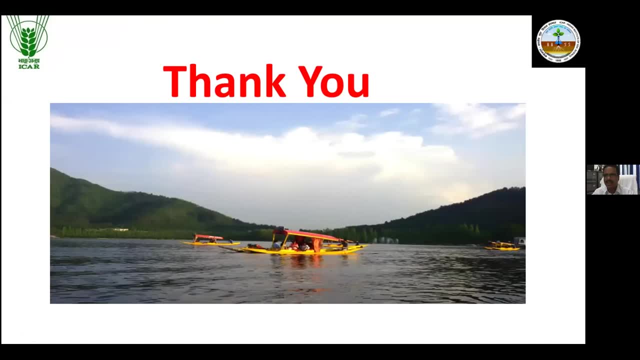 coordinated research projects and long-term fertilizer trials in around 25 universities. at university in india, we have seen that integrated nutrient management improves the soil organic carbon. so thank you very much, and thank you very much giving me opportunity. so this is the end of my presentation. thank you. 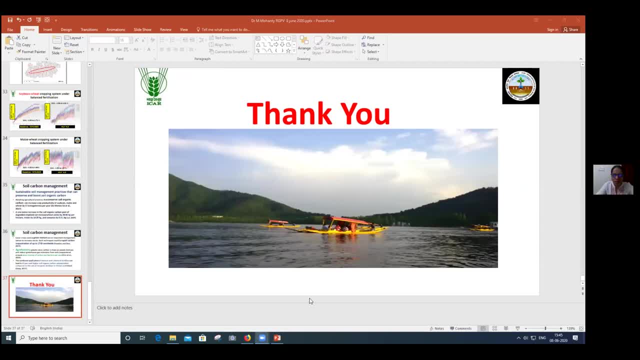 sir. thank you, sir. uh, i would like to request all the participants. if you are having any query, you may raise your hand or you may post in the chat box. yes, please, jitesh, are you there? ravi, pratik, pratik is in another meeting. ravi, who is there? uh, no, nobody one, only me. 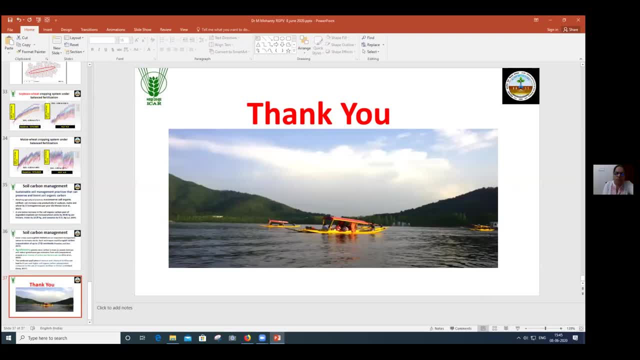 jitesh. i'm not able to see their hands, so anyone who has the question- i know they are all in india. this is a different subject for them. it is very relevant. if we are talking about the climate change, you can't neglect this topic. yes, you're right. 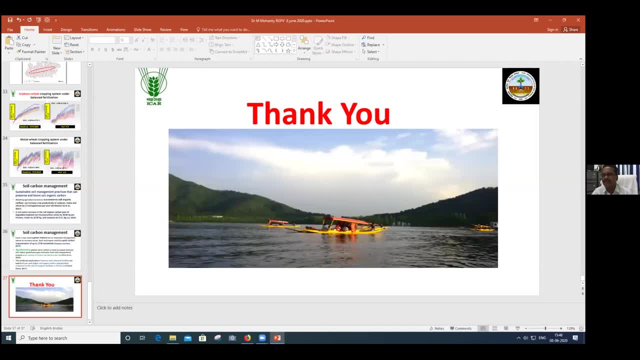 yes, because, um you, this is actually whole agriculture system. it can be source, that can be think, as i mentioned. so we always try to make it a sink rather than source. so we always use advanced techniques to measurement, all just like medical variance techniques. we say that from that instrument we can say that. 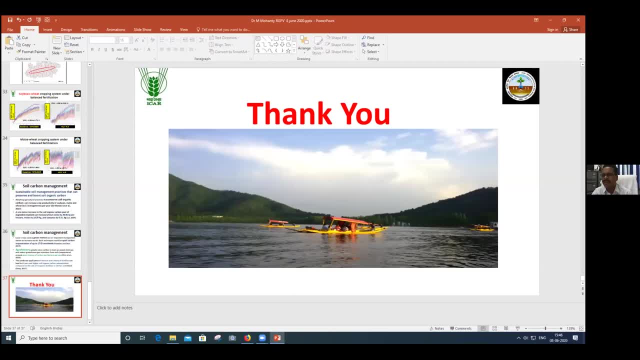 whether your system is carbons negative or carbon positive. so so, so the most important is that what type of management practice will follow and what type of crops are you following and property system and what techniques you are using, because we need always for such type of research advanced. 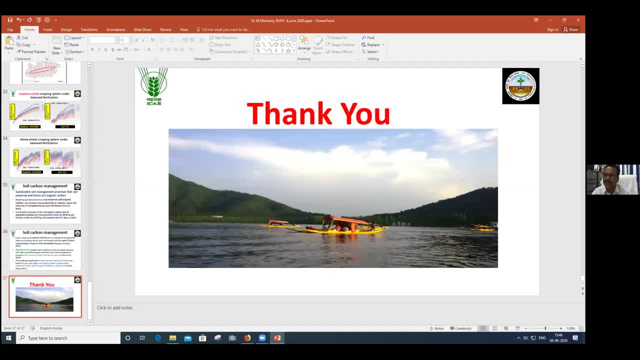 techniques. so advanced techniques are most important because they help us, to you know, give more details about the particular system. because, deliberately, we have included this topic of soil, organic carbon? because nowadays we are talking about the new technologies like iot, artificial intelligence, for the application of this. this area needs to be understood by the 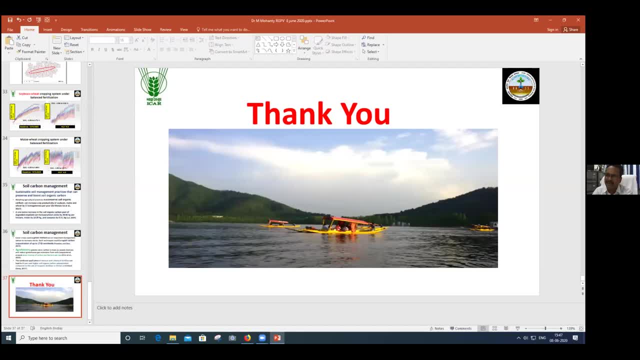 engineers also. yes, actually that's there for engineers. you know remote sensing approaches, because that's also most important one, because your school of environment and all they are working. so i have shown the soil organic carbon situation process. you will see that i have mentioned one near infrared and mid infrared spectroscopy. actually we are using those. 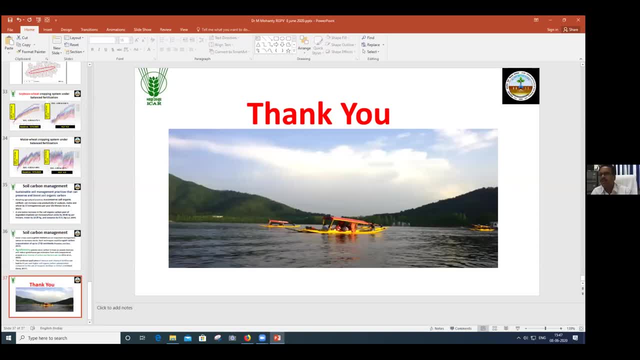 techniques to estimate uh, soil organ carbon. we can go to the field directly, you can take or you can bring the sample to the lab. you can also use that technique even through remote approaches to satellite. also, you can map whole country. so and once you get the map done and you 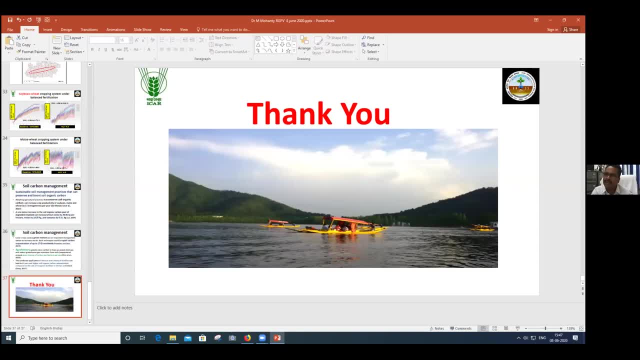 can use the modeling- advanced modeling technique. you can find the whole profile solid and carbon once the surface is done. there is a procedure we can make full profile carbon content. so this, this technique, is also good for engineers. i can say that and they can. they can help us, you know. 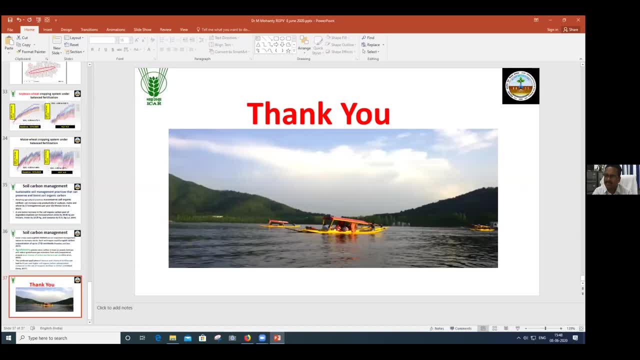 in this regard, so in remote sensing application particularly, and others of course, all instruments, engineering techniques, all the engineers they have developed those instruments. so engineering is always important because so far how much techniques are concerned, ma'am one sorry sir, one participant has posted to me that i am not so much. 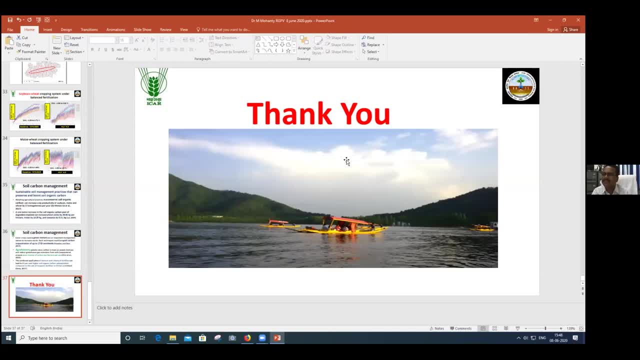 aware about the soil management, but it helps me to improve interest in soil management. thank you so much. yes, because i know it's all engineers, but you know, without agriculture, because agriculture is there. so, if i want to stay one line, our late prime minister, jawaharlal nehru, once said everything can wait, but not agriculture, because 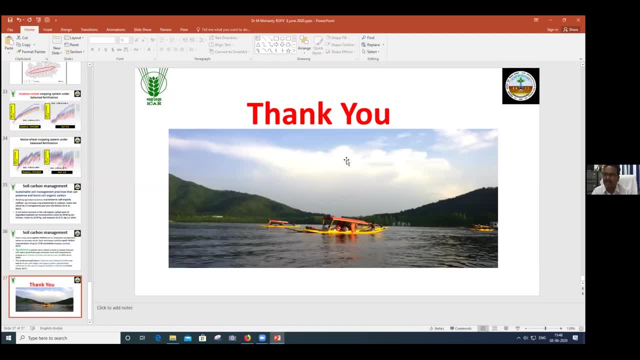 it fits the nation. so if, just like corona in the kobe 19, you see everything start but our agriculture, you always get food. you always get vegetables because farmers are there, they are working, they can't stop. if they stop means you, you'll be hungry. 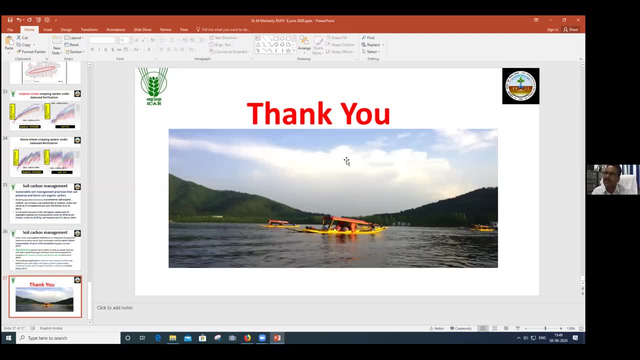 so everything can wait, but not agriculture. so it's a continuous project. we have been doing it for thousand years now and we'll do it without this. it is not possible so, since we need to be going to continue for years to come. so every management practices, whatever we follow, definitely. 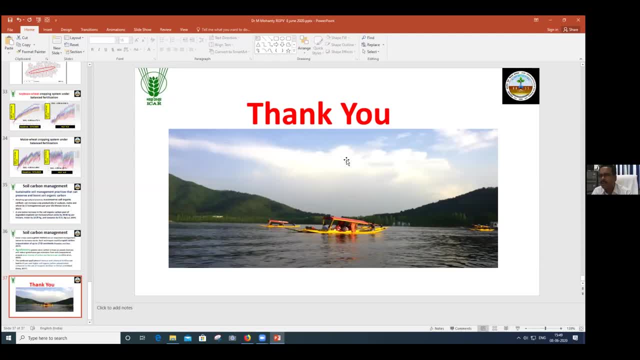 that actually impact our environment. that also um change our climate, that also change our water cycle. so all management practices lead to greenhouse gas emissions, like methane, nitrous oxide, because we are adding a lot of fertilizer, so in that case we are expecting nitrous oxide emission and nitrous 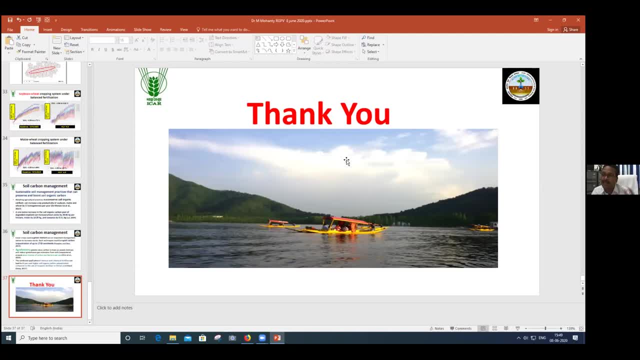 oxide is 300 times more potential as greenhouse gas- no potential- than carbon dioxide. so 300 times little bit concentration of nitrous is more potent, no, it's more dangerous than carbon dioxide. so definitely when you are adding. you know, in a big country we are having um 141 million hectare area. 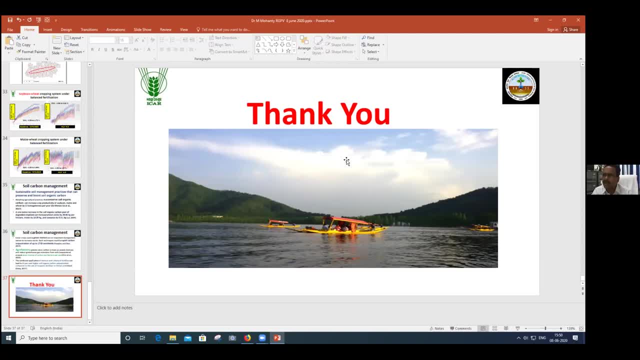 million hectare. we are adding lots of thousand, thousand tons of nitrogen fertilizer. you are expecting nitrous oxide emission also on different so. agriculture is source, but we want to make it, you know, sink through our better management practices. that's what actually we have been working for. so 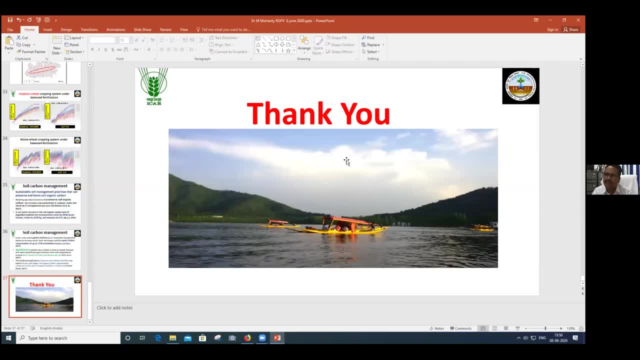 many years now. so what should be the best- and we have observed that that's the presentation was all about- what type of money, the practice the farmers should follow and so that we can make the agriculture of the farmers, our young farmers, not because we want you to be taking care of the farmers. 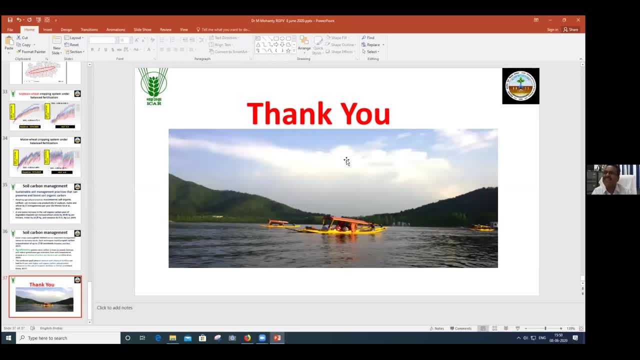 and the technology and all of that, but we will be taking care of the farmers in the future. so thank you. so it to absorb many things and it also, um, when you add anything with soil, if the soil solution most important, those chemicals that are soluble in soils, that may contaminate, but still if they. 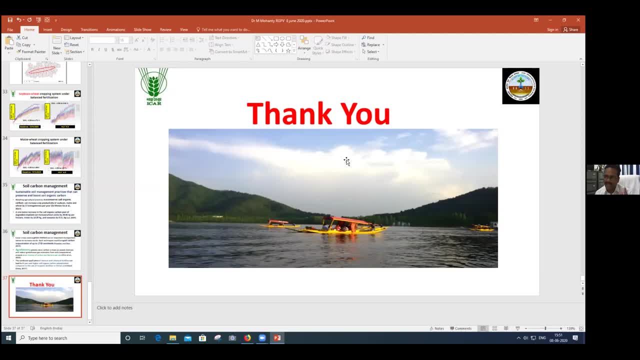 are biodegradable, the microbes present in the soil. that's why, without microbes, cannot think of the world. that's why i told in the very beginning: so without like so microbes, they may degrade. you know that some of the chemicals may be biodegradable. they can be, you know um. 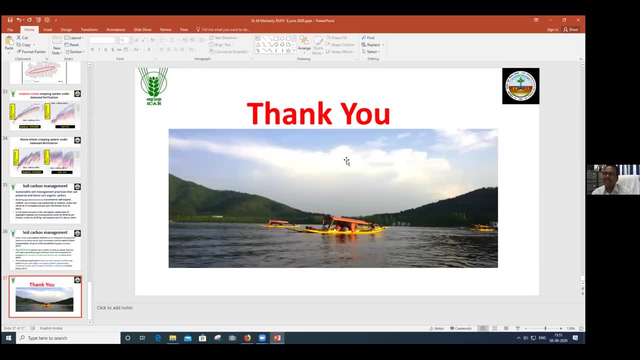 decomposed are forming another compound of easily, maybe a long chain reaction, maybe simple sugar, simple amino acid, something. so that is that may be fun, but if that is not firm, if they are not biodegradable, that's because polluted. if they are biodegradable, definitely. 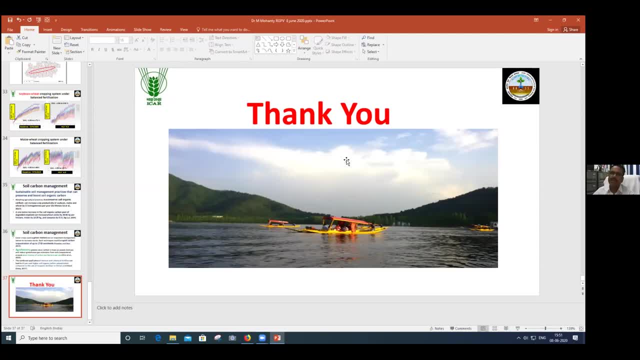 this will come to another form- which are not poisonous, which are not polluting our soil or our environment or water bodies, then that is a chance. but carbon, carbon, having you know, carbon also presents us. it's actually filter to the soil, water also, i told you one, and it also presents. 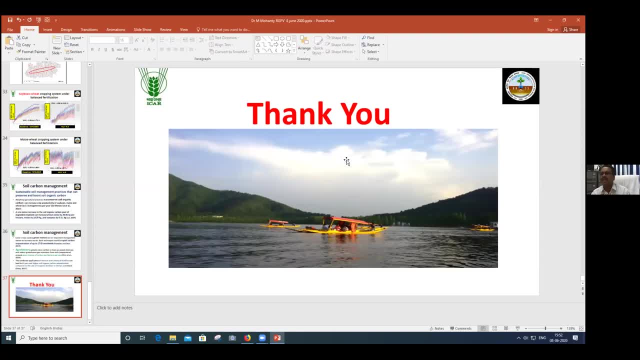 up those um garbage pumps, complexes, because it has been so many compounds, you know so many functional groups so it has so many charge negative charge sites and that helps because its carton exchange capacity is very high and that is absorbing some heavy metals. so presence of your 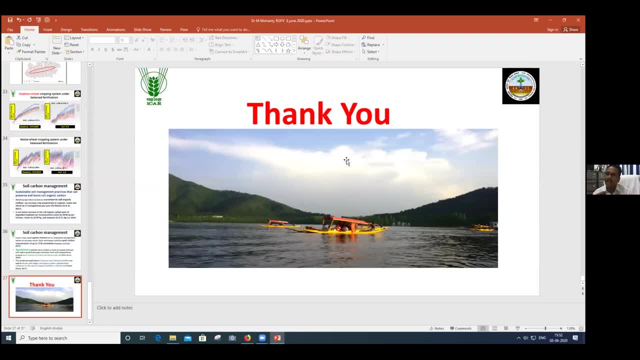 carbon definitely attracts those heavy metals and binding, we call it chelating. it forms a chelate, a constant compound which won't allow to release to the soil. so that's why it will reduce the pollution level presence of your carbon also. okay, sir, thank you so much. sir, this is duba here from 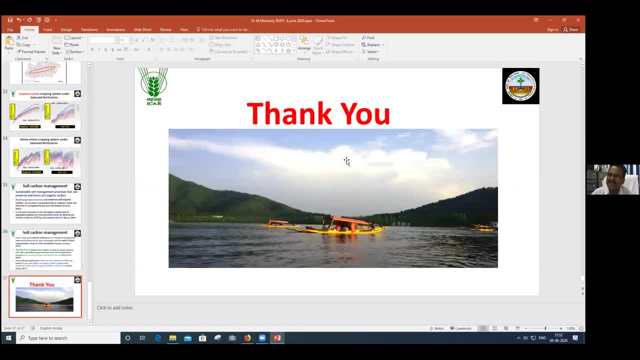 indoor institute of science and technology indoor. okay, it was really highly informative, sir. thank you. thank you so much, sir. welcome, most welcome, if you have any questions. thank you, yes, ma'am, thank you, uh, good afternoon sir. good afternoon, uh. yes, sir, this soil sequestration is something new to me, because we have heard of forest acting as a thing for carbon. 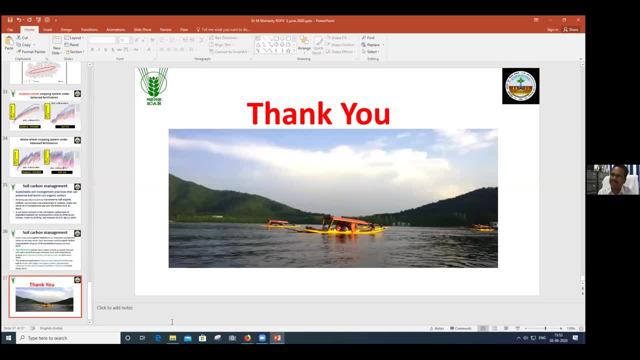 dioxide, yes, but then soil alone can sequester carbon is really very surprising, and it's good to hear that soil can act. act also sing for co2, yes, but so the thing is, to what depth does soil sequester carbon? because in one of your slides i saw it was top 30 centimeter. yes, 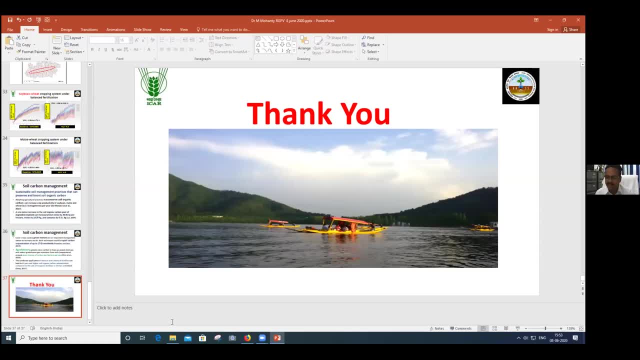 yes, actually, why i mentioned that? also? because 75. because when you talk about agriculture we talk about the crop plants, what crops we are taking. so most of the plants, those cultivated, we are cultivating, except the deep rooted, like two or other. they are going deeper otherwise others. 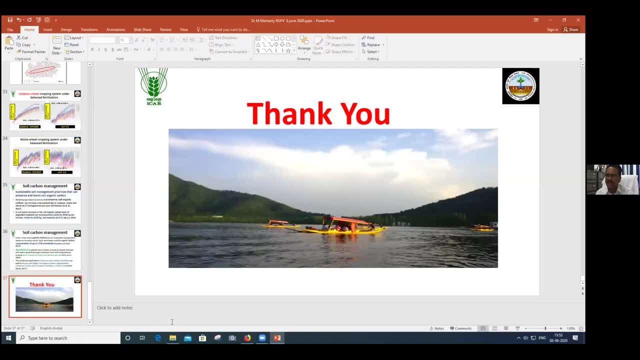 just live in. the 75 percent of their good zones are in the top 30 centimeters. but sequestration can be at the low depth because we also develop a concern. so we want also the soil to be sequestered. We also want to trap soil below 30 or 45 or 60 centimeters. 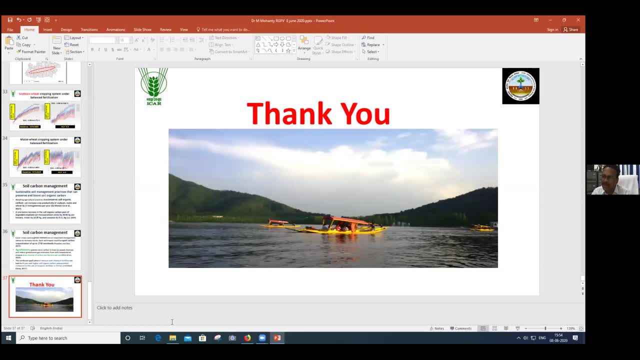 so that it will not expose to the atmosphere. You know that once the carbon compound is exposed- that means the presence of moisture as well as temperature- then decompression process microbes start eating it. So decompression process starts and carbon dioxide will be released. 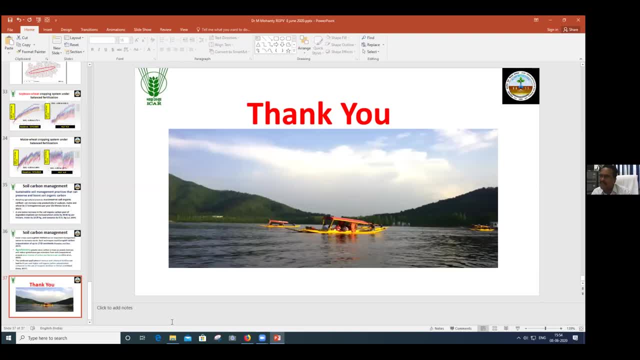 But once it's trapped in a deeper part of the profile. that's why those carbon which are there in the deeper part of the profile, they are stored and sequestered forever, Unless otherwise we go for deep plowing, we don't go for excavation, expose those subsoil. 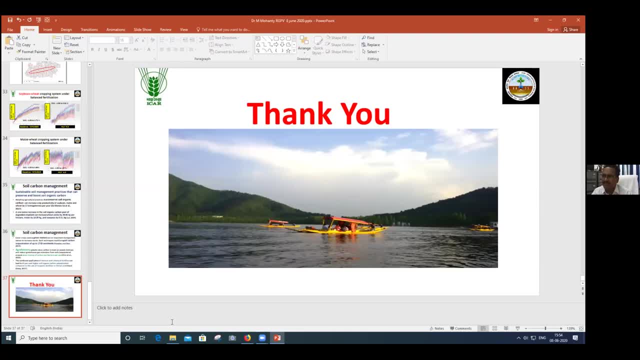 then there is a chance, Otherwise it will be there. So that concept is because I presented only 30 centimeters, but so far carbon sequestration is concerned, we always go for 1 meter depth Because we want to see that. 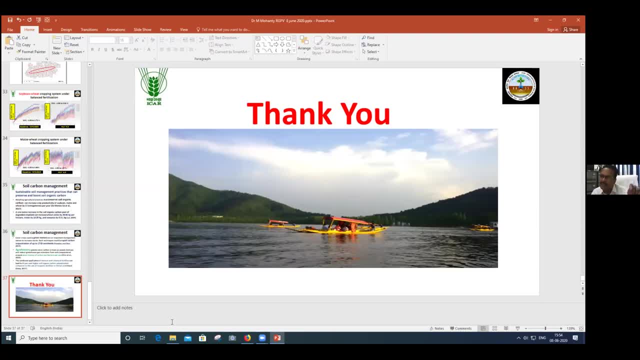 That's why one slide I have shown 3 meter depth. also, it considers both organic as well as inorganic, But I am more concentrating on organic. So organic one, because where rainfall is high, if you don't have carbonates or bicarbonates in the soil, then we don't talk much about soil inorganic carbon, But arid regions like Rajasthan, or maybe Western, maybe Haryana, Punjab, where you can find inorganic carbon contents are more than the organic ones because of carbonates, bicarbonates, calcium, sodium, potassium, magnesium. 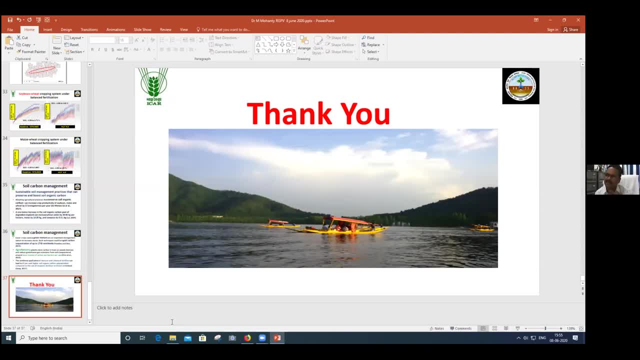 So this is what actually the concept is, But I presented 30 centimeters just according to my own convenience, I can say. but, just in time, my root zone is within 75 percent. you know, with that, And deserts, even deserts, can do this. Without trees, even deserts can act as a sink for CO2.. Soil is always there. Yeah, always there. That's good sir. But there are different process starts actually. So that different process will start because vegetation will be less. 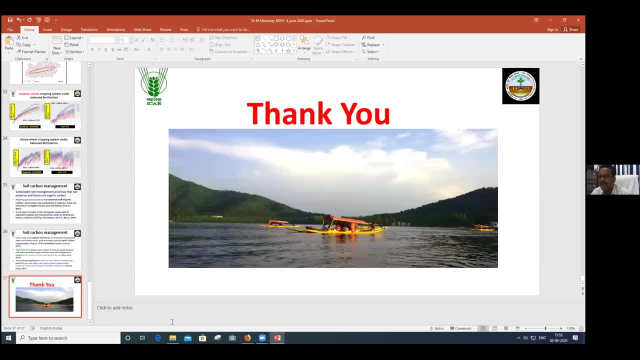 Don't know, bicarbonate carbonate. they are sort of just sink for carbon, carbon dioxide. Two different processes. This process will not act. That will be different process for them. Thank you, sir. My domain is actually chemistry, So it was very interesting sir. 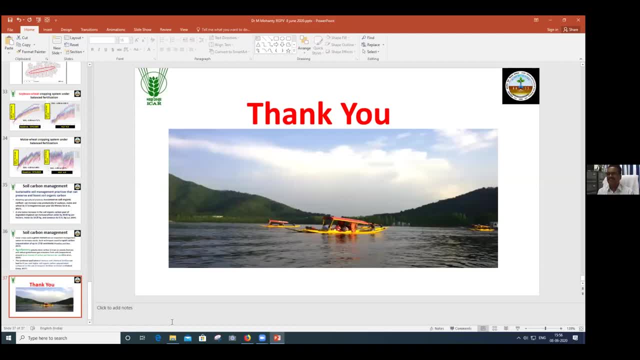 Very interesting topics, Thank you. Thank you, sir, Ma'am. your phone is muted, Sorry, sir. So one question. one more question from Mr Dushyant Tiwari. He's asking how the burning of crop residue affects the soil's organic carbon. 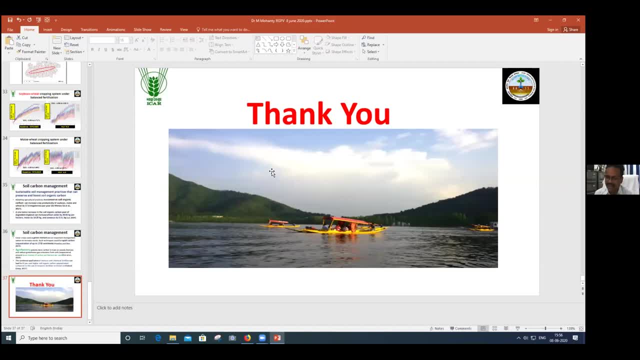 Quality Okay. So again, carbon quality Okay. definitely, when you burn, some amount should come to the atmosphere. Some carbon dioxide also lasts through burning, but still you can see those black. you know you can see those ash in the soil, but so far as quality is concerned, definitely that. 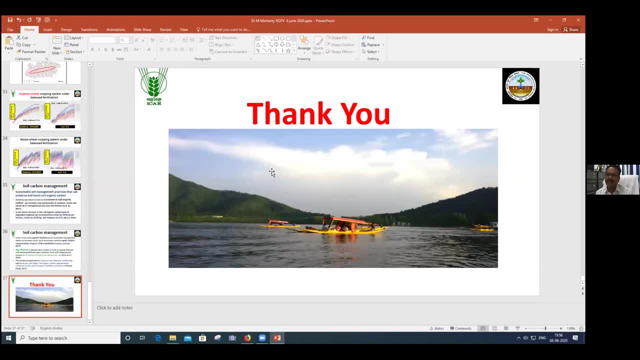 will be lost in the quality, because those black matters, you can say those ash, may not be eaten by the microbes very easily, you know, Because there's no nitrogen there, because it's just carbon, and the carbon may be inert sometimes, But we target also inert one. 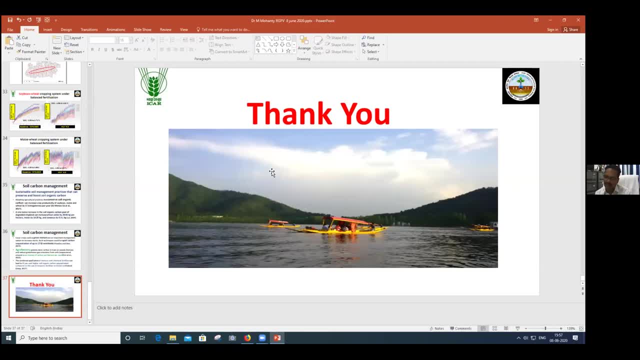 So when you talk about biochar, also through the process of burning, also that pyrolysis might have done in some parts of that, you know burning process, because it's not that only a hundred degrees Celsius or something will be there. That will be 200, 300 degrees in some zone, some zone of burning. 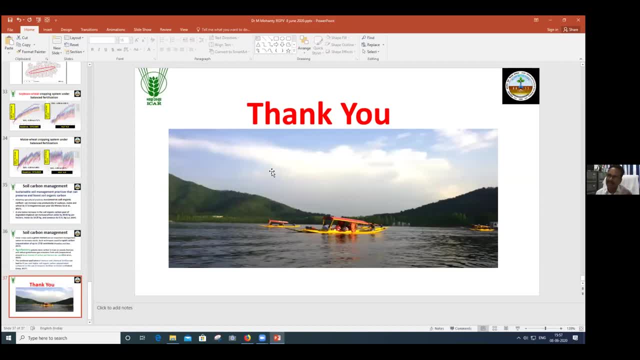 So in that case also you expect That some biochar might have formed which are more inert and resistant material. So that will also go to the soil organic carbon. But quality wise I can say, okay, that adds something to the inert part of the material. So that will improve. but we lost significant amount through burning That otherwise would have been added to the soil system. because of burning we lost significant amount. Only maybe 10%. 50% is added, 80, 90% is added. 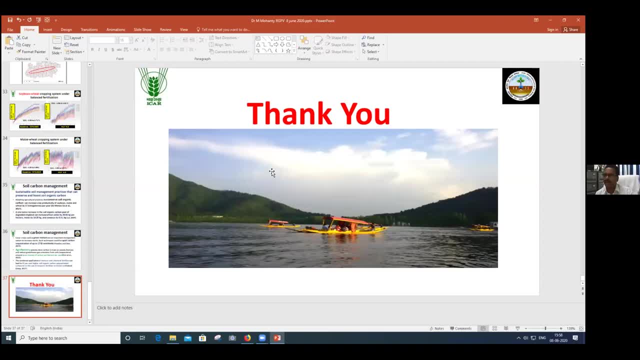 So 80, 90% may have lost as carbon dioxide, you know, suits metal, maybe some other forms. Thank you, sir. Most welcome, Dr Kapadia. your mic is on. Do you have some question? Dr Kapadia is there. 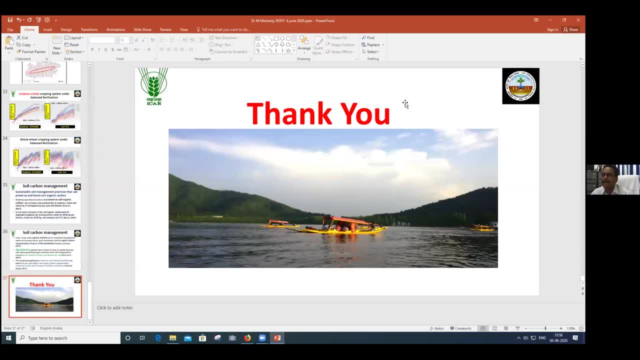 I think so, By mistake. she is on, Sir. one more question is that how to improve the soil bearing capacity by using soil carbon assessment? Okay, Because just like our soil health assessment, you might be knowing. government of India, MP government, everybody's talking about how to improve soil health. 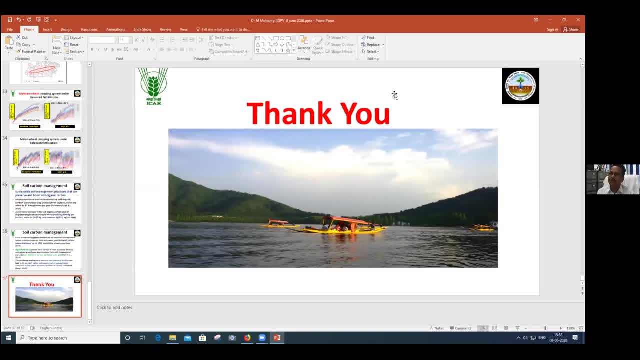 So definitely it is one indicator of soil health. So carbon content is more means you expect other nutrients, because presence of carbon- actually it influences soil health. So carbon content is more means you expect other nutrients. Actually it influences the nutrient cycling process in the soil. 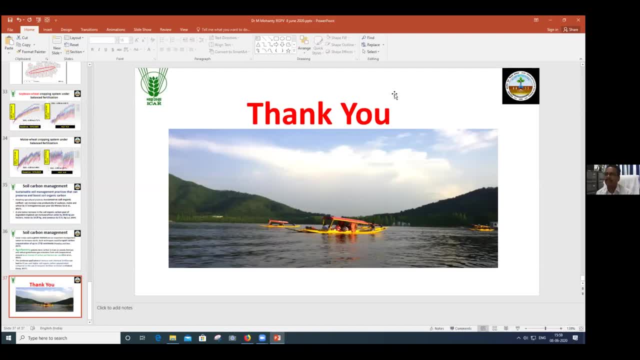 And the nutrient cycling process. when I talk about, I talk about the essential nutrients, not all the nutrient element that you study in your physics chemistry classes. No, It is the essential nutrients like nitrogen, phosphorus, potassium, calcium, magnesium. 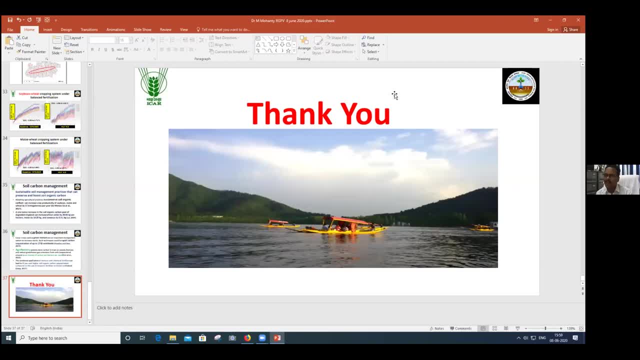 copper, iron, manganese, zinc, molybdenum, boron. These are all So actually this process, the presence of carbon that helps in improving the soil health. So this is a very important thing. I think it is important. 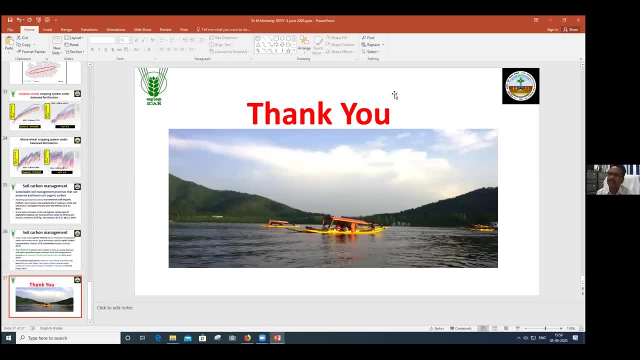 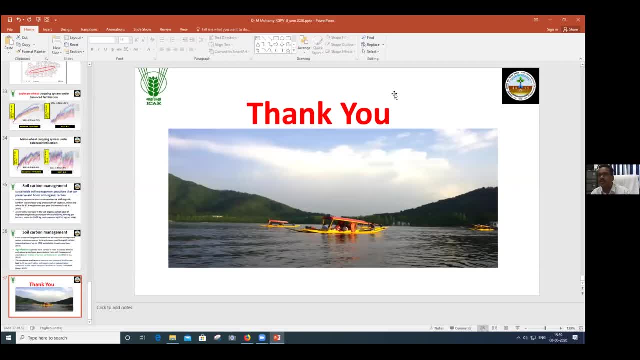 No, Any vessel of rebels is not presence in you know ability of those nutrients. So indirectly or directly, it is a whole healthy great info. So carbon is more means it's the nutrients have. better Recycle the cycle, sicklish process, winger and microbes are alive and you know the without. 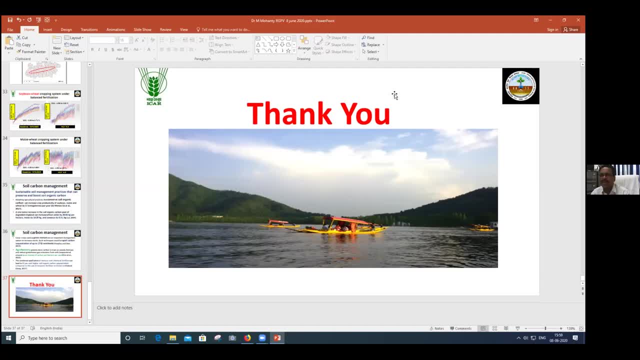 that restore, suppose, to the carbon sources for them. so my cause will not survive with the present. So you'll find that- and there is less time on- You'll get less number of bacteria. fun trayer- maybe beneficial, maybe not beneficial, but population will decline and soil biodiversity will be lost. so this is also one important that the 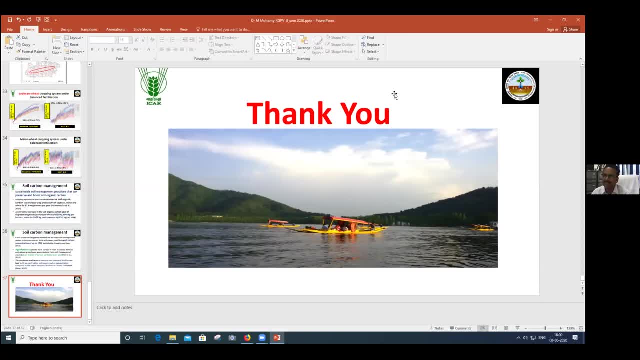 bias diverse is maintained with the presence of organic matter. so it makes all healthy. i think questions are known and there are no more questions. yes, please. i would like to convey here that, uh, engineering is called engineers or technologists. they can't be working the lab. all the engineering technology is for the application in the field of for the common people. 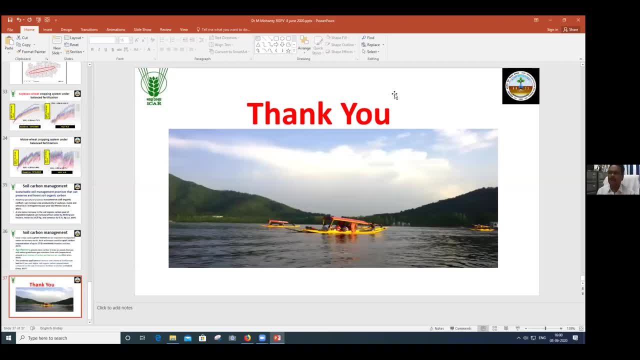 so we can't segregate that, we are not able. whatever i said is the integration of everything. your part is there because instrumentation part is yours. if i am a scientist, i work, i think it was definitely. i need something. you talk about iot, maybe you talk about ict you may talk about. 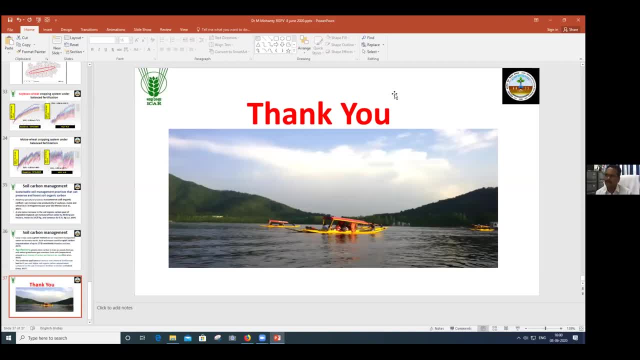 a drone application. i want to have a camera fitted to the drone uh on aerial unmanned vehicles. so i think your application is there. only thing is that we have to bring the problem to you, having some concept in our mind, and talk to you and see that i want to develop this type of of. 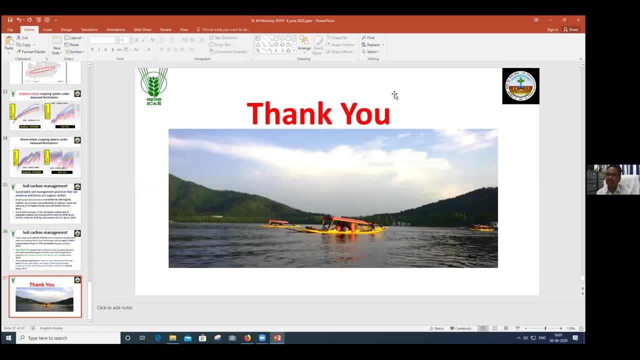 instruments, maybe a sensor, so you help us so and engineer, then that case engineer will go to the lab and develop that for us. so and we are apply most of the things we have been applied parts whatever i showed. this is but basic part is we are doing also some basic work, but this 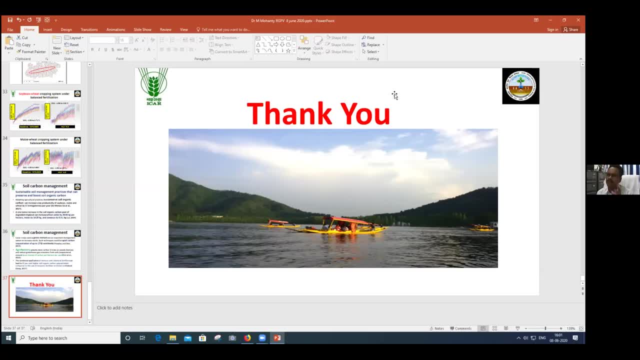 is the basic work. if i go to you and through some processes and with some concept in my mind to develop something, definitely i will bring engineers to lab developing a sensor for me, and we have a movie with gpb and we are expecting- uh, very soon- some 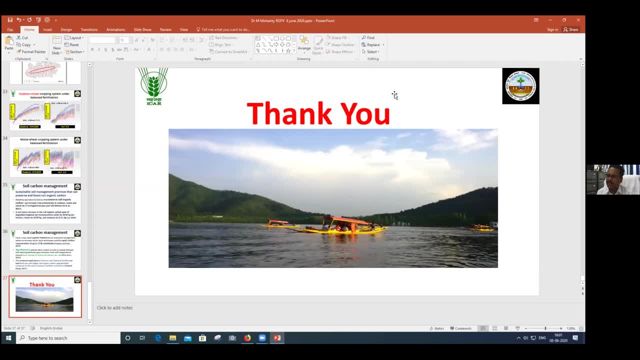 degree of, you know, uh, some involvement in our process. so it is already done. actually, we are waiting for the fund, i guess, and once it's done, definitely at gpb, and we will be working together for development of some sensors. so i would like to uh have a request that rgpv has. 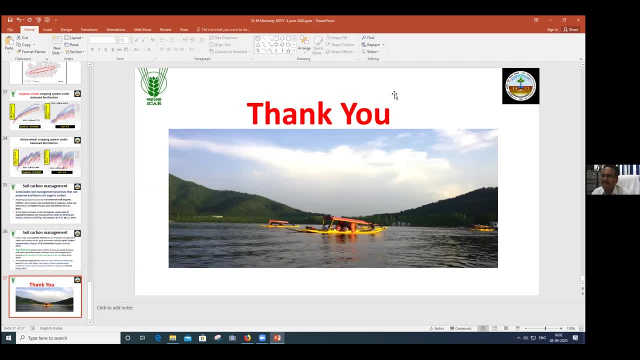 adopted five villages under unna tabian. very good, they are nearby villages. actually, hardly came to 15 kilometer distance, so definitely if soil sciences can help us, so farmers, so it is. we are having them for you also. yes, yes, so we can jointly work for the farmers here by improving. 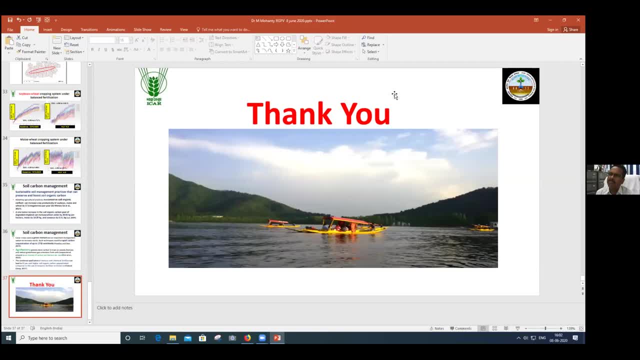 of course, because we are also having in our mirror. in that program we have adopted 55 villages. we also go there. now could be time so we have not visited. so we go there and listen to the farmers. we, we also work with them and we are also having- we are also having so many programs- farmers, scientists. 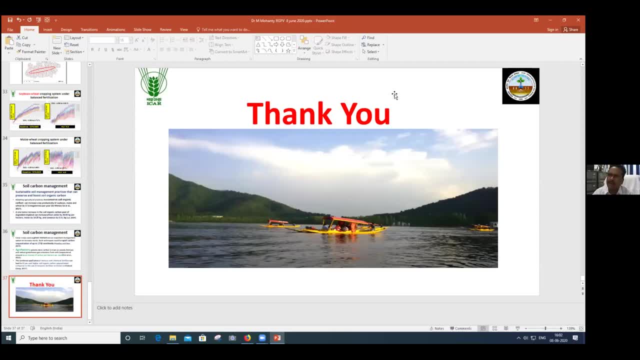 interaction and then some many forms of program, different types. so in that case also, if you want to bring, take us to your villages and if you can bring the problems to us to solve their problems, then definitely we are there to help, because we are there for this community only farming community. so those related to natural resource management. 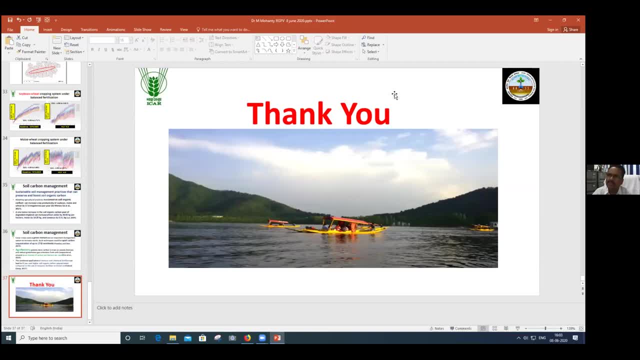 related to soil health management. definitely, our institute is more than capable of doing that, actually. so we are ready for that. not only me. we have teams, you know, team comprising of five scientists, uh, six scientists, having 10 teams. actually we have 60 scientists or 55 scientists. 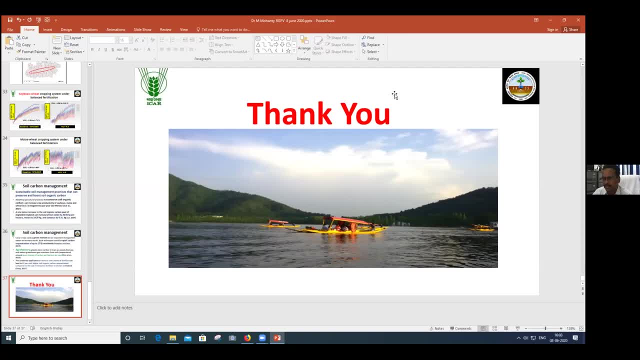 55 villages. so we are there actually, so definitely will help us, and without mo, you also, because this is our job, our duty. so our director, of which you don't deny this, and we are ready and we are always available, so we will help definitely, we will think. 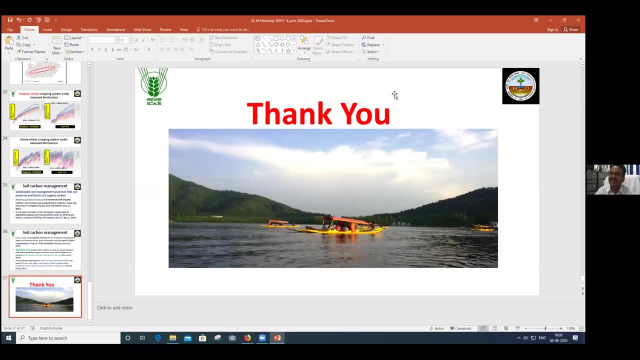 thank you so much because we will lake in this area to support the farmer. because i'm from energy environment department, we use to support only in the area of renewable energy. we installed solar power plants. We are working in the area of making these villages energy efficient. 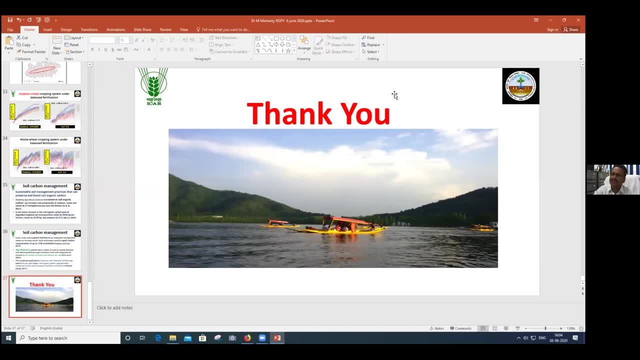 with the support of Urjavikas Nigam Limited, But definitely I want to involve your department and agricultural department so that we can support our adopted villages in a better way. Of course, Sure, sure, Why not? We are ready, Thank you. 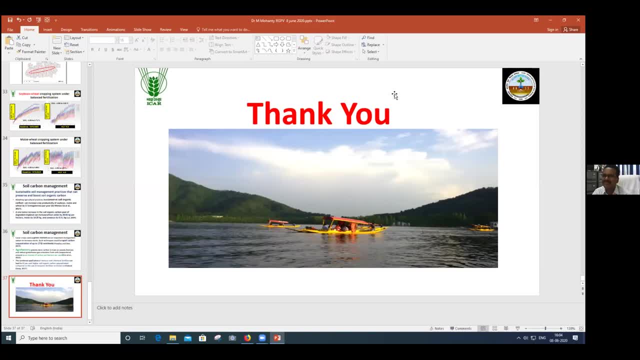 Thank you so much, sir, for a wonderful presentation. It's a very good presentation. It's definitely all the faculty of different disciplines got the new perspective on the new area of climate change. Thank you so much for giving us the time. So thank you very much for giving me the opportunity to talk to you and discuss the matter and 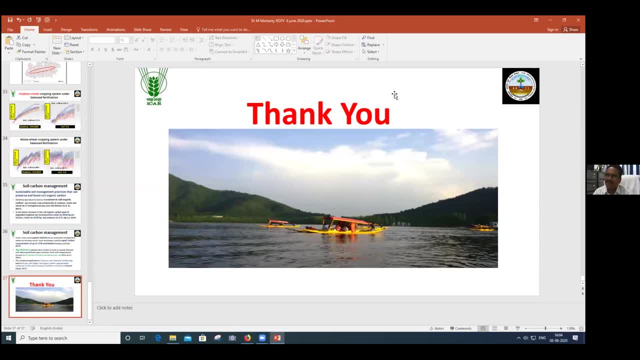 talking to the faculty members. I know this is a different topic, but I hope they must have got something they are not used to. So I'm really obliged and grateful to you inviting me for this. Thank you so much. Thank you, sir. 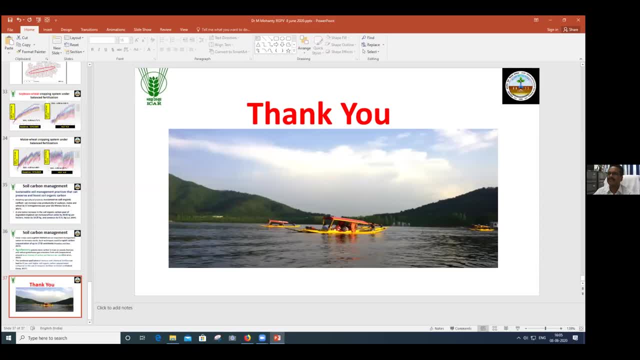 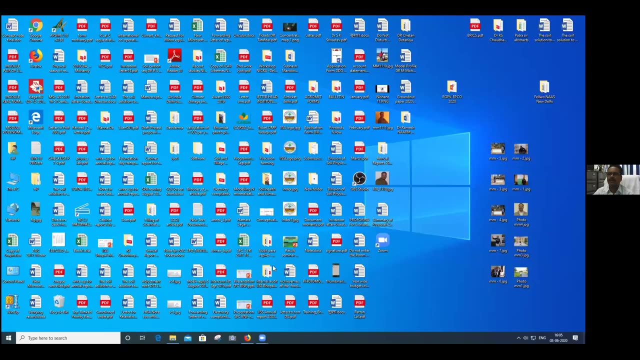 I would like to inform all participants. Now we are having the session, Tomorrow we are having the online examination, So we can take this time From last four to five days. you are listening to us only, So we would like to listen to all the participants. We would. 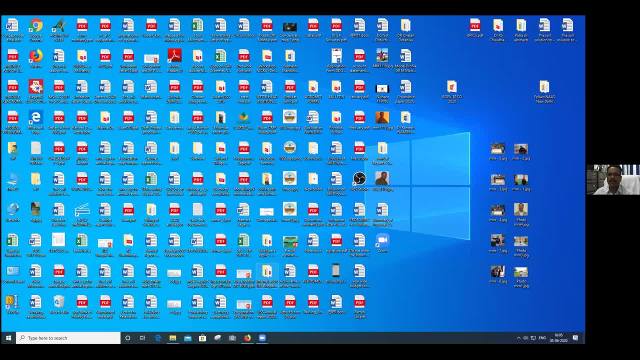 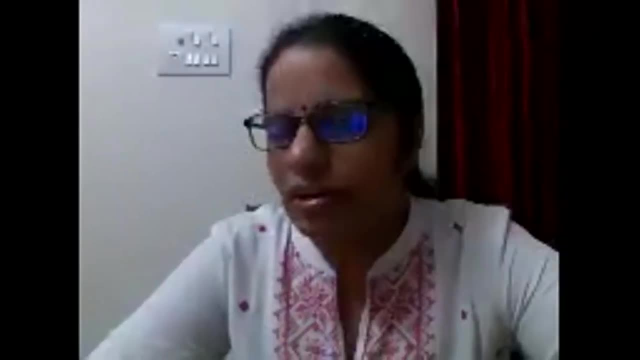 like to know their feedback. So you may raise your hand one by one. You can share your experience. We would like to listen to your inputs. So I would request all the participants to share your experience one by one, because we all belong to different. 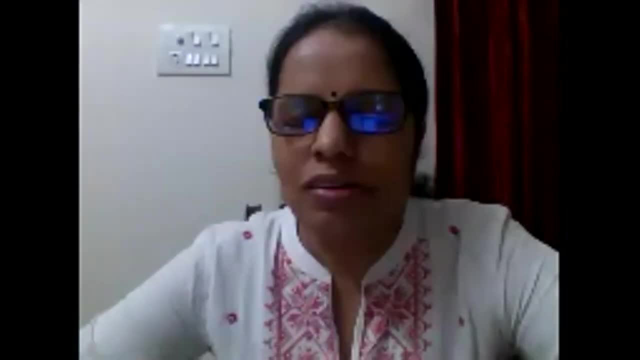 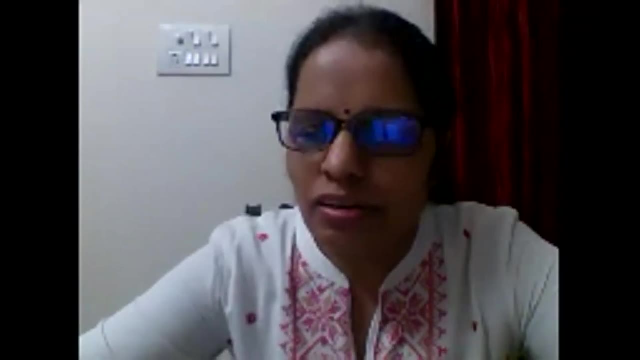 disciplines And this topic of climate change is definitely being planned to involve all the streams, especially the mechanical, civil, electrical, chemical, which are more close to this area of climate change. So it's my humble request, Thank you, Thank you. 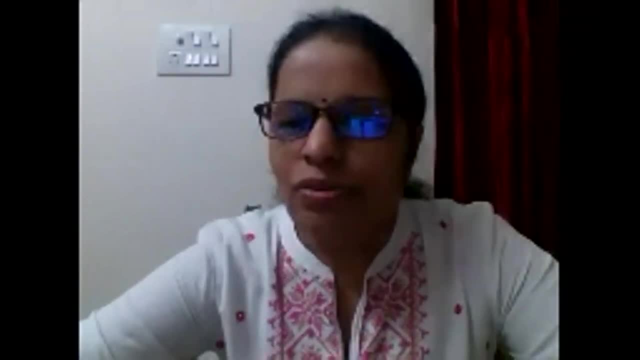 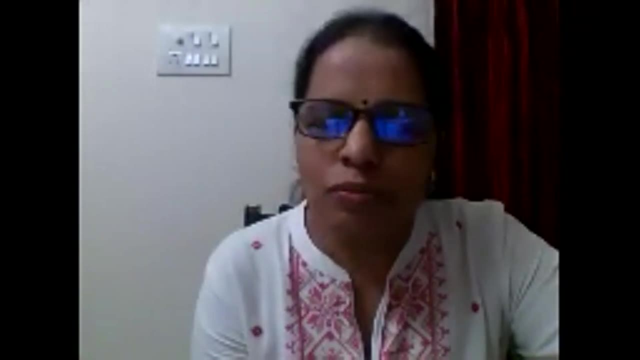 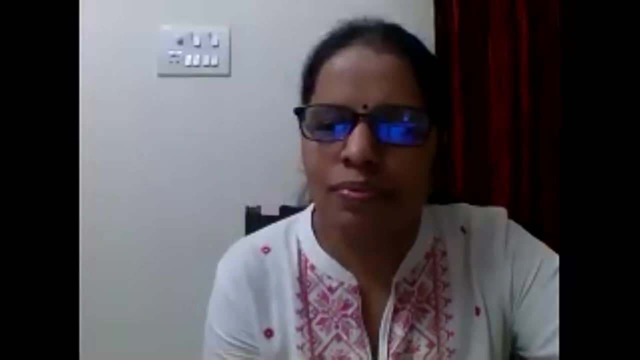 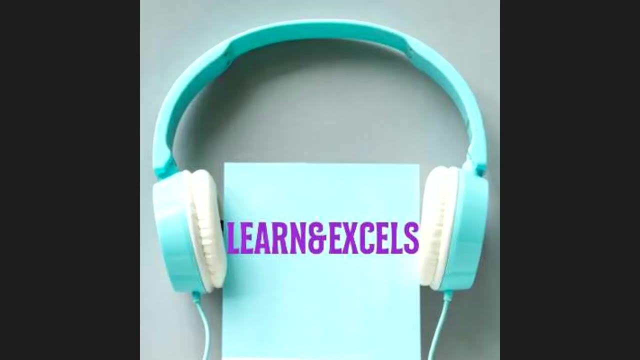 Hello, Good evening, ma'am Okay, angry. Hello, good evening ma'am Okay. I'm Dr from Arvinderaw College in worry, Okay, so what we will do I I'd love to talk to you. 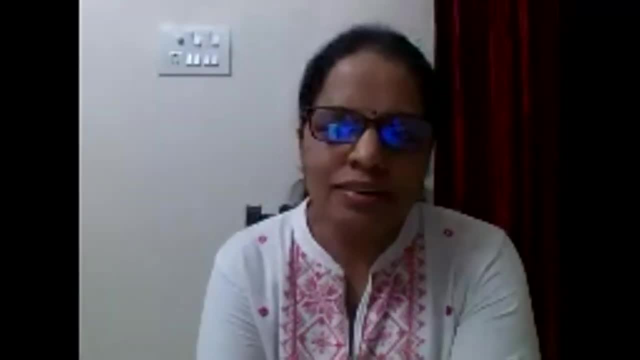 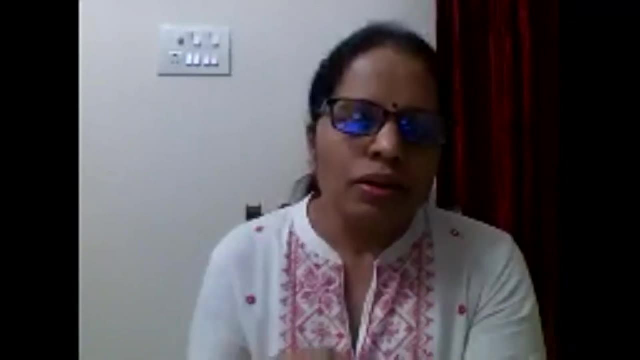 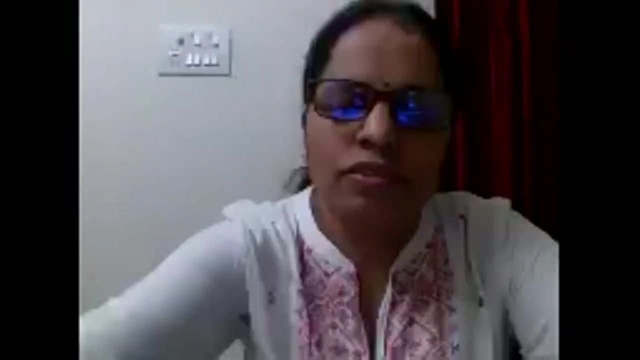 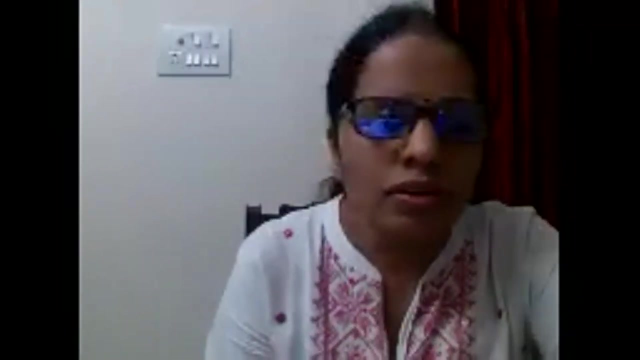 You, Are you able to see the table of Rune's hand? Are you all able to see? Okay, you can raise hand if possible, and we will unmute one so that it will be easy for us to listen to each and everyone. Anoop ji. 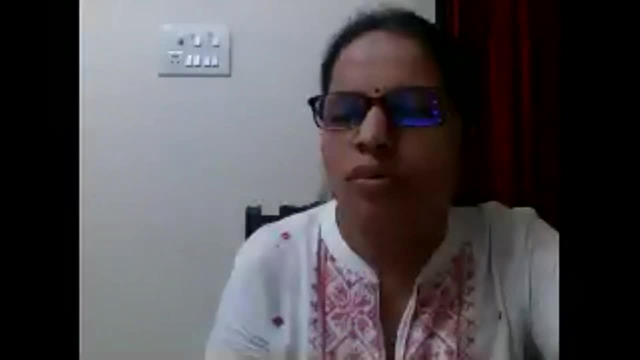 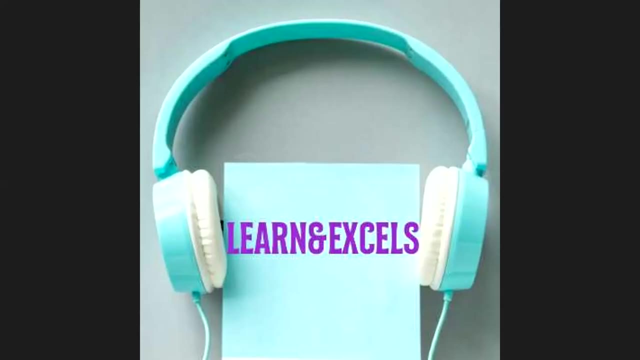 Jitesh Vijaya ji, Anoop ji, Anupam Mandluji. So, okay, we can. we will start with Anupam ji. Okay, good evening, ma'am, Good evening, so you can share about your institute. and about your discipline and 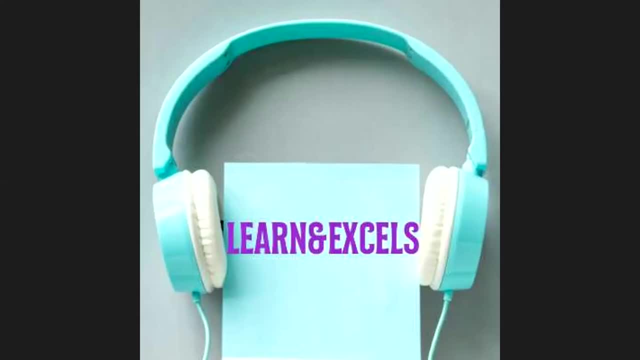 then about the program. okay, Okay, I am Dr Anupam Mandluji from Sri Aurobindo Institute of Technology, Indore. I am working there as associate professor in engineering chemistry department and we have projects related to environment chemistry with civil engineering. 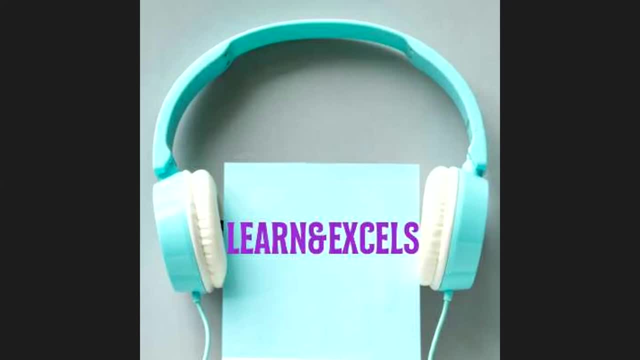 department also, that is, the effluent water treatment and all and I am taking subjects that is, chemistry, environment. so that is why I have joined this particular course, because it is more related to environment and analysis of water, that is, the input water- drinking water- and the output water. 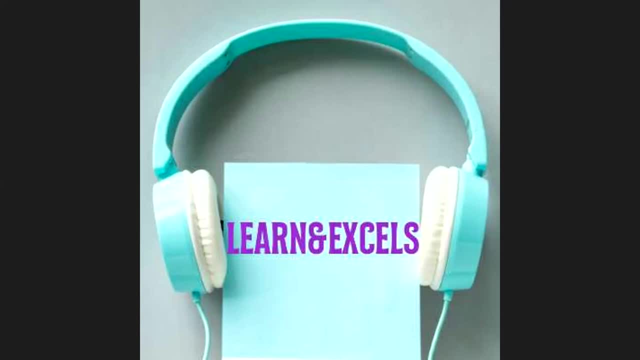 effluent water. so this particular training is very helpful for me, and we just have so many topics and ideas here so that we can use this as a project for a civil engineering student in their major project in the final year. This is my opinion, right, ma'am? 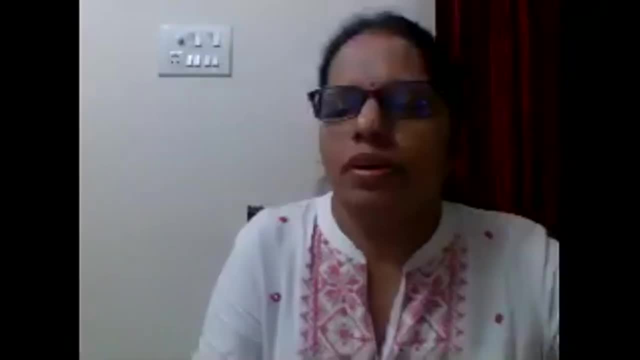 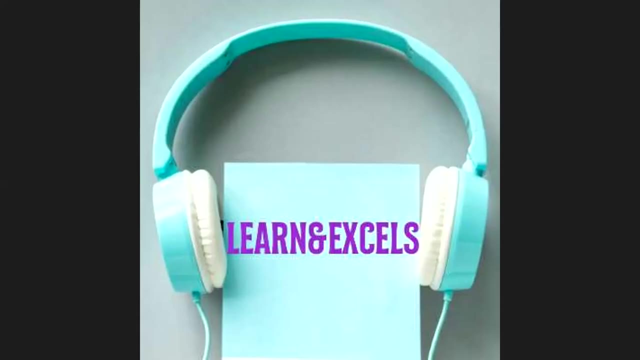 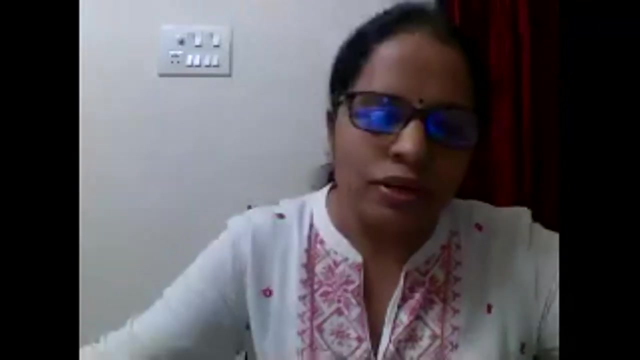 Thank you, Anupam ji. So next is Vijaya ji. so I would like to again repeat that we will share. you will share your name, institute, and then your discipline, and then how this climate change program has benefited you and will benefit you further in your work. 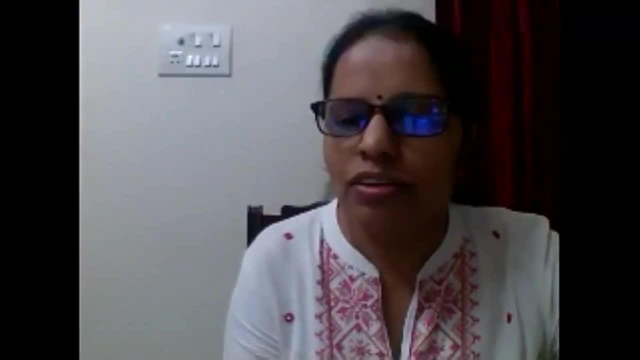 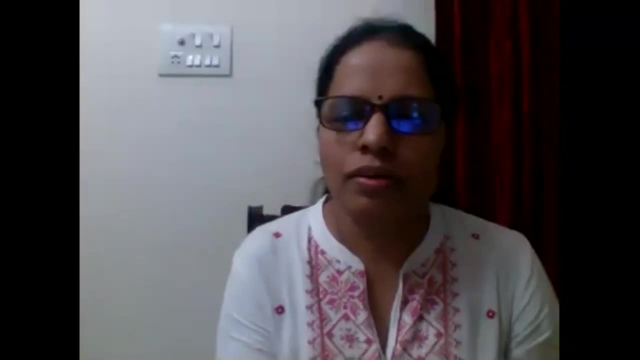 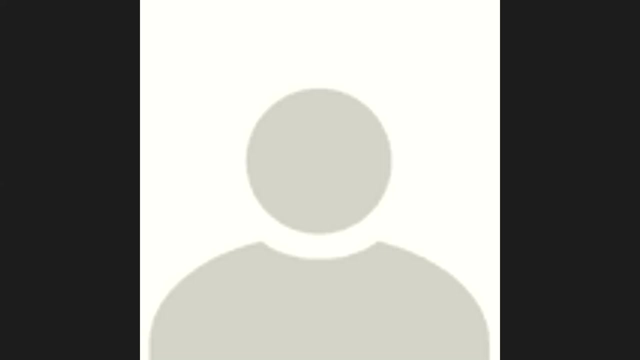 So Vijaya ji. okay, I have to unmute Chitesh. can you unmute Vijaya ji? Thank you, yeah, good evening, good evening everybody. This is Dr Menon from corporate group. I am from the department of chemistry and 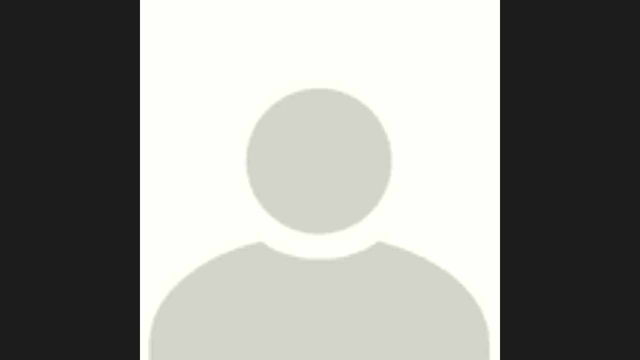 I think from the past 10 years I have been very closely related to climate change because I have quite an interaction with Mr Lokhande Thakkar, because he stays quite close to me, So we actually discuss a lot about these things and basically because of my, because I am-